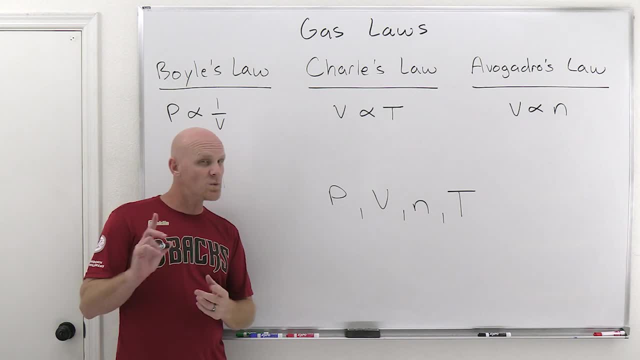 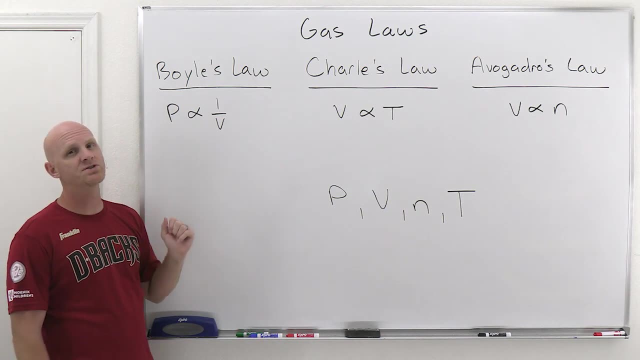 So that's kind of implied in there. so just keep that in mind. That'll be important in one key place I'll bring up All right, so we'll start with Mr Boyle here. And Mr Boyle here said that pressure is inversely proportional to volume. 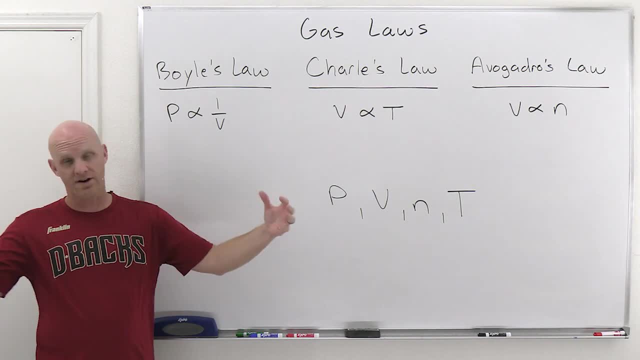 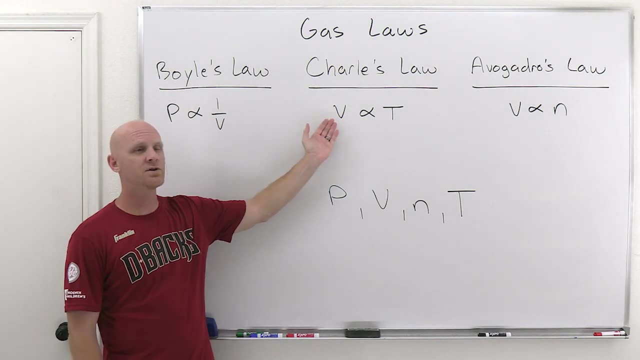 So he says, as your volume goes up, your pressure goes down. or as your volume goes down and gets smaller on the gas, then your pressure goes up. So there's an inverse relationship there, whereas Charles here compared volume to temperature and he said they're directly proportional. 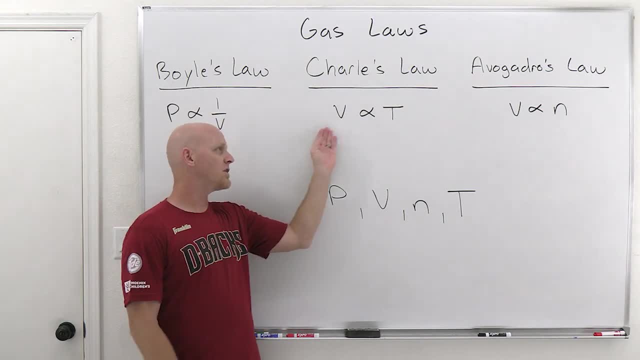 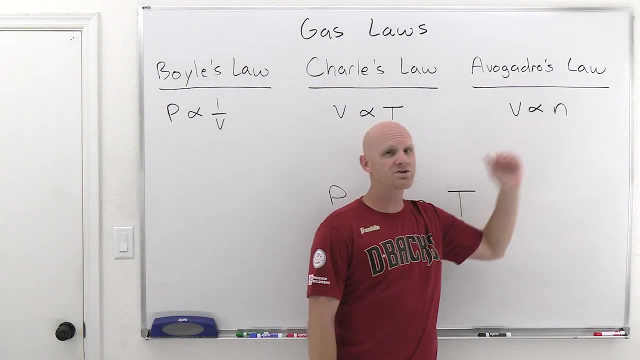 Again, assuming we hold the other variables constant, then volume and temperature are proportional. As temperature goes up, volume goes up. And then, finally, Mr Avogadro said volume is proportional to the number of moles of gas. As you add more moles of gas, the volume of that gas is going to increase. 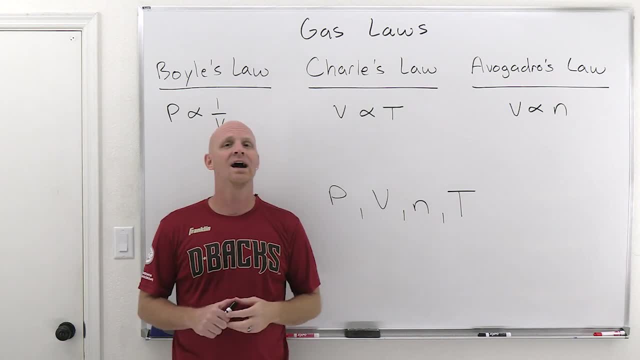 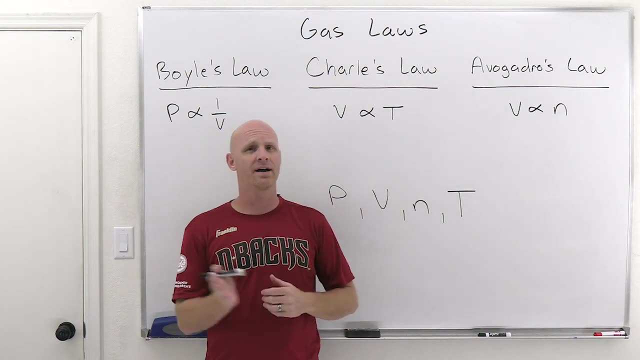 again, assuming the other two variables are proportional, The other two variables are held constant. Now I like to kind of envision Mr Boyle over here and Mr Avogadro over here at a little kid's birthday party way back in the 1700s or 1800s. 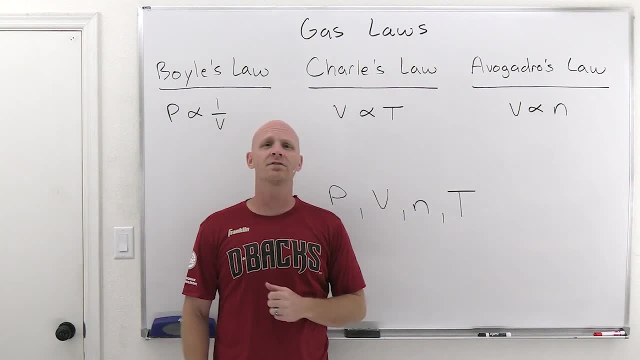 While at this little kid's birthday party, Mr Avogadro finds a balloon lying on the ground that has not been inflated and he picks it up and he blows it up And he's like Eureka. My name is Amadeo Avogadro. 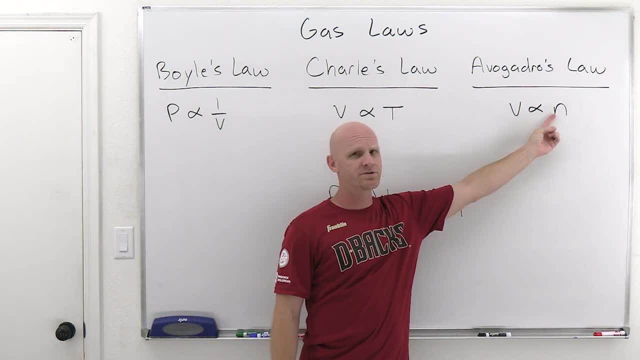 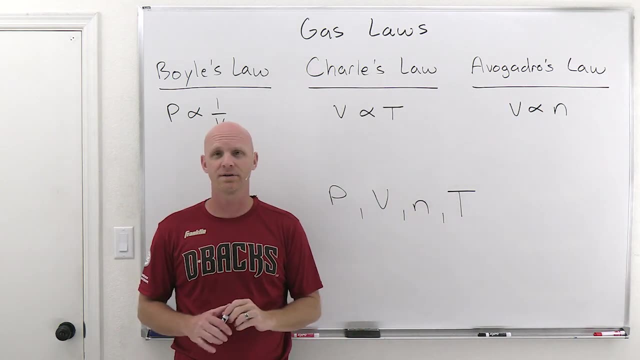 And I have just discovered that as I put more moles of gas in the balloon, it gets bigger, It has more volume. Way to go, Sherlock. So. but that's exactly kind of what Mr Avogadro discovered. So, and truth be told, he said you know, what he really said is that 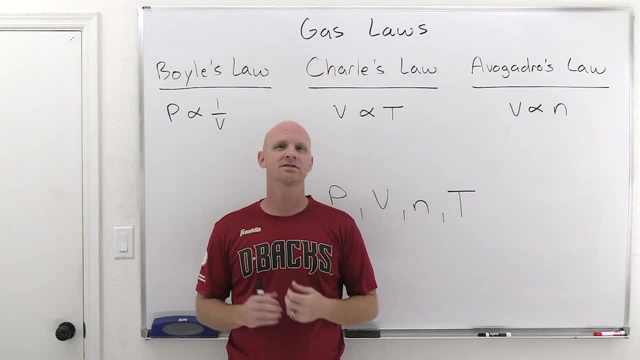 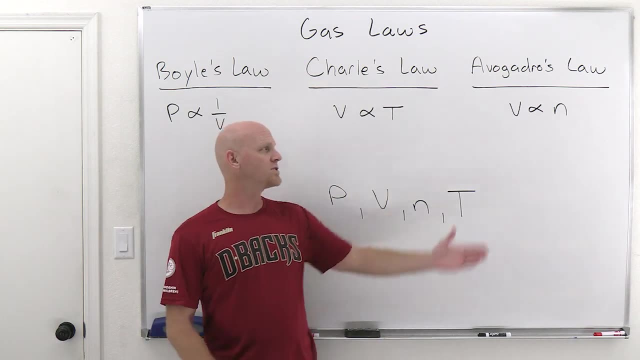 you know, if you have two gases under exactly the same conditions of pressure and temperature, then equal volumes will have an equal number of particles. That's what he really said. Well, what we translate that into is they'll have equal number of moles. 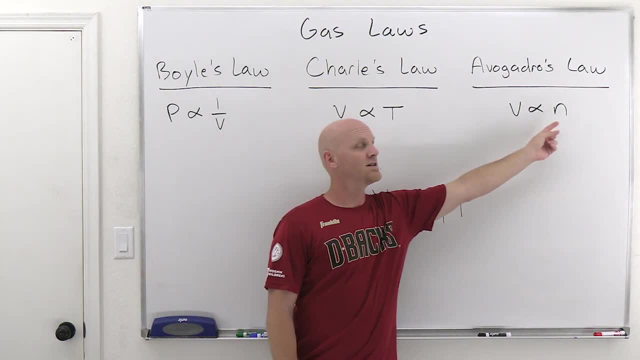 and that really under the identical conditions of pressure and temperature, that your volume is really proportional, therefore, to the number of moles of gas in that sample. So we're kind of extrapolating it out a little bit from what he said. 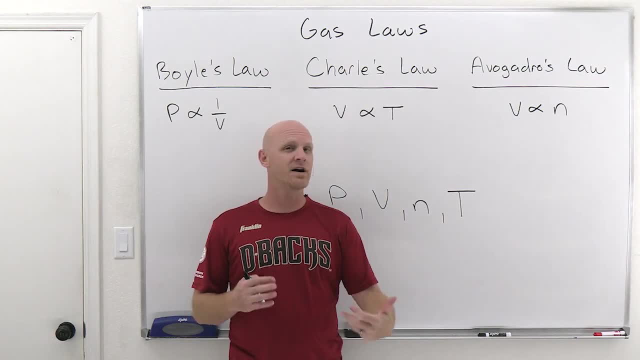 but I like to really simplify it, But really he really did make a profound discovery. I just kind of like to make light of what he actually discovered. Well, Mr Boyle- not to be undone- is at the same party, and so he picks up a balloon off the ground that's not been inflated. 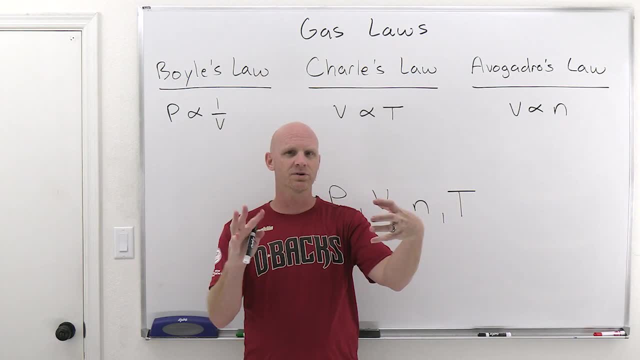 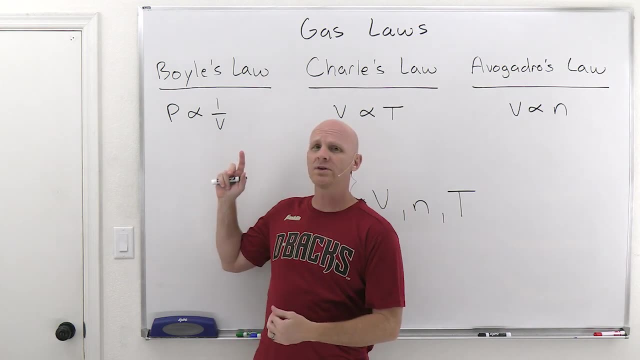 and he blows it up and ties it off, and then he starts squeezing on the balloon and squeezing on the balloon, and then it pops And he's like Eureka, I'm a genius too. So, as I made the balloon smaller and smaller and smaller, 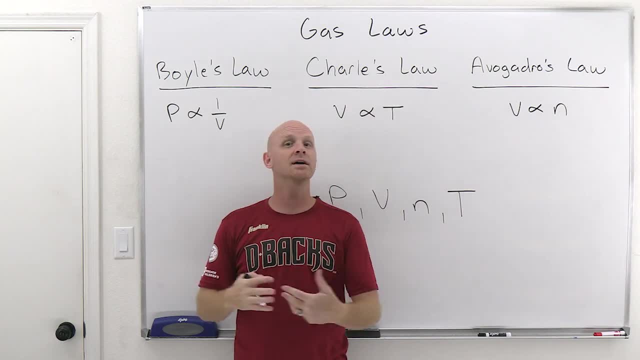 the volume got smaller, the pressure went up high enough to make it pop, And so pressure and volume are inversely proportional. Put my name on it, So we have another Sherlock here. It used to be a lot easier to get your name on something here. 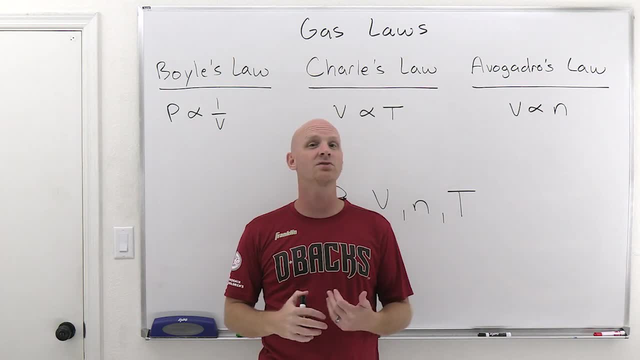 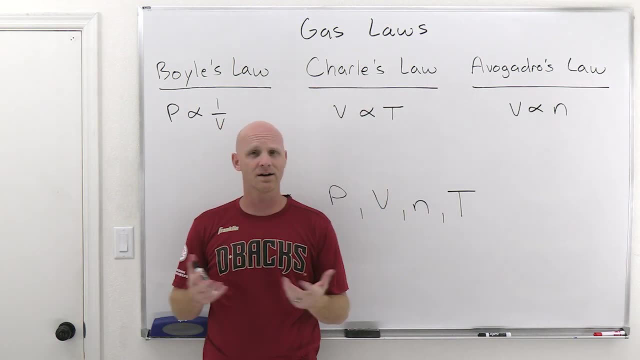 So, but that was Boyle's conclusion here, that pressure and volume are inversely proportional. And Mr Charles is the only one I'm really going to give credit to. I don't think he was really at this birthday party that I'm making up. anyways, that didn't exist. 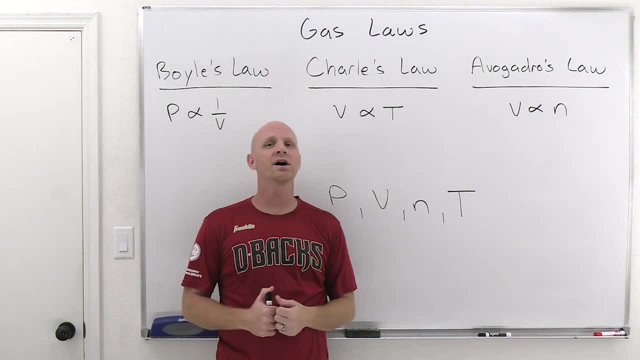 So this fictitious birthday party. But he said volume and temperature are directly proportional. Now I live in Arizona And if you go out on a hot day in August from your air-conditioned house there is a huge temperature increase, Say from, like you know, 75 degrees in your house. 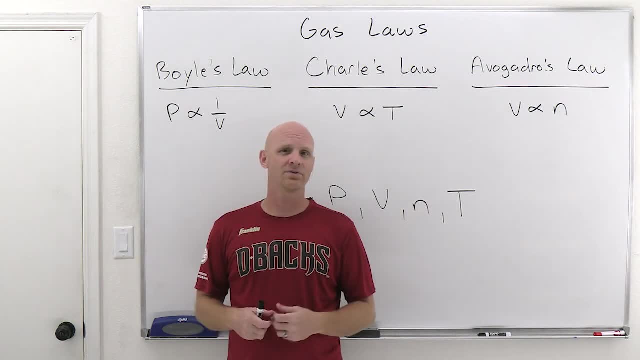 to like 110 or 115 degrees outside your house And if you take a balloon that's just filled with air- not a helium balloon or anything like that, although you can do it with that too- but just a regular air-filled balloon- 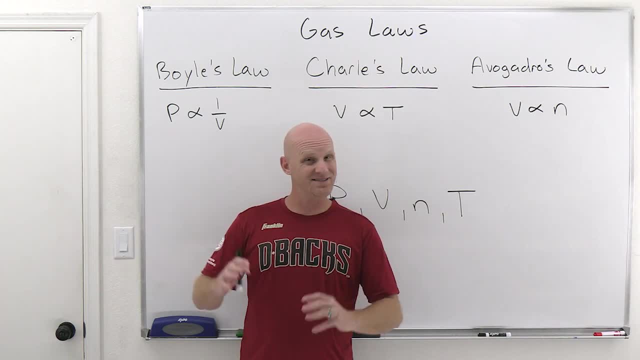 and you know, rather full tied off and you take it from inside at 75 degrees to outside at like 110 degrees, you will actually notice actually expand. So as the temperature of the molecules goes up, the volume goes up as well. 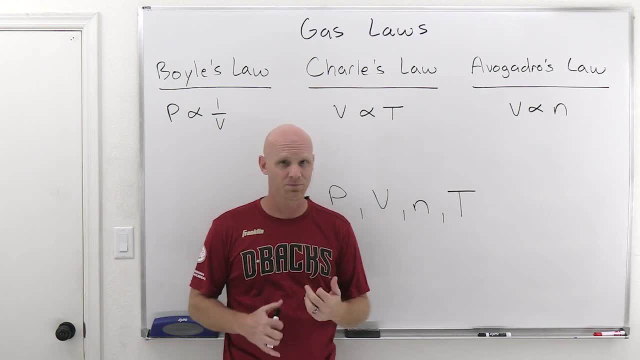 And so it's actually noticeable enough with that big of a temperature difference to see that difference. And you can also see this kind of you know in a hot air balloon. I like to envision Mr Charles kind of you know riding in a hot air balloon. 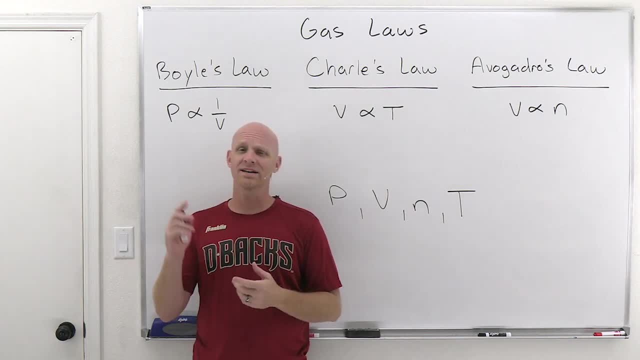 And again, that's completely fictitious, But I like to envision that- And he's riding in this hot air balloon And he sees some power lines up ahead which also didn't exist when he was alive. But hey, it's all fictitious anyway. 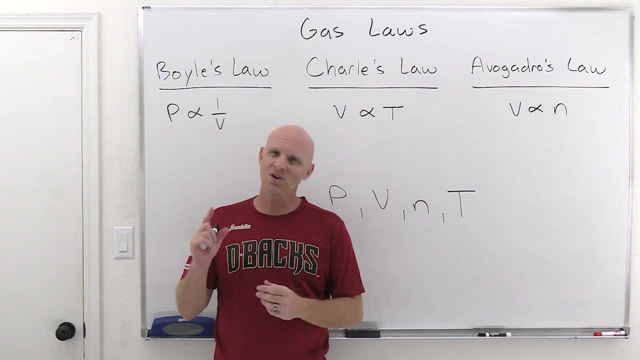 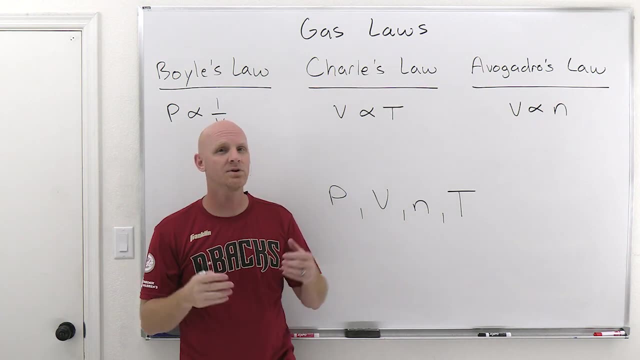 So he sees these power lines And so what should he do? And don't think jump, That's not his option here. So what he's going to do is pull the jet and heat up the gas inside the balloon And that's going to cause that gas inside the balloon to expand. 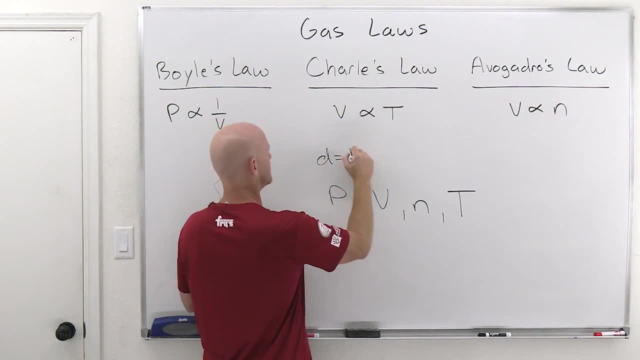 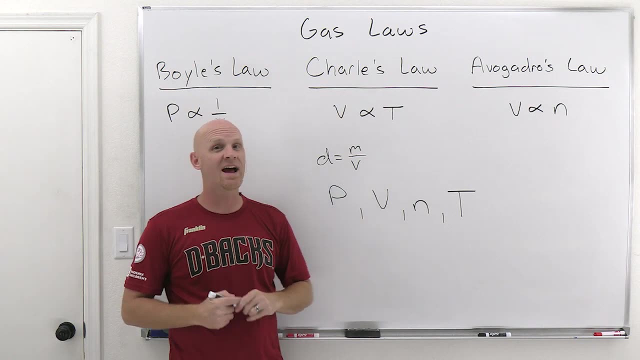 And as it expands, keep in mind that density equals mass over volume. As that volume inside the balloon expands, the density of that gas in the balloon goes down And all of a sudden the gas inside the balloon is less dense than the gas the air around it. 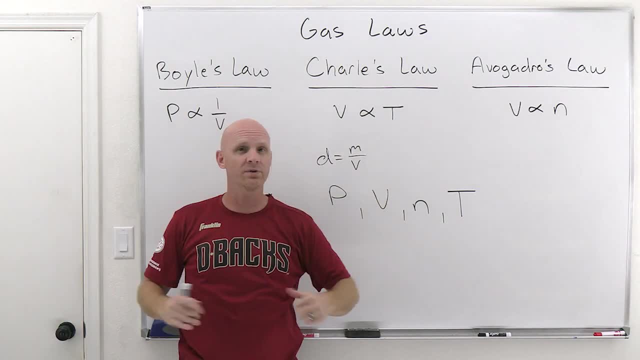 And when you've got you know something that's less dense than the fluid around it, it's going to rise, Like putting you know a ping pong ball, you know, and carrying it to the bottom of your pool. So if you let it go, it's going to rise to the surface. 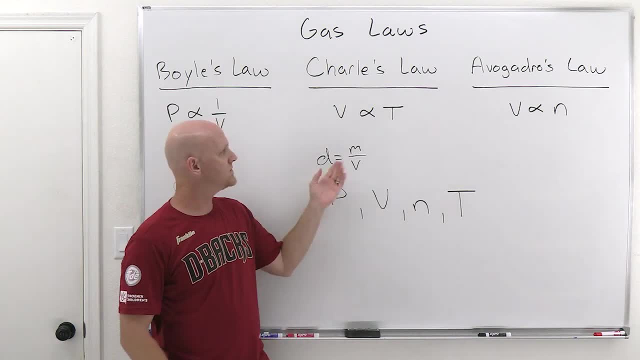 because it's less dense than the water around it. Well, same thing: when you heat up the air inside that balloon, It's going to be less dense. That air inside the balloon is less dense than the air around it, And so it's going to want to rise. 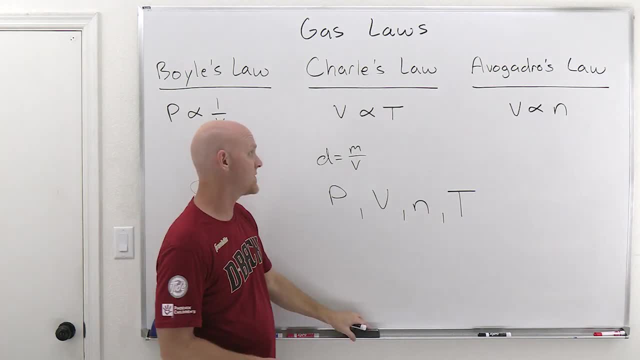 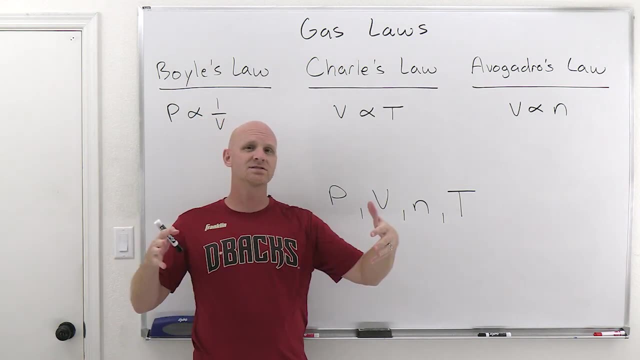 There's a buoyant force acting on it. It's really what's happening there, And so that's what I like to think of Mr Charles, figuring out that you know temperature and volume are directly proportional. As you heat up a gas, it will expand again. 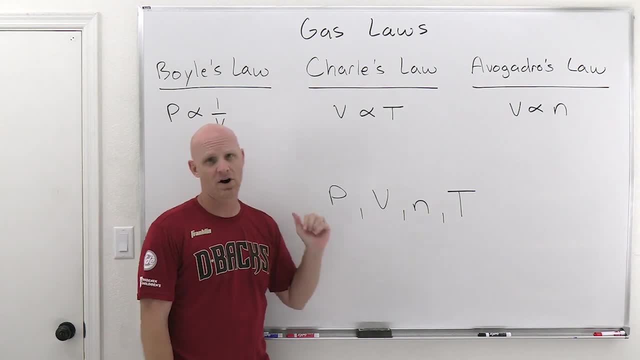 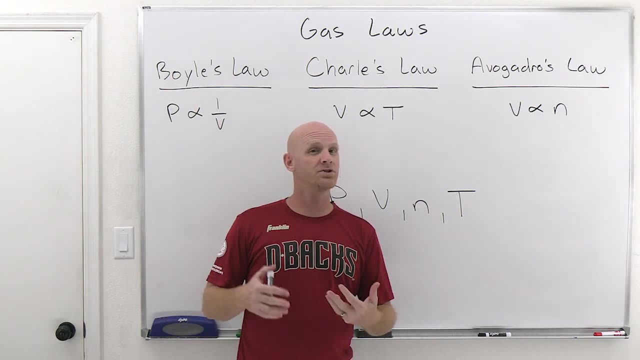 assuming you're keeping P and N constant. So there's our three gas laws there. You should know what they're comparing volume to and you should know if they're directly proportional or inversely proportional. And again, it's pressure that's inversely proportional to volume. 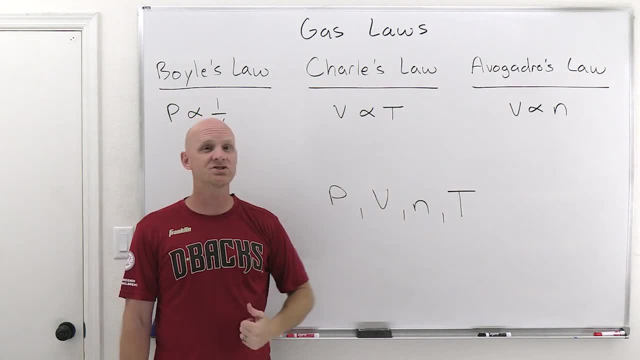 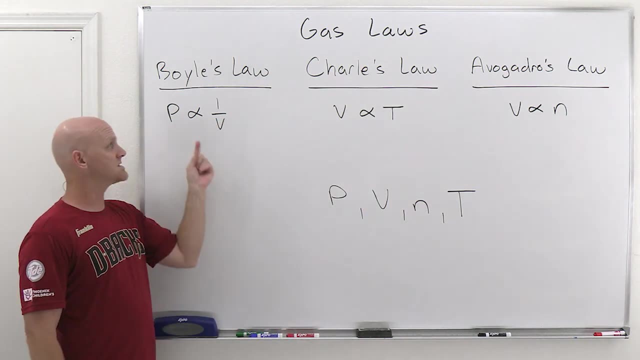 but both temperature and moles of gas. there's a direct proportional relationship. But again, keep in mind, all three of these are dependent upon the other two variables being held constant. So if I said, does Boyle's Law say that? as you know, 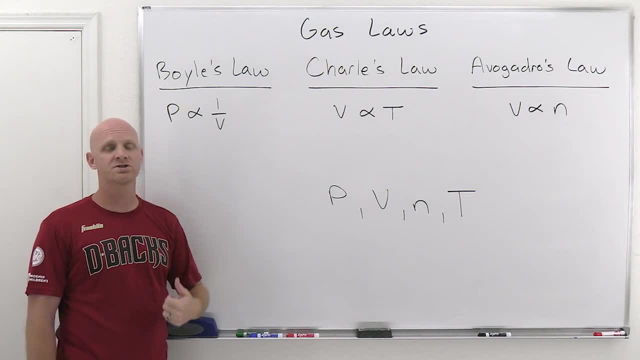 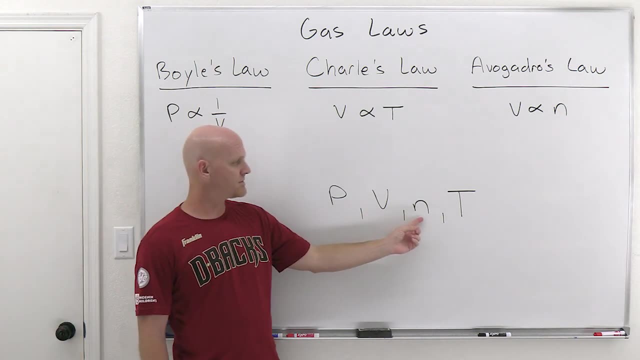 volume goes up, pressure goes up, pressure goes down. or as volume goes down, pressure goes up. is that true always? Well, that's true if you're holding the number of moles of gas and temperature constant. So if I make the volume smaller, 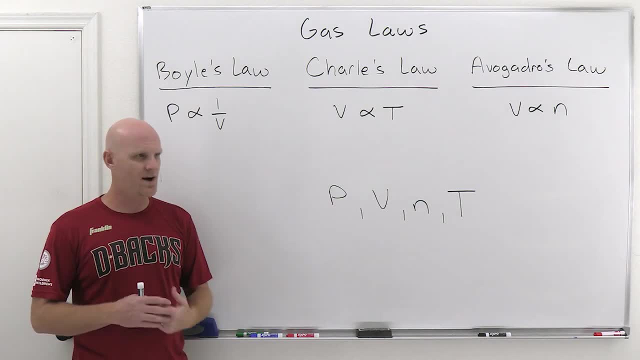 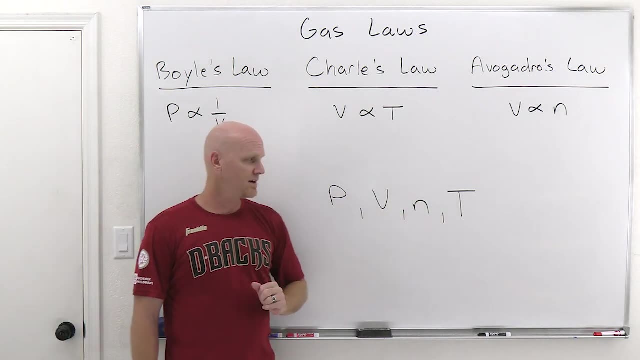 does that mean the pressure has to go up in all situations, for everything? Well, no, But it would mean that it has to go up if the number of moles of gas and temperature are being held constant. Now, one thing you should know: 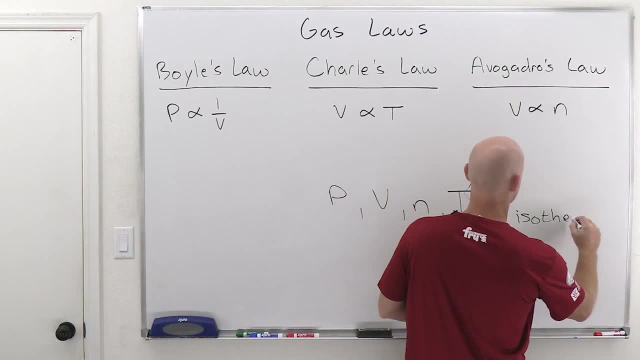 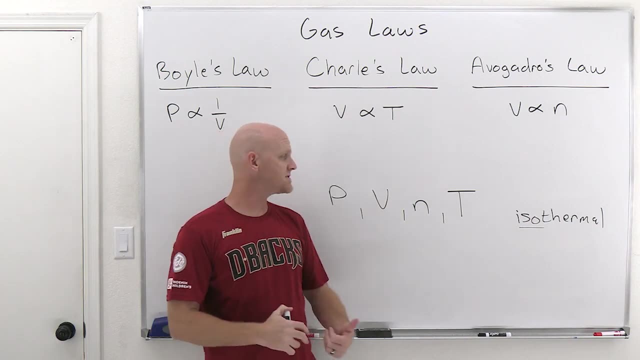 and I'll just throw this vocabulary in there. some of you guys are going to get this one is that isothermal is a word we use. Iso means the same and isothermal just means the same temperature, so constant temperature. So we might say that you know. 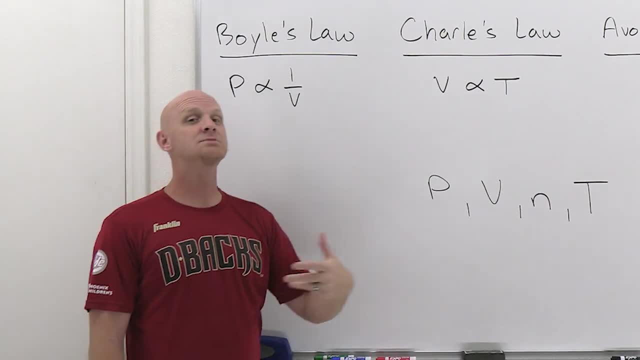 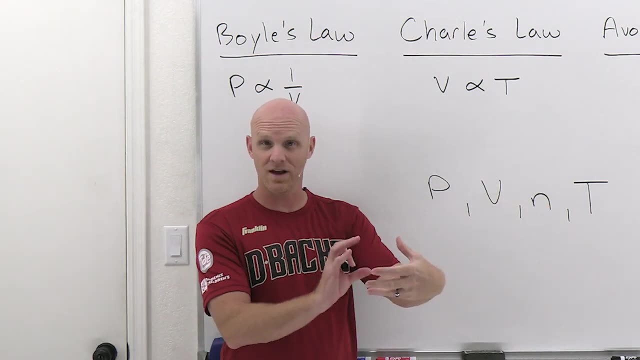 if we carry out a process isothermally for a specific sample of gas, well, if it's a specific sample of gas, well then we're not adding more gas to it or removing gas to it, It's just for that set sample of gas. 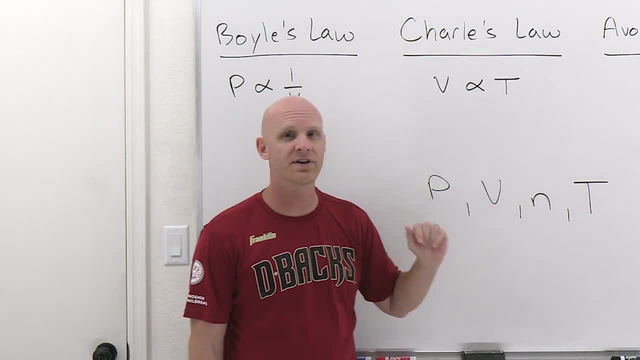 So if I'm doing a process isothermally for a specific sample of gas, that would be one way of indicating to you that, yeah, it's at constant n and constant 2.. It's at constant n and constant t And under those conditions. 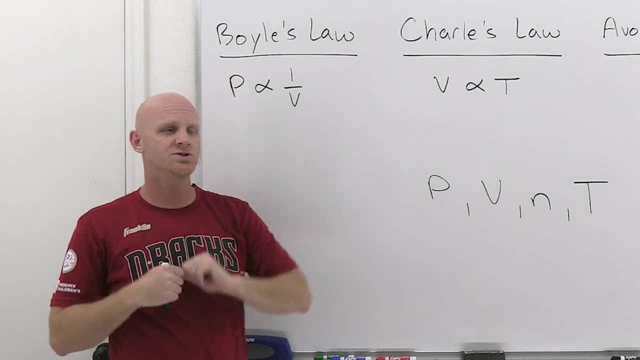 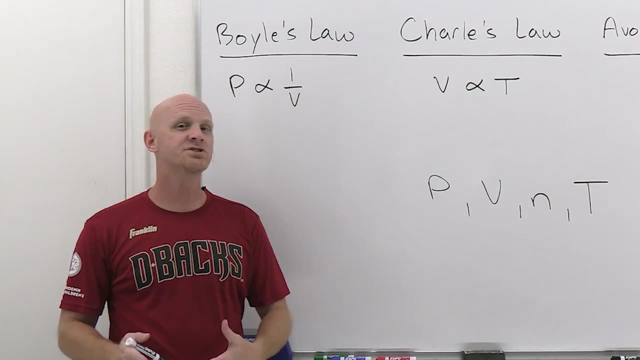 that's when pressure and volume are inversely proportional. So, and again, it's not just an inverse relationship, but inversely proportional. So if I double the volume, the pressure's cut in half. If I triple the volume, the pressure's going to be a third of its original value. 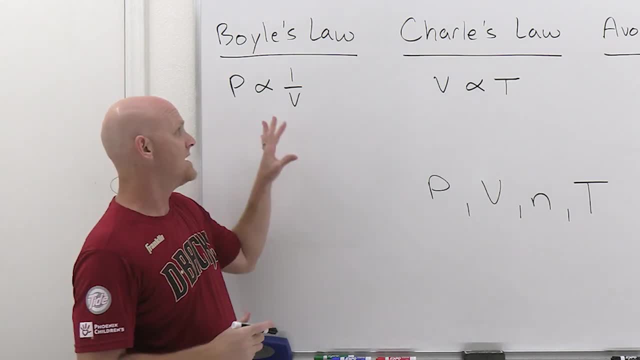 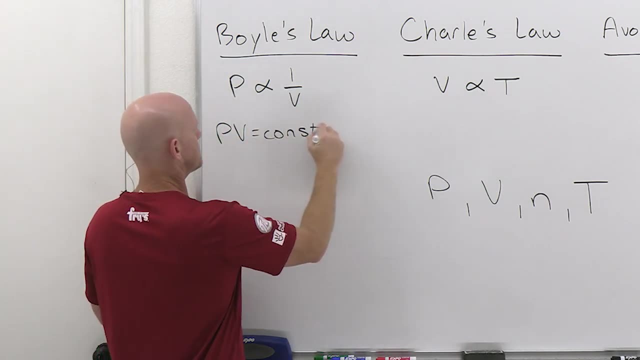 There's that inversely proportional relationship. Now there's a couple other ways you can actually, you know, explain this. You could say that p times v equals a constant. So this way you know if p times v equals a constant. 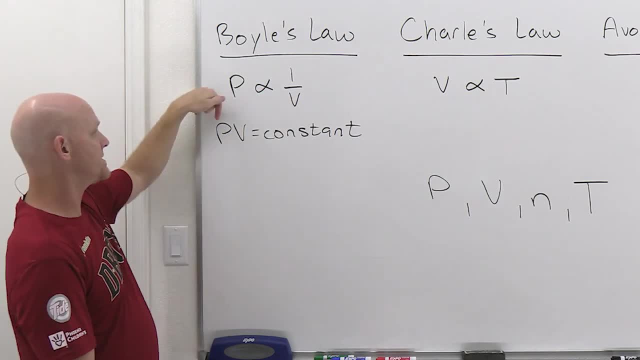 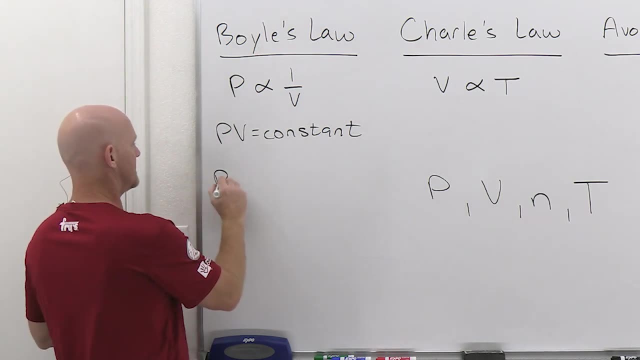 well then, if your volume goes up by a factor of 2,, well then your pressure would have to go down by a factor of 2 to multiply, to equal that same constant. You could also say: p1v1 equals p2v2,. 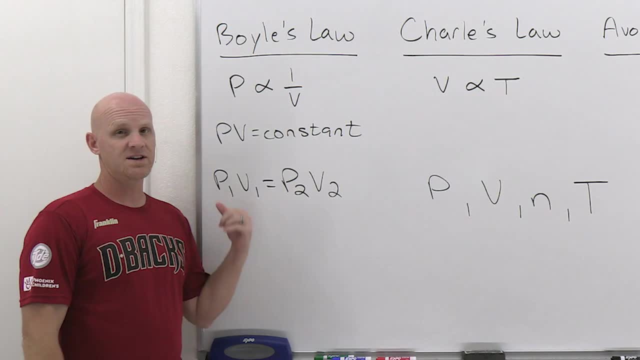 another way to express it, And so you're just, if you're you know, say changing and altering the conditions of a gas from one set of conditions to a second set of conditions. So I got four variables here, If all I'm changing is pressure and volume. 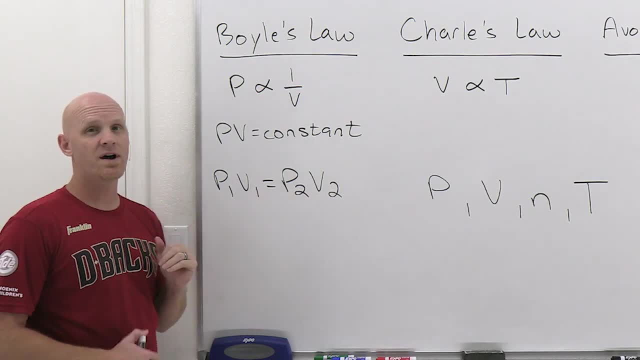 not again moles of gas and temperature. there's your Boyle's Law, another way to express it, And if I give you, you know, say the initial pressure, initial volume and final pressure, I could say what's the final volume? 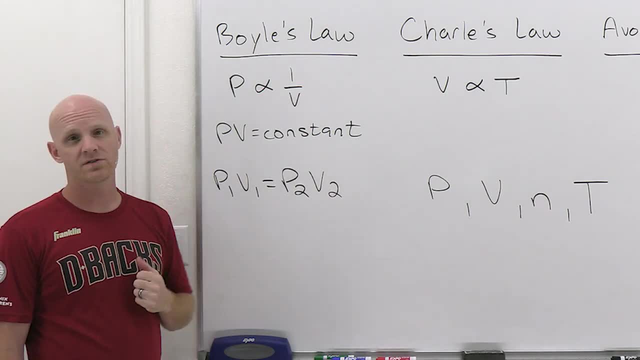 So essentially I could give you any three of these four variables and say what's the fourth one. So you know, if I start off with, say, a pressure of one atmosphere and a volume of one liter, and let's say I change that pressure, 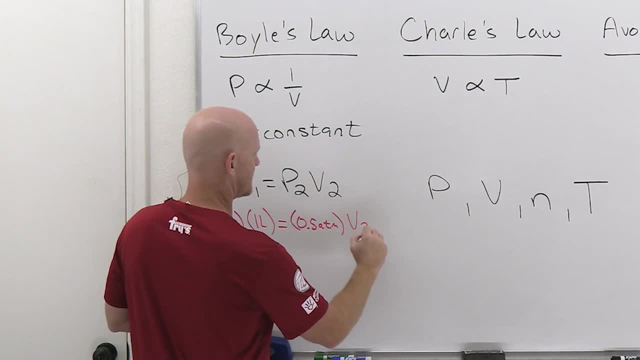 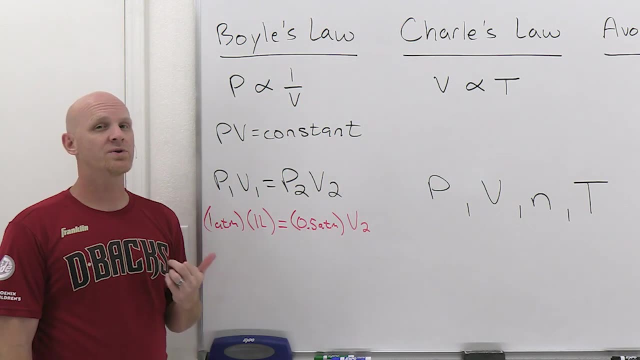 to 0.5 atmospheres. well, the question might be: what's that final volume? Well, in this case, I've taken that pressure and cut it in half. And if you cut the pressure in half, the volume needs to double. 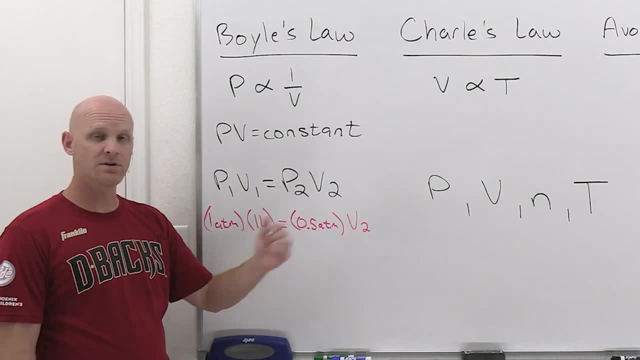 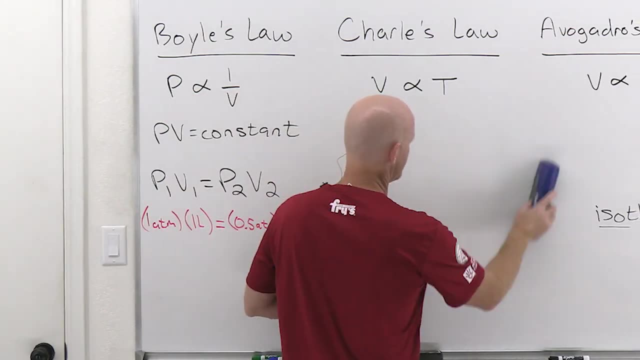 and we would anticipate that it would be two liters. And if, lo and behold, you solve for V2 there, you will indeed get two liters, Okay. so let's go on to Charles' Law here, And Charles again compared volume to temperature. 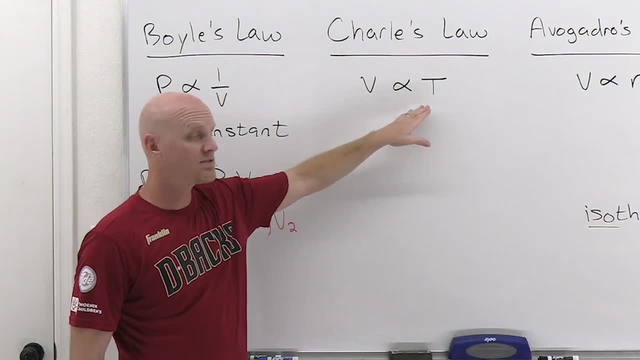 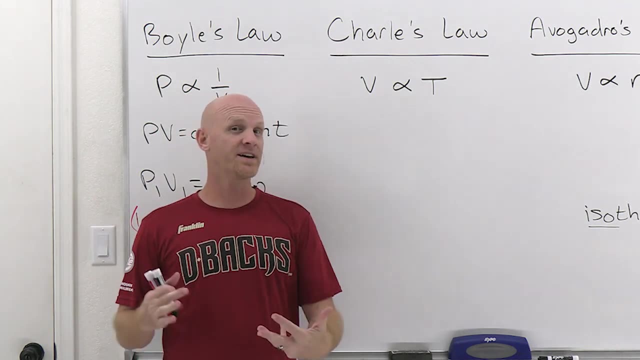 and they're directly proportional. Now, one thing that's super-duper important here is that whenever you deal with temperature in this chamber, it is going to be on the absolute scale, on the Kelvin scale, not Celsius. So, if you notice, 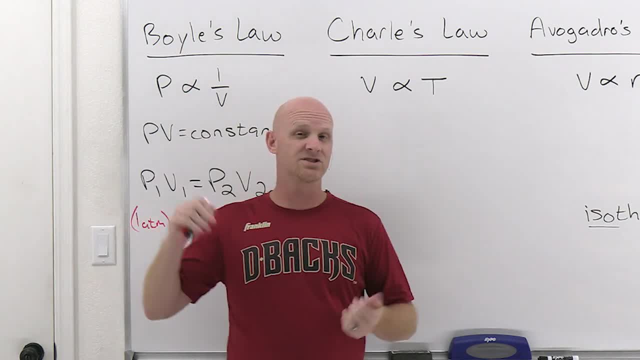 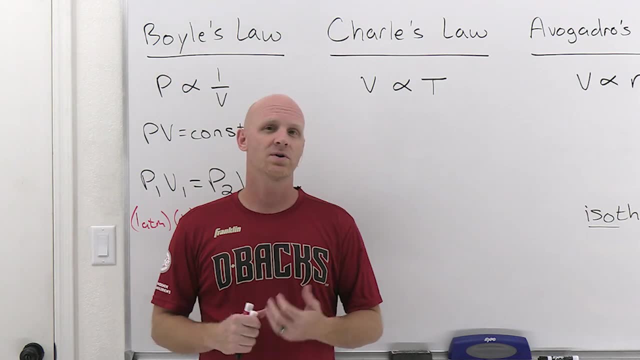 Celsius. you know Mr Celsius or Centigrade, or I don't know if that's his real name or where the nature of that name comes from, but the Celsius scale does not have a true zero, So he just you know. 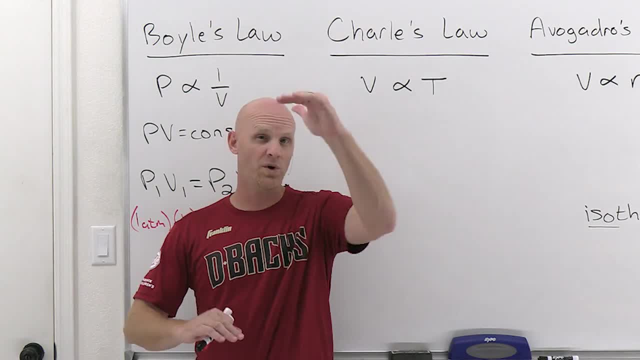 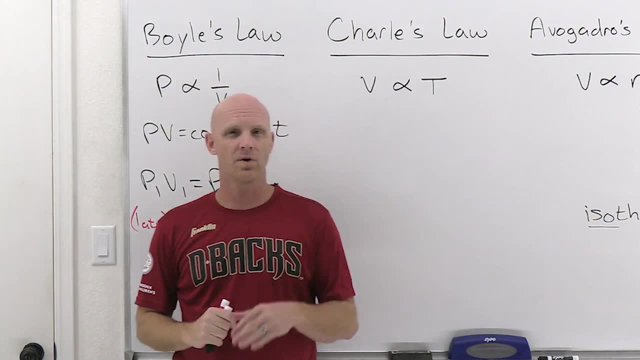 Mr Celsius saw where water froze and boiled and made those the 0 and 100 marks on his scale and then just divided the difference up into 100 little degrees. So but you can go colder than zero. That's what I mean by it's not a real zero. 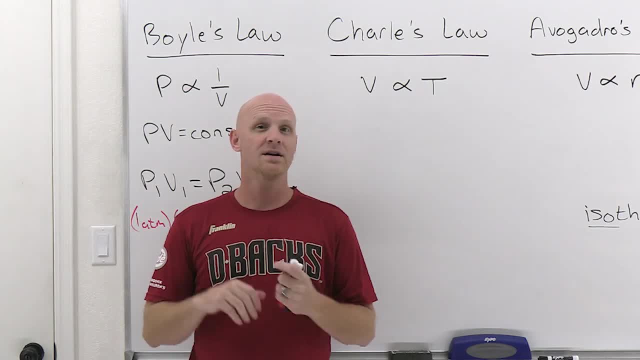 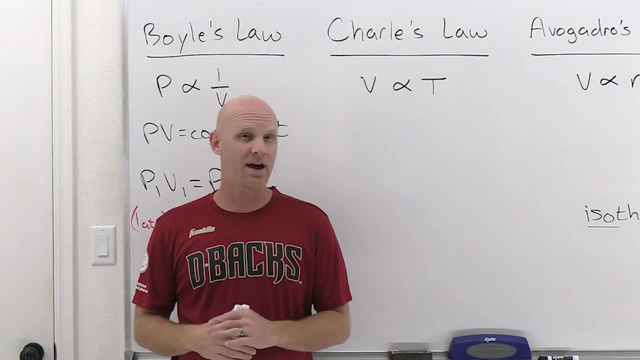 It's not the absolute zero. That's what we get on the Kelvin scale, though. So absolute zero Kelvin is the complete absence of heat. You can't have a lower temperature than that, And so that's what I mean by having a real zero. 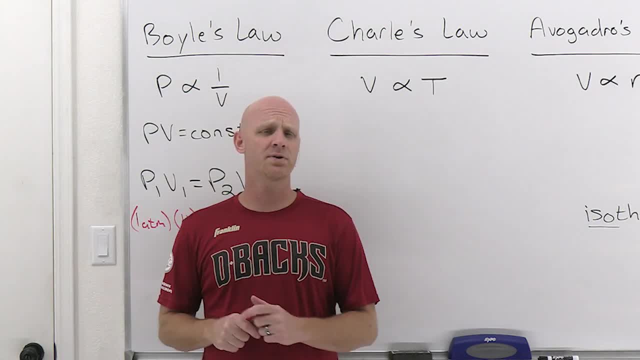 So it's kind of like I decided: let's say that I'm the most important person in the universe and I'm the standard by which all other things are measured. So you know, I'm 5'8" and so 5'8". 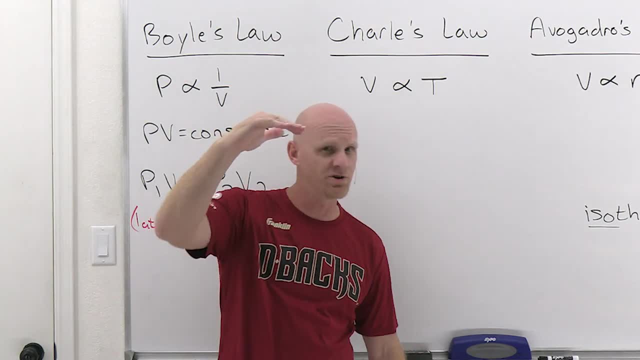 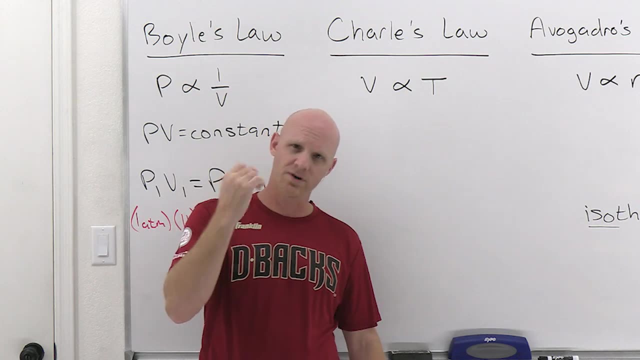 on the new Chad scale is the new zero, And so if you're 5'9", well, on the Chad scale, you'd only be one inch tall. If you're 5'8", you're six foot, you'd only be four inches tall. 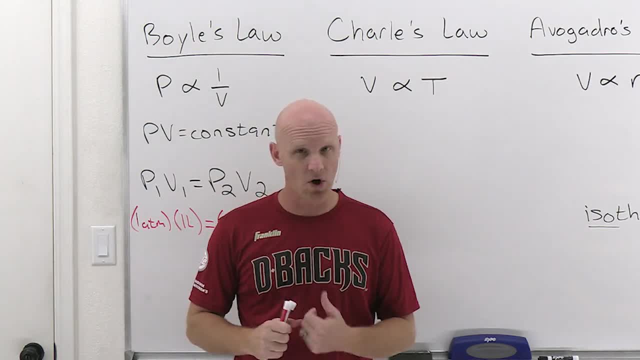 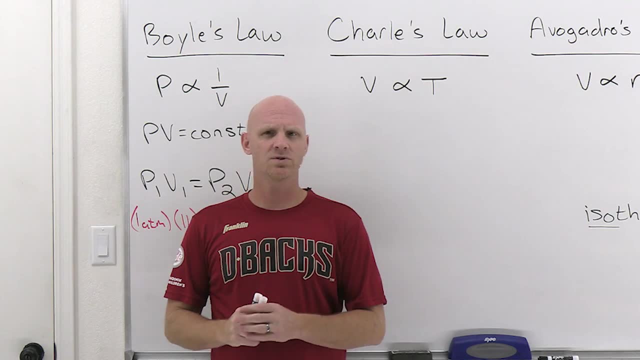 If you're 5'2", you'd be negative six inches tall on this new Chad scale. Well, obviously, 5'8" is not a real zero. So, and in this case, if I told you somebody, you know who is. 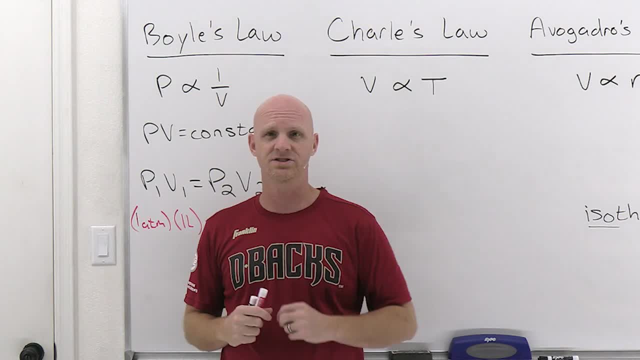 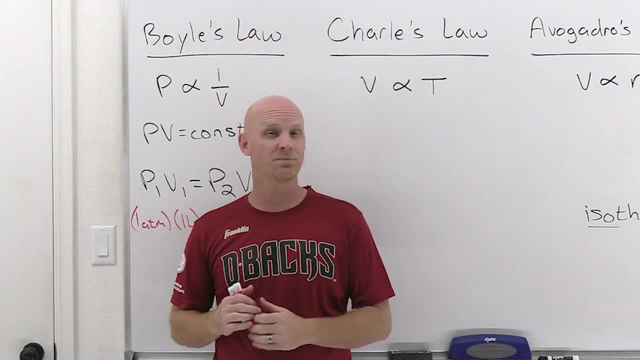 you know, say, two inches on the Chad scale versus four inches on the Chad scale. would it be accurate to say that the person who's four inches tall on this fictitious Chad scale is twice the height of the person that's only two inches tall? 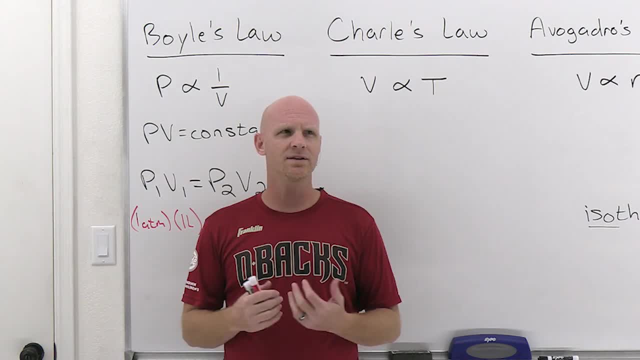 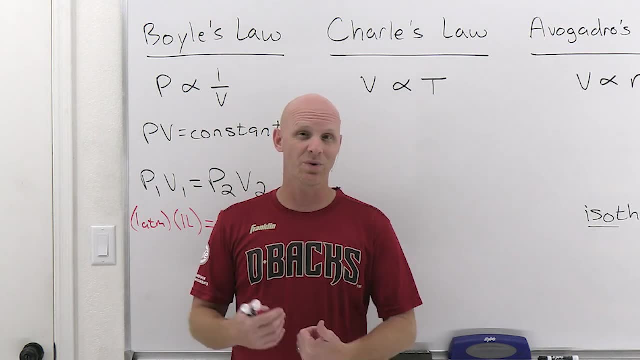 Well, no, Because again, two inches versus four inches on the Chad scale is five foot ten versus six foot tall, And that's definitely not a difference by a factor of two. And so when you don't have a real zero, you can't actually use that scale. 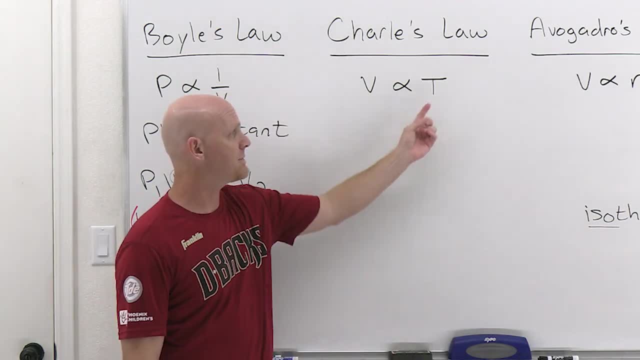 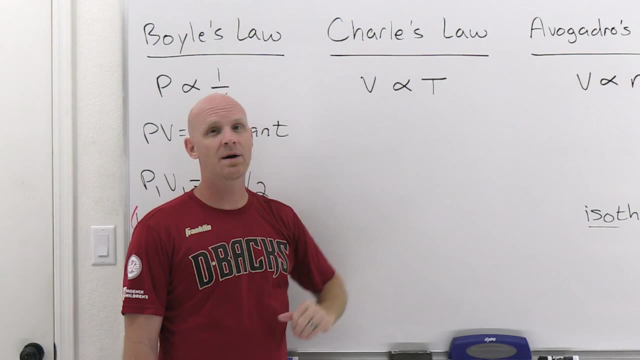 to talk about like doubling and tripling. And that's why, in this particular chapter, when we're talking about like proportionalities and stuff like that, we have to use the Kelvin scale. So volume is direct proportional to temperature. but make sure you're doing. 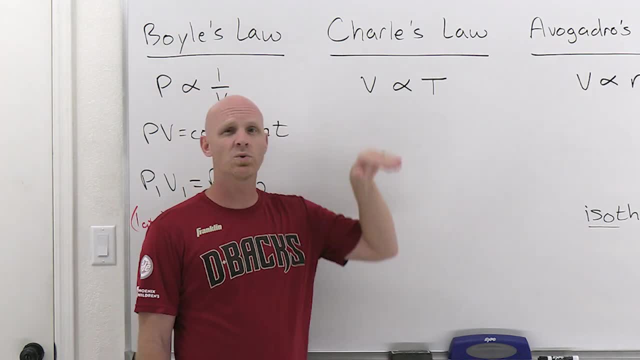 in Kelvin. So if I told you that you know I increased the temperature from 10 degrees Celsius to 20 degrees Celsius, you're supposed to realize: oh, that's Celsius, That's not. a doubling to 20 Celsius would be. 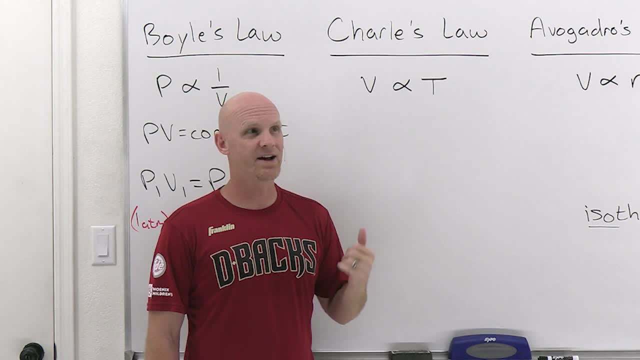 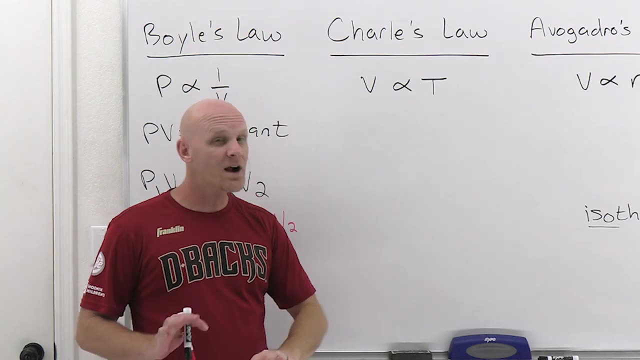 you know, 283 Kelvin to 293 Kelvin, which is like less than a 10% increase, And a less than 10% increase in temperature should give you a less than 10% increase in volume. So be careful on. 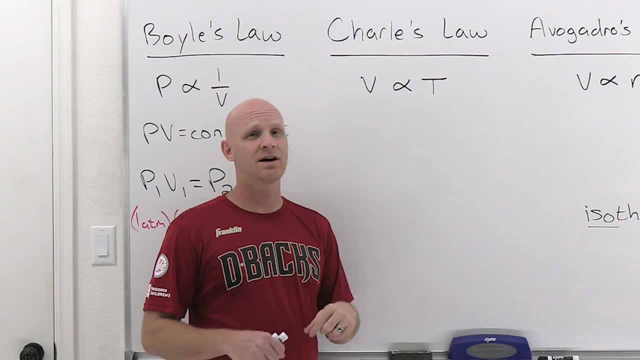 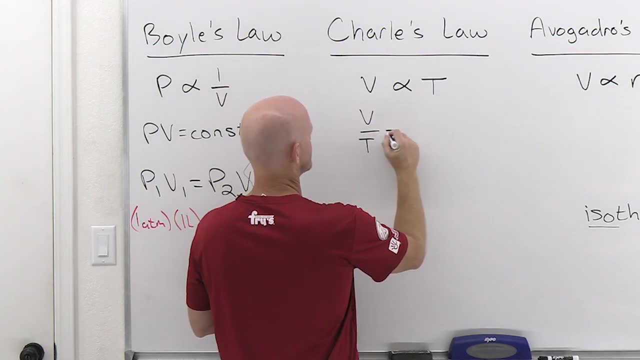 you know temperature in this chapter, Everywhere in this chapter, you should definitely use it in Kelvin, All right. Another way to express this, though, is to say that volume over temperature equals a constant, And so, if this ratio always gives you the same constant, 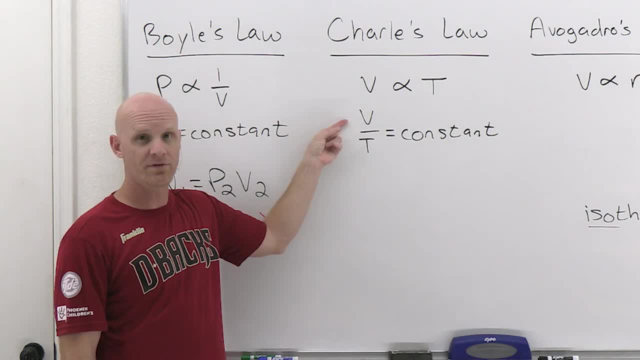 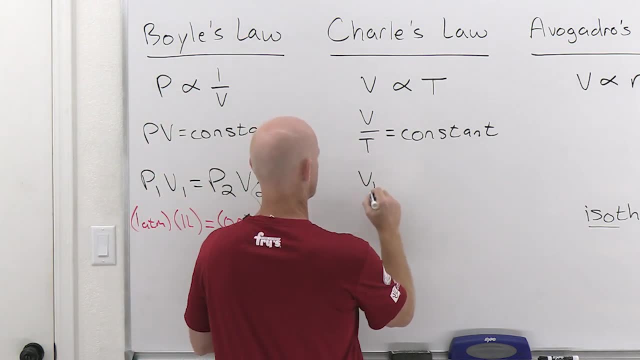 if you double the temperature again in Kelvin, you'd also have to double the volume, so that this equals the same exact ratio, the same exact constant. And another way to say that would be: V1 over T1 equals V2 over T2.. 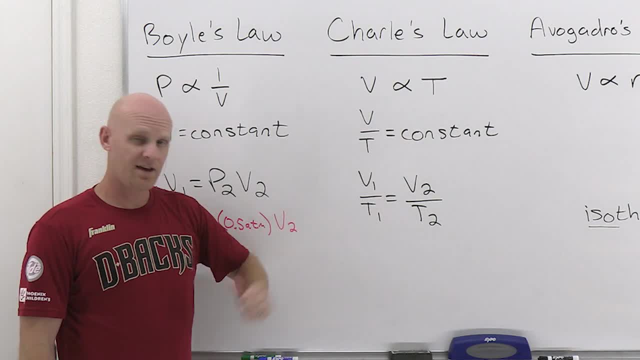 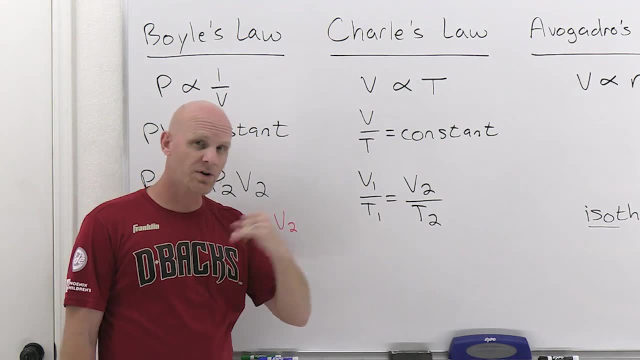 And similar to what we had over here. so if I give you, you know, any three of these conditions, so I'm gonna have a gas in our two sets of conditions, in this case, where the number of moles of gas 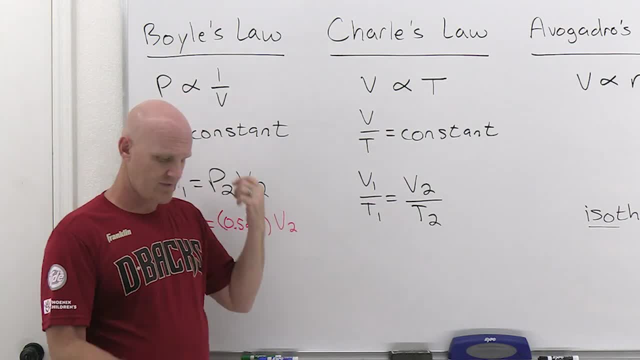 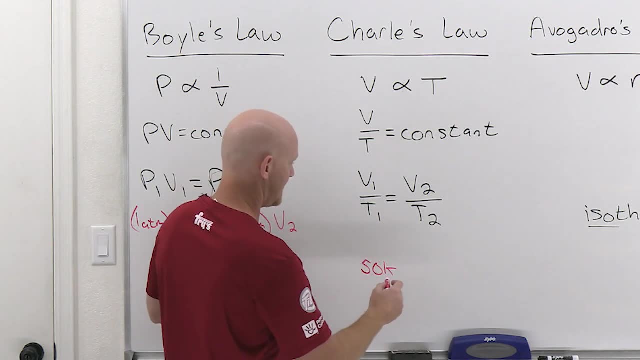 and the pressure are held constant. So if I told you that I had a gas at an initial temperature of 50 Kelvin and then I'm gonna change it to being at a final temperature of 100 Kelvin, and if its initial volume is one liter, 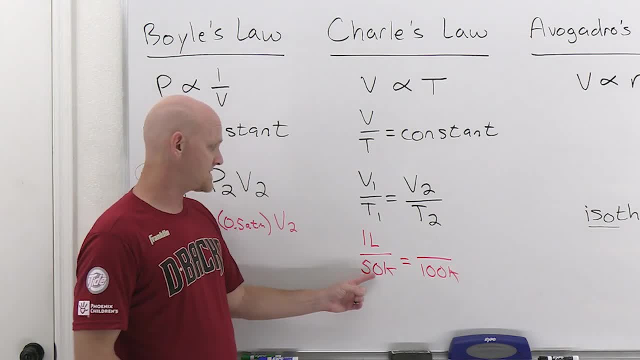 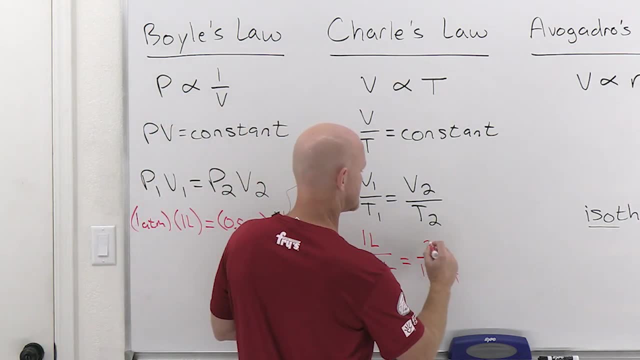 and then I say: well, what's the final volume gonna be? Well again, in this case, on the Kelvin scale, I doubled the temperature, which means the volume should also double and therefore go up to two liters That way. 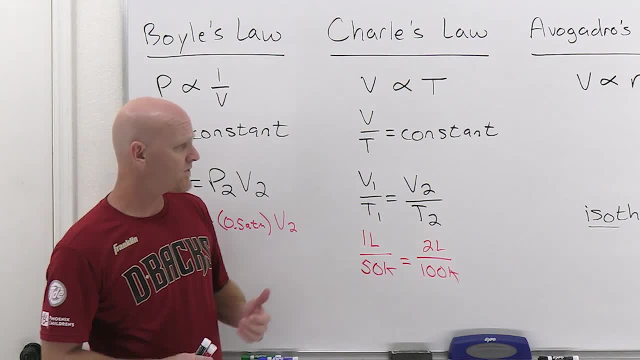 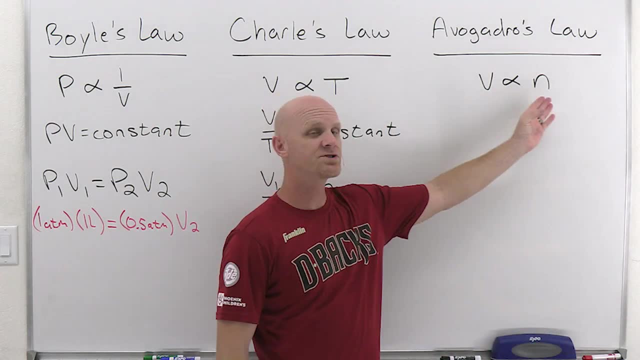 one over 50 and one over 100 maintain that equality. So that's Charles' Law. And then, finally, we'll make our way over here to Avogadro's Principle, And again we're gonna say that volume is proportional to the number. 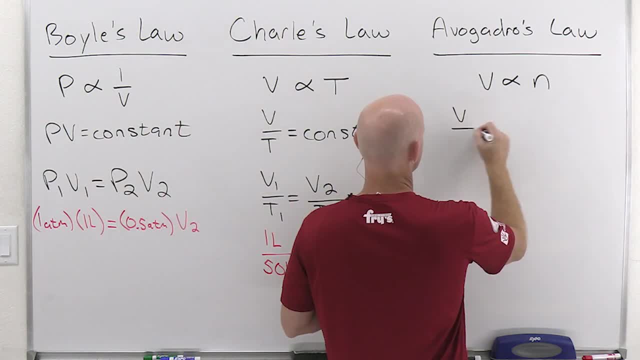 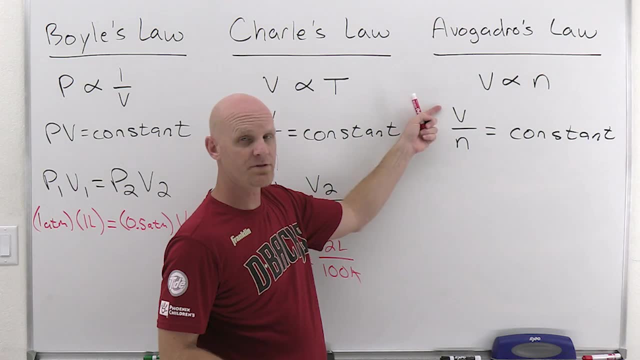 of moles of gas, assuming pressure and temperature are held constant. Another way to say this is to say that V over N that ratio is equal to a constant. Once again, if you double the number of moles of gas, you'd have to double. 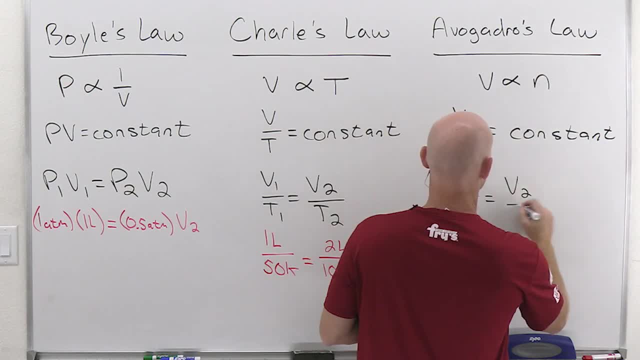 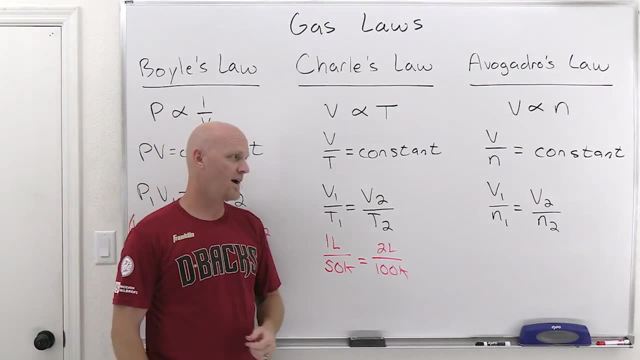 the volume, so that this ratio of N1 equals V2 over N2, just analogous to what we saw with Charles' Law, with temperature instead of with moles of gas, But pretty much exactly the same. So these are the different ways you can express. 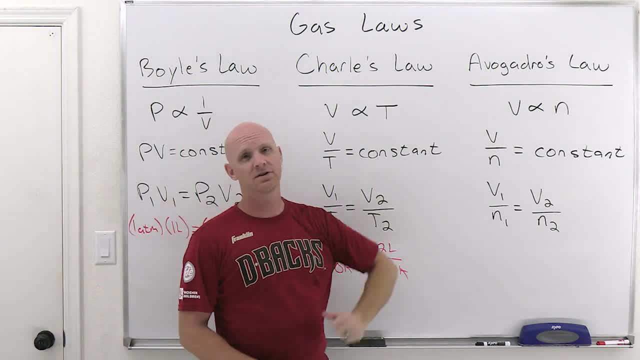 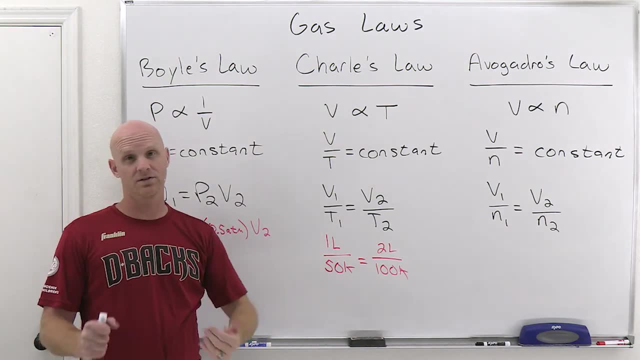 these three lovely glass laws. You should understand all three of them for each, because you could get, you know, a question on the test that just says which of the following is an expression of Charles' Law. Well, you've got three possible. 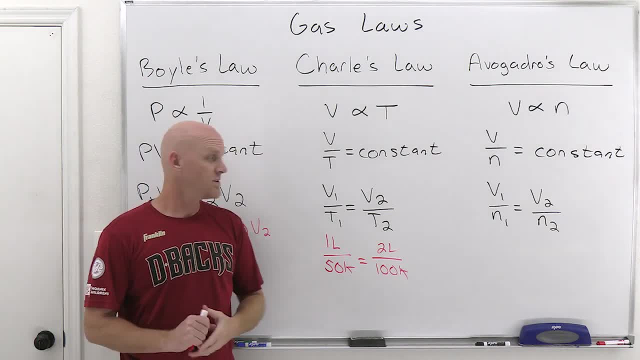 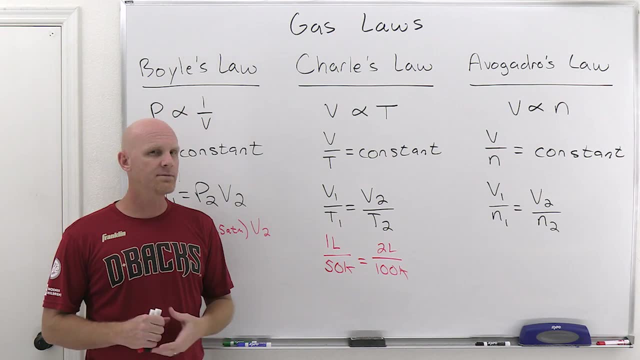 correct answer choices that could show up there. You should also be prepared to do some basic calculations with these. However, we'll see in just a sec that you know more than likely, you're probably just gonna take a look at using the combined gas law. 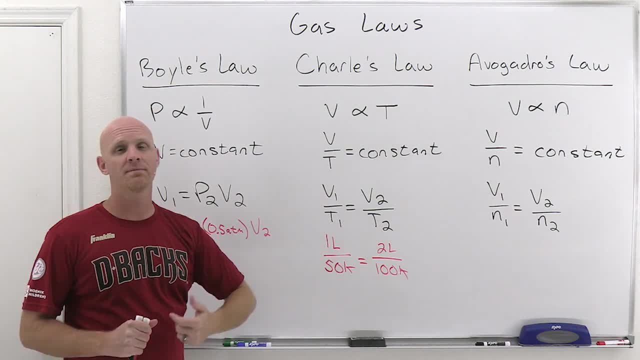 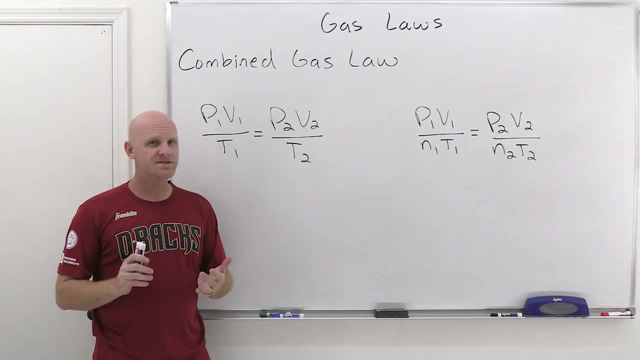 instead of one of these individual ones, because that combined gas law can essentially reduce to any one of these once you realize which variables are being held constant. All right, so now we're gonna move on to that combined gas law And the combined gas law. 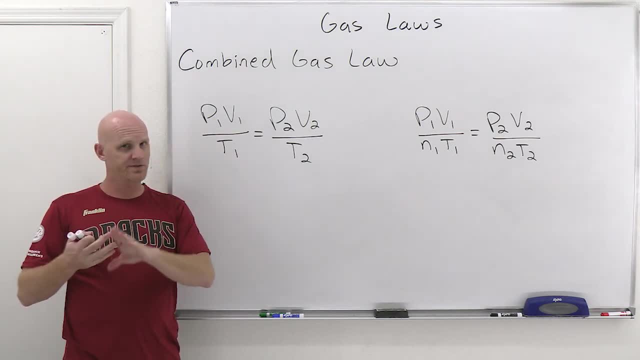 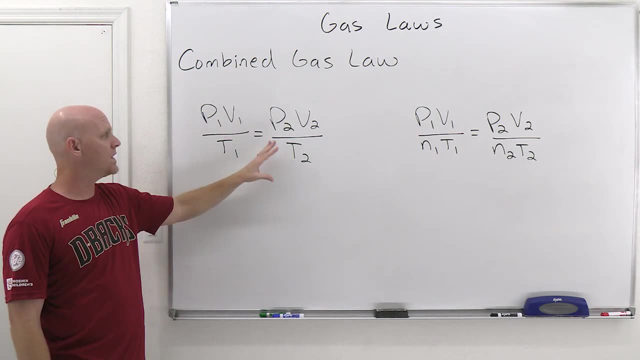 just essentially combines Boyle's Law, Charles' Law and Avogadro's Principle into one, And technically it actually doesn't even combine Avogadro's, but we will So. but if you combine Boyle's and Charles' into one, 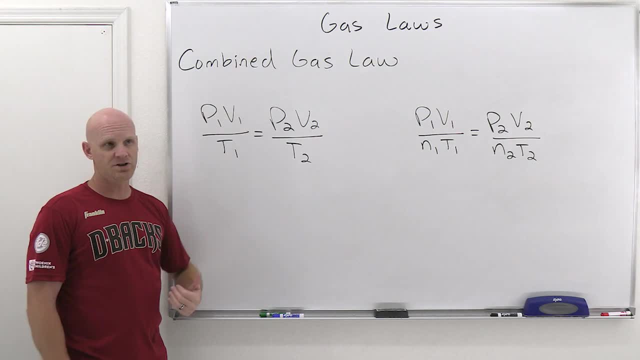 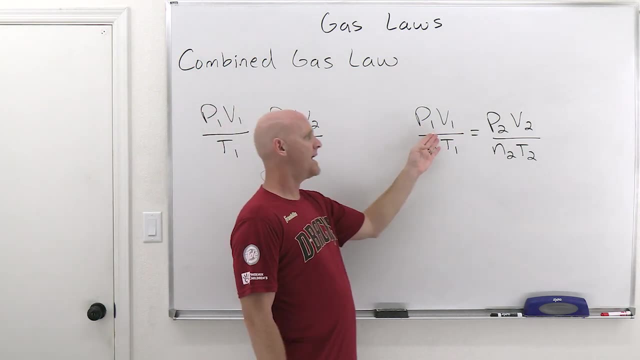 you get: P1V1 over T1 equals P2V2 over T2.. And now you can actually look at changing not just two variables, but now three. Well, technically, if we throw Avogadro into there as well, now you actually get. 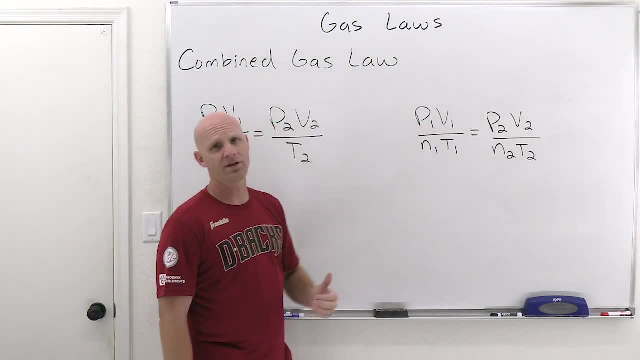 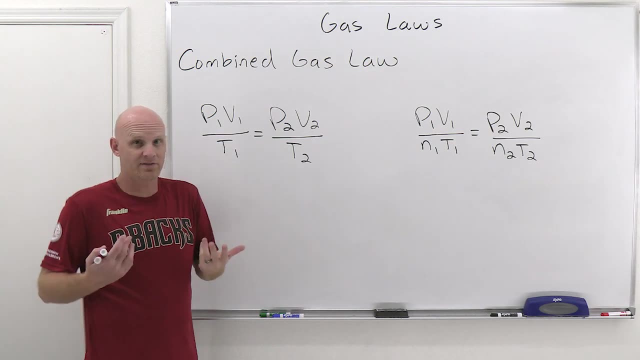 P1V1 over N1T1 equals P2V2 over N2T2.. And I'm really disappointed that in the actual combined gas law they don't usually include the number of moles. Well, what if you actually add more moles of gas? 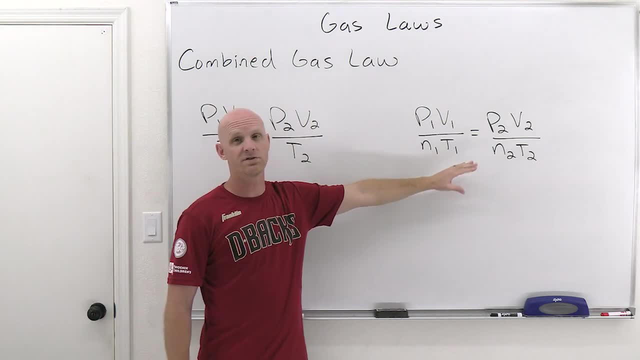 and you don't account for that. Well, you don't with the combined gas law, So this is what I call the better combined gas law. You're probably not going to find it in your textbook or anything like that, So, but it does allow us. 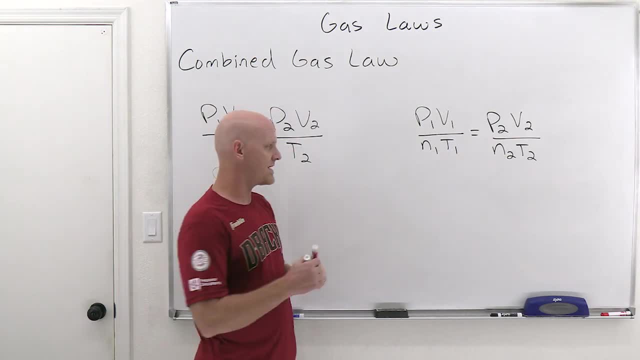 to account for the number of moles. Now one thing to note, because this is not going to be in your book. it's probably not going to be on any summary equation sheet or anything like that for you. So one thing to note. 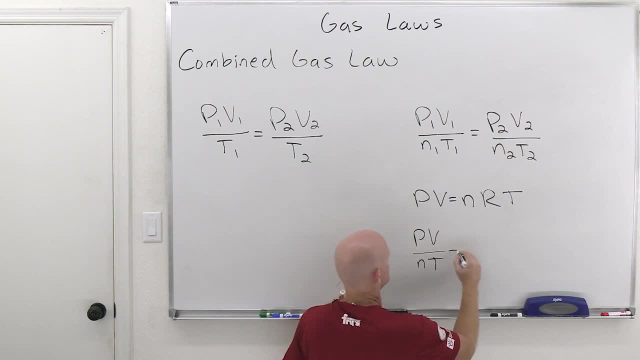 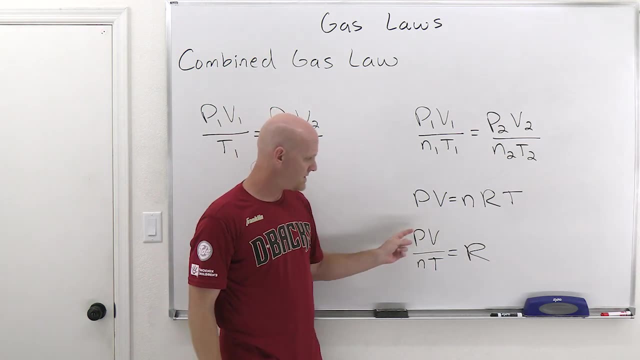 if you look at your ideal gas law, which we have not covered yet, which is the ratio of PV over NT equals R, And it turns out R is a constant. And so if this ratio, PV over NT, equals a constant, so it will, then 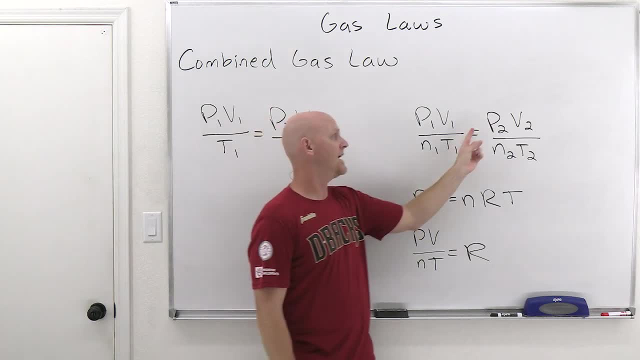 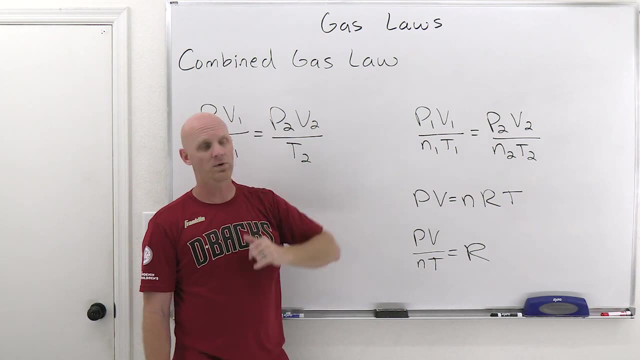 under one set of conditions, that ratio is going to equal the same constant as it will under a second set of conditions, And you can derive this better combined gas law from your ideal gas law that we'll learn about later on in this lesson. So 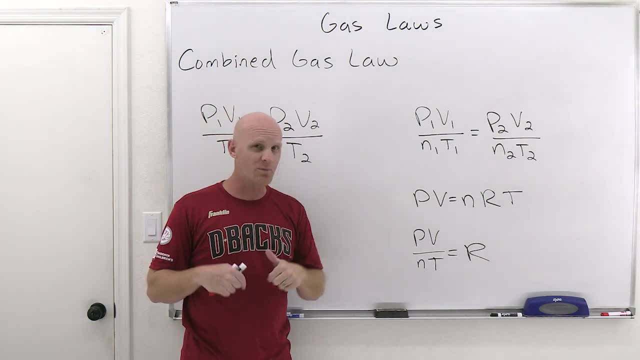 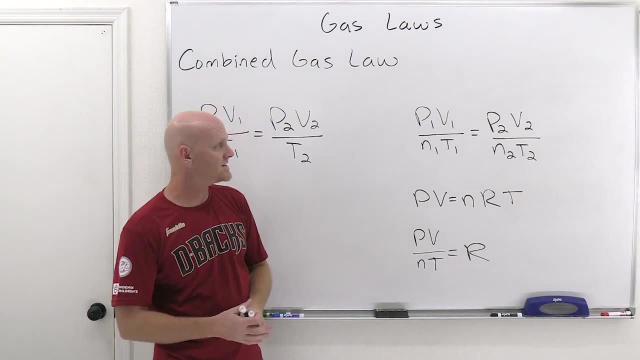 I just want to pull that out. I realize we haven't covered it yet, but we'll get to it in this video And hopefully a good chance. you've seen it in class already, So but we'll get here to this ideal gas law. 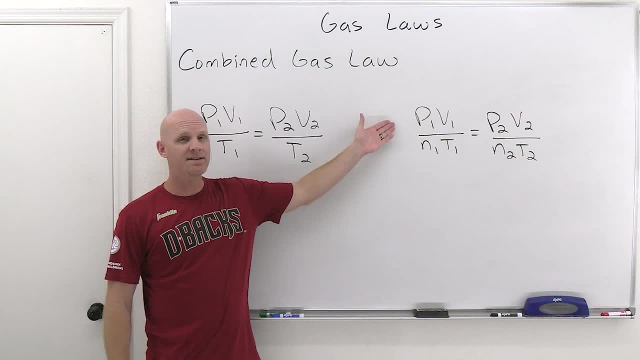 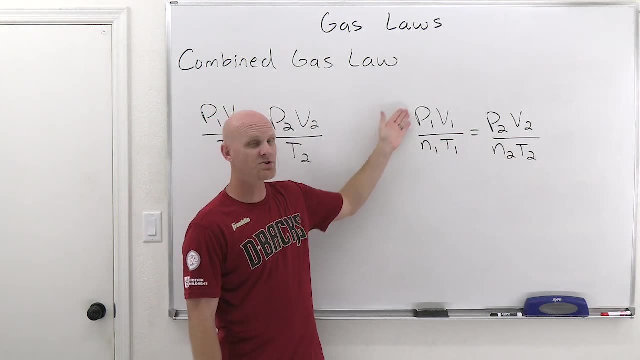 in just a little bit, All right. So for this combined gas law, essentially you've got two sets of conditions And you could have. you know, we've really got four initial conditions, four final conditions, as many as eight variables. 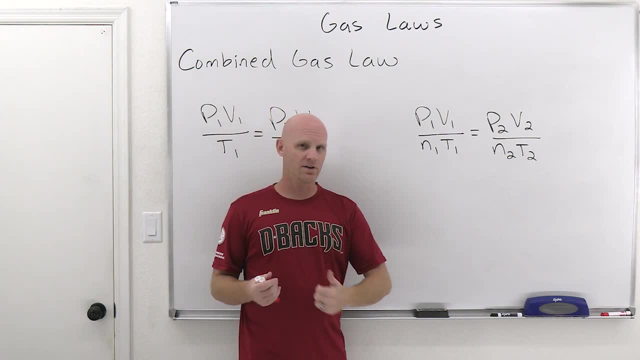 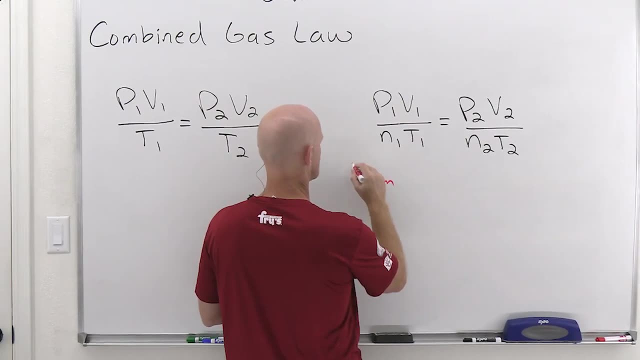 And I give you seven, you solve for the eighth. Well, you know, if I gave you a specific sample of a gas at a pressure of one atmosphere, okay, so initial pressure is one atmosphere with a volume of one liter. okay, 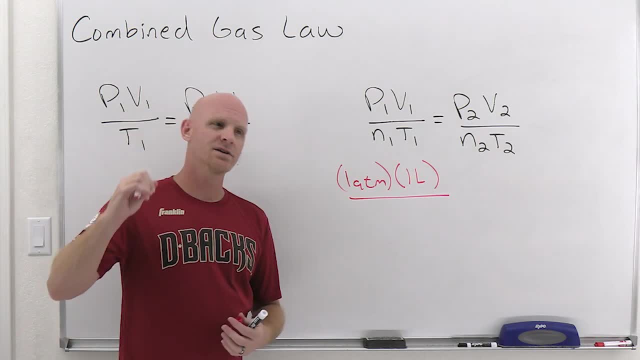 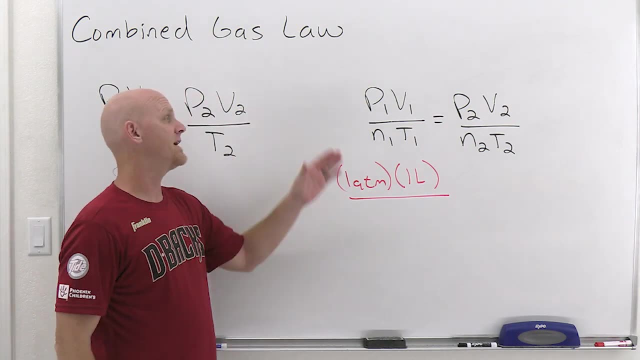 so, and a temperature of, let's just say, zero Celsius. Well, again, on this you got to be careful. Temperature's always got to be in Kelvin, everything you do in this chapter. Now it turns out pressure and volume. 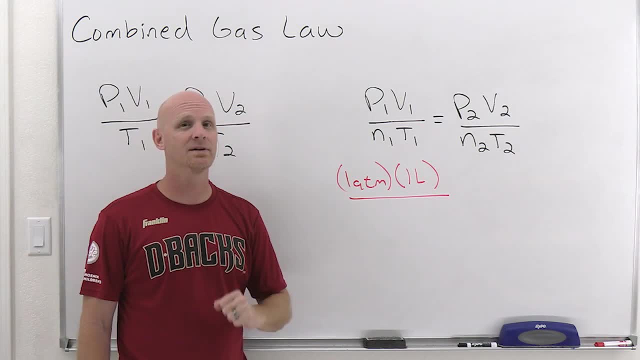 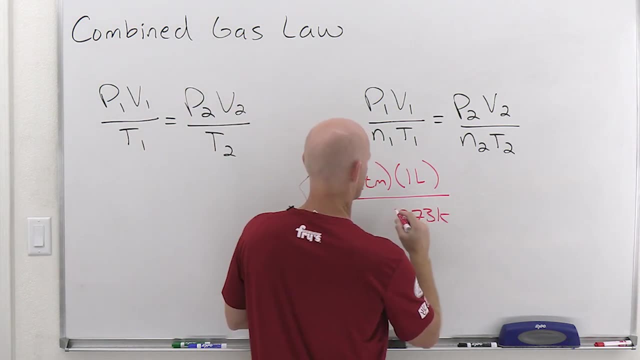 as long as you use that absolute scale, has to, has to, has to be in Kelvin. And so if I say zero Celsius, you're supposed to know: oh, that's got to be 273 Kelvin. So, and then I'm just. 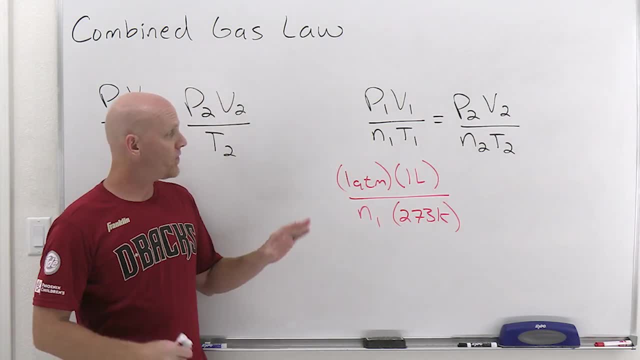 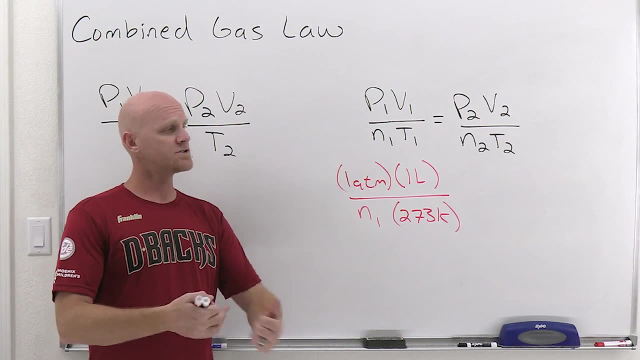 going to call this N1.. I don't tell you how many moles of gas we have, but we're going to alter the conditions for a specific sample of gas, And so we're just going to change the conditions. We're not going to. 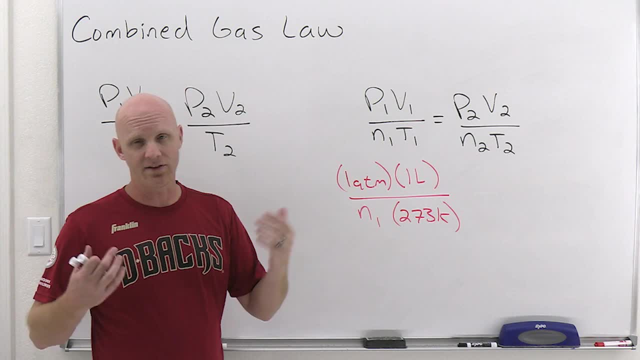 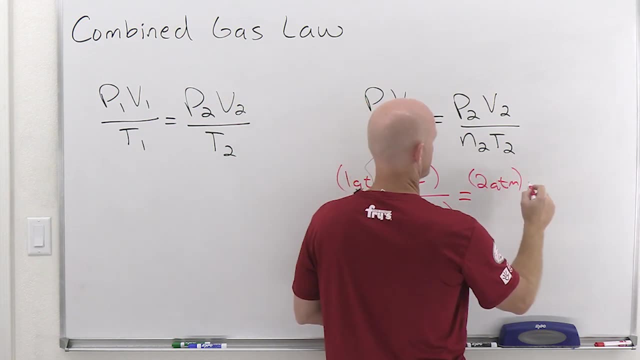 add any more gas to it. We're not going to remove any gas from it, And so we'll find out that, in this case, I'm going to change the pressure to two atmospheres, And the question's ultimately going to end up being: 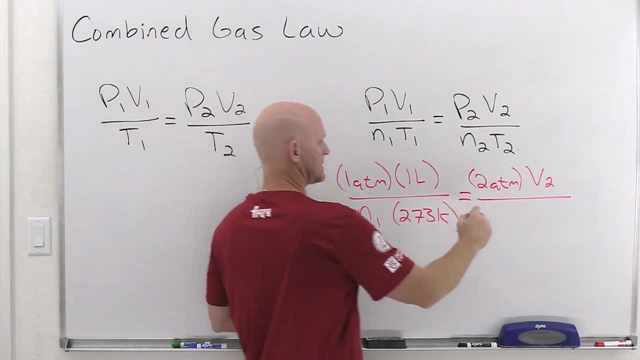 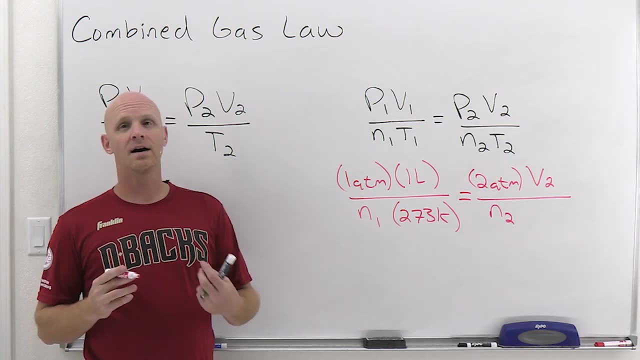 what is the volume? So? but we've got the same sample of gas. I'll come back to N2 in a minute, And then we're going to change the temperature up to 273 Celsius, which is 546 Kelvin, And so 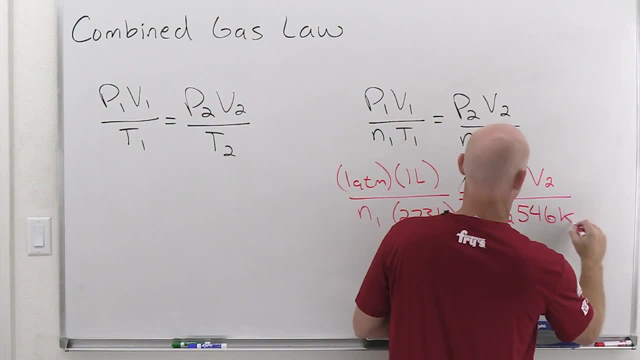 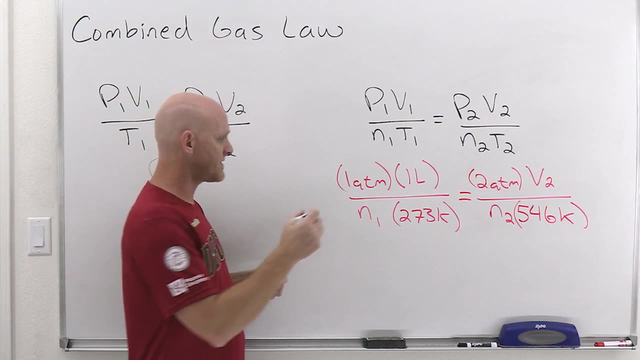 once again. in this case, though, N1 and N2, it's the same sample of gas. I haven't added two at a. I haven't added two at a. I haven't removed anything from it, So those are going to be equal. 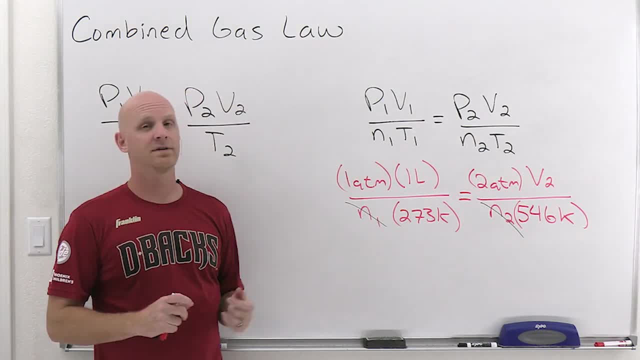 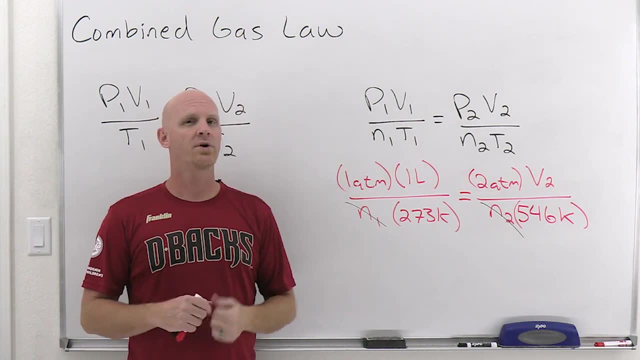 We'll get rid of those. And the question is: what is the final volume of this gas? Well, we can kind of look at this and look at things individually here. What did I do to the pressure? Well, I doubled the pressure. 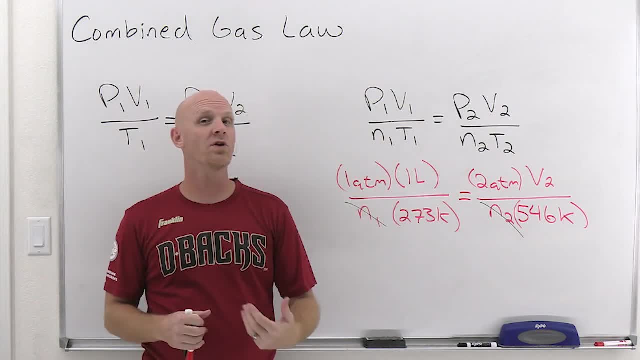 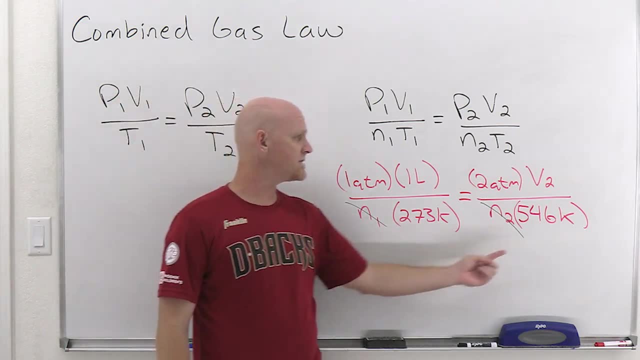 If I isolated that alone, what impact would that have on the volume? Well, pressure and volume are inversely proportional. So if I double the pressure, that should cut the volume in half. Okay, Well, let's go take a look. 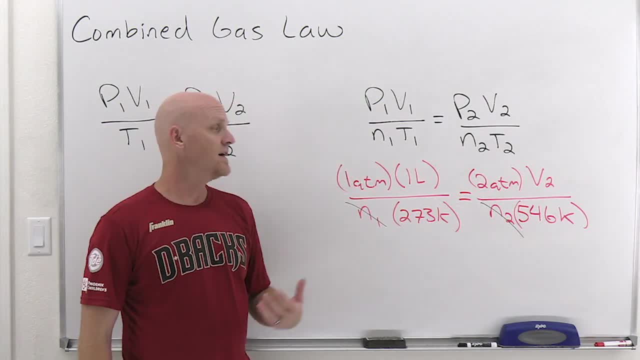 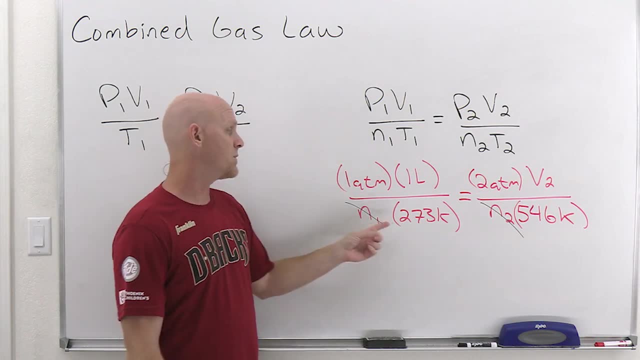 at temperature For temperature. here we're on the absolute scale, And double the temperature, it should double the volume, Charles' Law. Well, based on what we did with the pressure, the volume should be cut in half. Based on what we did. 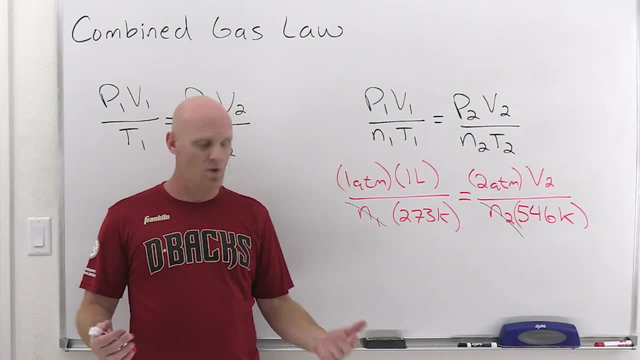 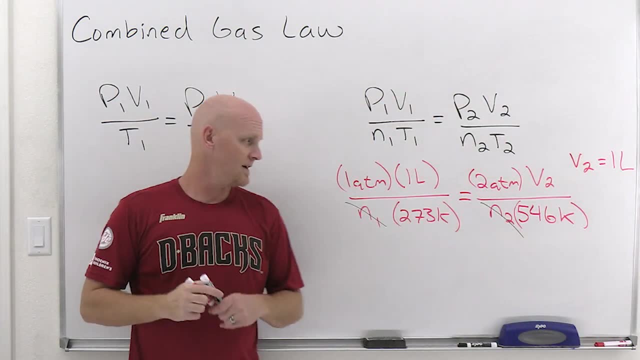 with the temperature, the volume should double, And factoring both those in actually means we're going to get no volume change, And if you actually solve for V2 here, you're going to get that it's still equal to one liter. So 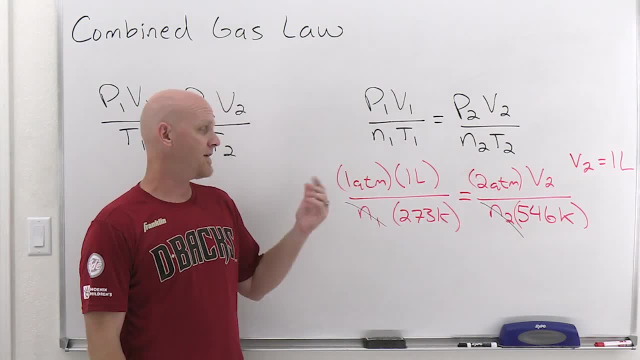 but that's how you could plug in all the variables you're provided with And again, had the- let's say we just hadn't changed the temperature- Well, we could have canceled out of the equation. Cool, So ultimately you can get. 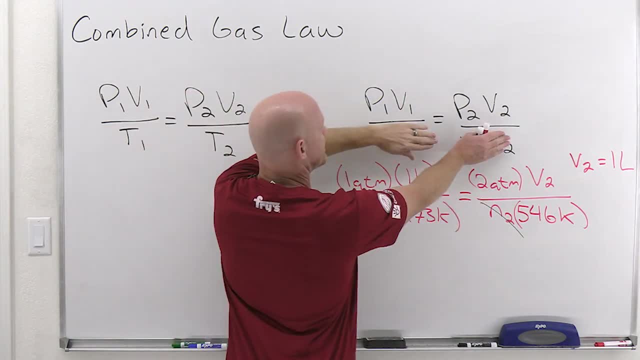 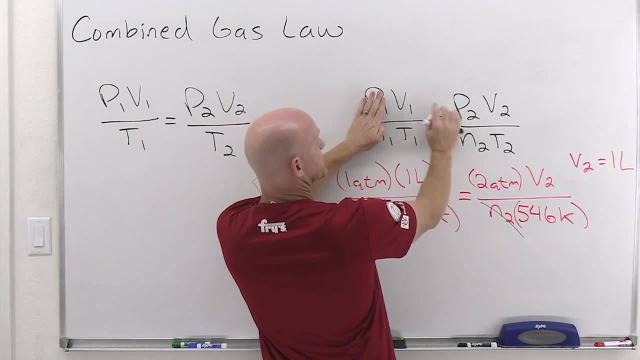 Boyle's Law out of this. If you keep N and T constant, well then these cancel and you're just left with P1B1 equals P2V2, Boyle's Law. If you hold P and N constant, well then P1 and N1 and P2N2. 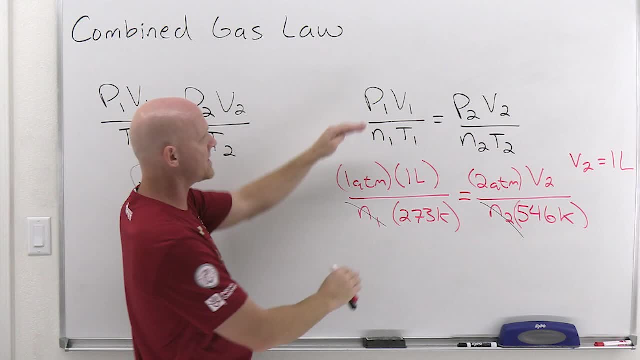 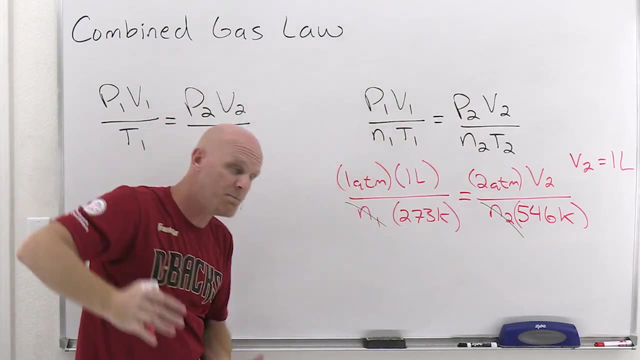 cancel and you're just left with Charles' Law. And if you hold pressure and temperature constant, then you're going to be left with Avogadro's Law, And so all those other laws can be derived back from here. But the truth is, 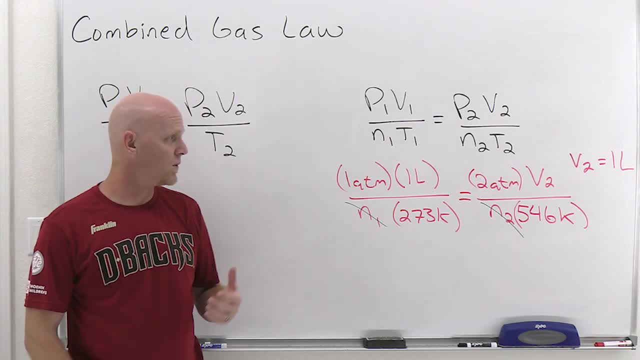 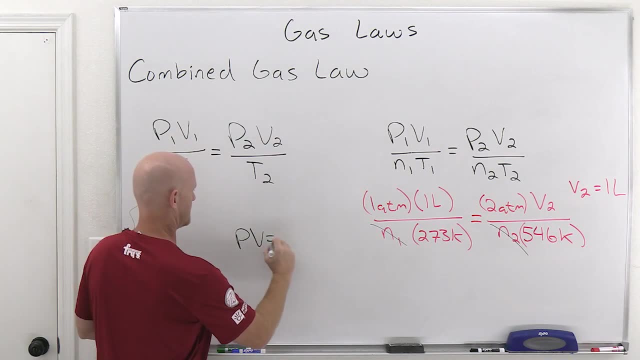 again, it's better. combined gas law, Cool. Now one thing to note: we're going to talk about the ideal gas law soon, So, and again, that's going to involve an equation: PV equals NRT And a lot of students. 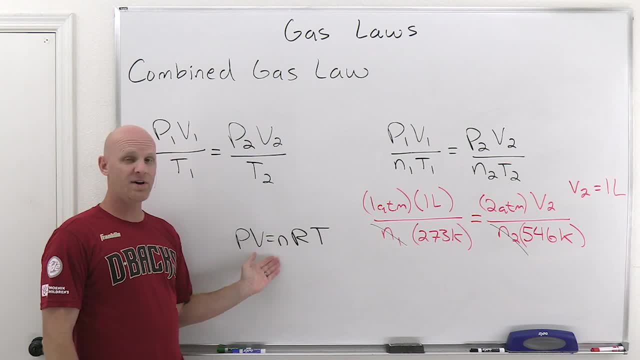 don't know well when would I use the combined gas law versus, you know, the ideal gas law? Well, how do you know? Well, again, the big thing is this: The ideal gas law. you have one set of conditions. 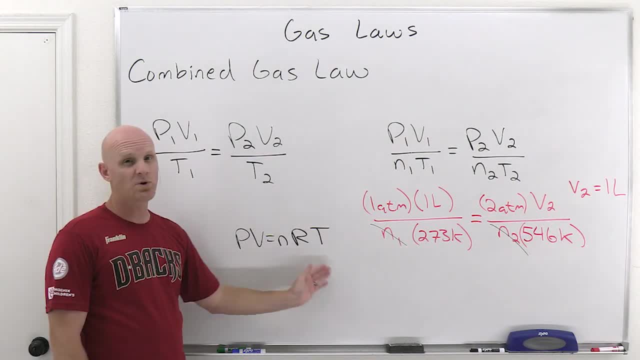 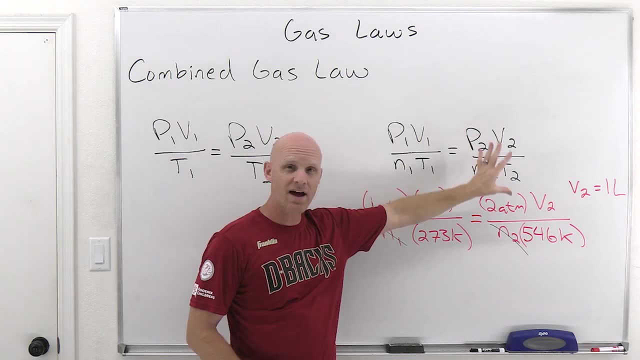 You don't have a single temperature and then that's a constant And you're going to get three out of the four provided typically and solve for the fourth. But the combined gas law deals with one set of conditions and then you're altering it to give a second set. 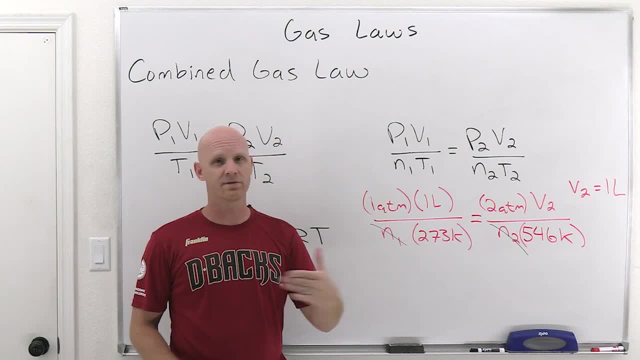 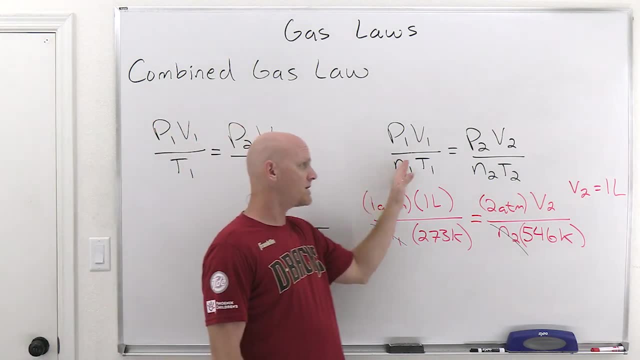 of conditions And you're given everything except one variable under either the initial or final set of conditions. So the real question comes down: do you have just one set of conditions? You're probably doing the ideal gas law calculation If you've got parts. 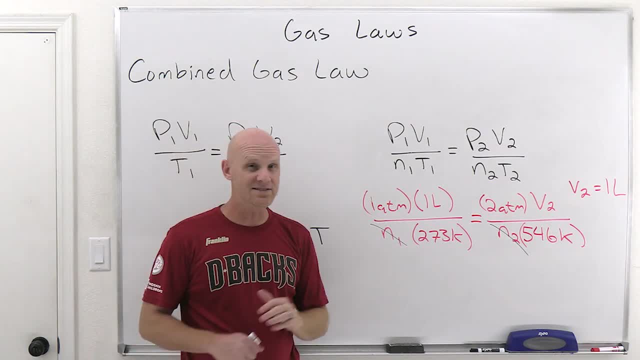 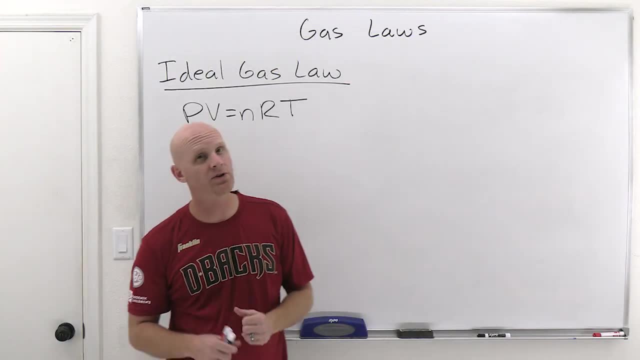 of two different sets of conditions, you're probably doing the better combined gas law in this case instead. Cool, So let's take a look at that ideal gas law. All right, So now we're going to deal with the ideal gas law. 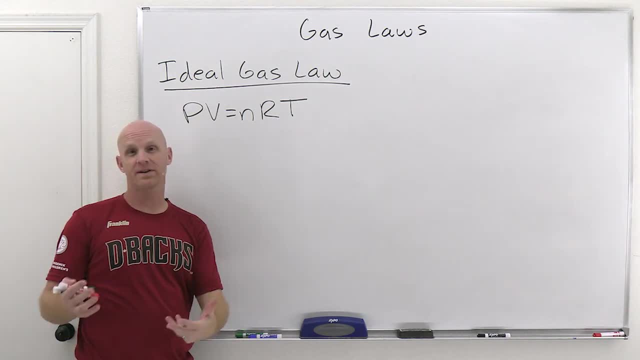 So PV equals NRT and we call it the ideal gas law. Some books will call it the perfect gas law, So either way. So, but it's the ideal gas law and the reason we call it this is that only a gas. 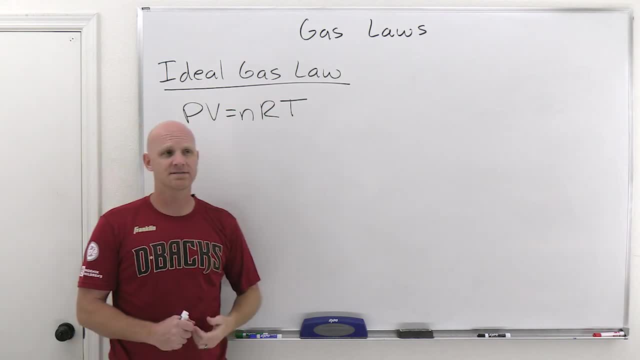 that's behaving ideally will follow this law. And so it turns out, not all gases exhibit ideal behavior, or at least more commonly. what you're really going to see is that not under all conditions, And so there's no such thing as an ideal man. 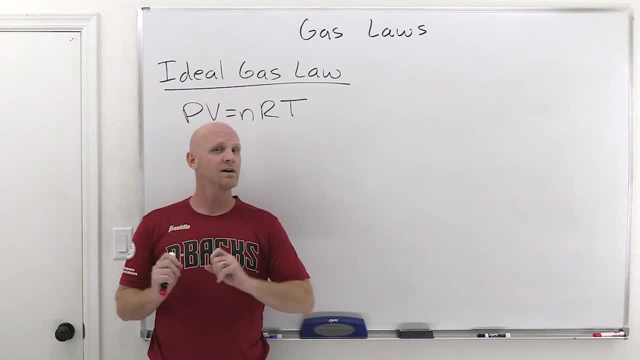 and they don't exist. There's no such thing as an ideal man. There's no such thing as an ideal gas. However, there are conditions where both gases and men are more likely to behave ideally. Now we'll learn about what those conditions. 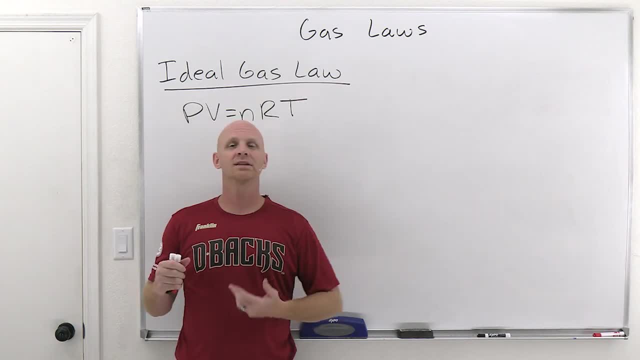 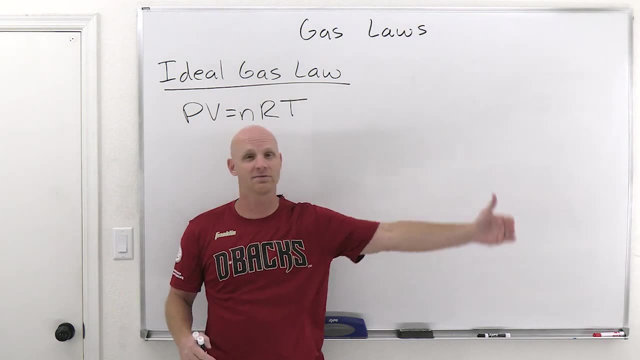 are for a gas here in a little bit. But for a man those ideal conditions would be like a first date. So a man is much less likely to do rude things and things of that sort on a first date, as opposed to say after being married. 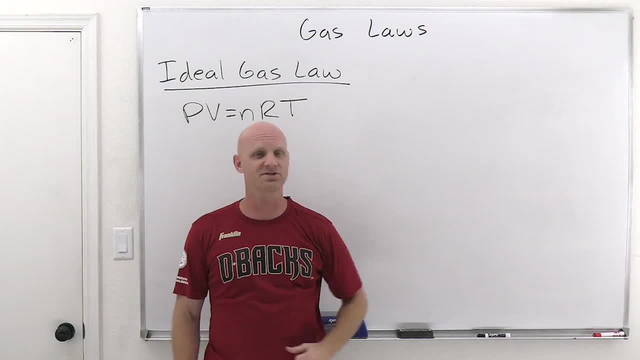 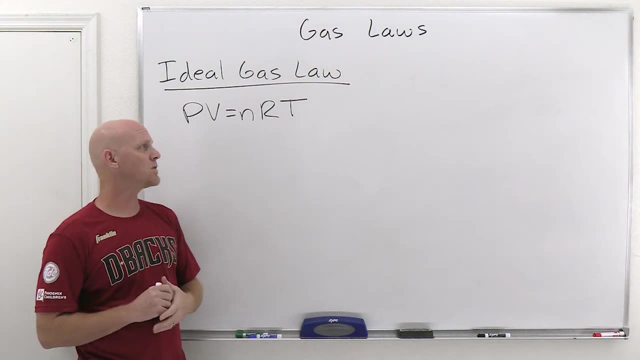 for 20 years and things of this sort, As opposed to being married for 20 years or something like this. So ideal gases: again, it turns out they don't exist. However, we'll find out in a little bit. we'll talk more about it. 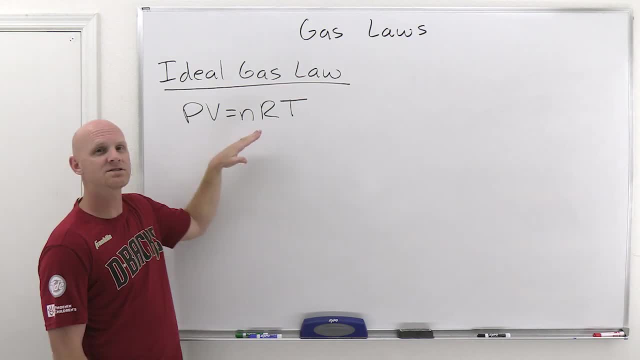 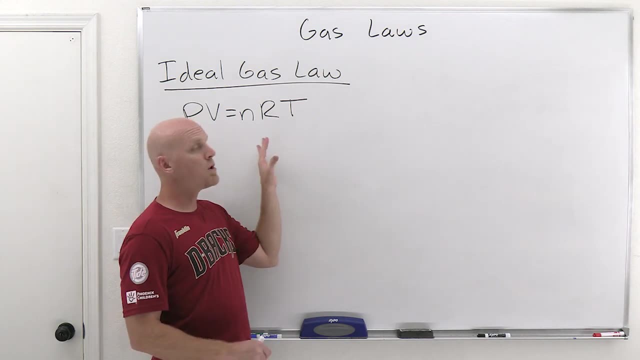 in a second that under conditions of low pressures and high temperatures. that's when gases are most likely to obey this lovely mathematical expression, the ideal gas law, And we'll review that again a little bit. So it turns out. this is all part. 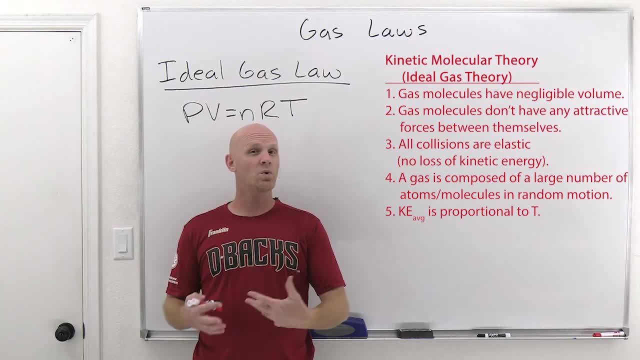 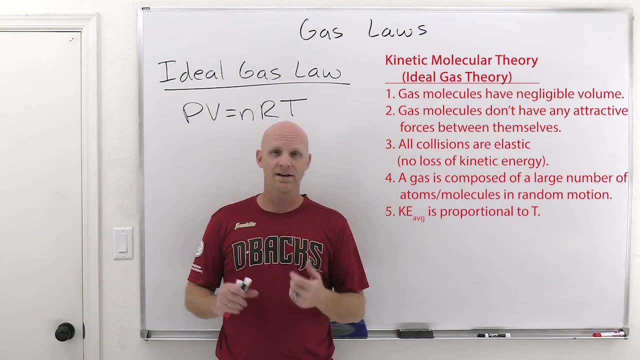 of what we call kinetic molecular theory, and I'll put it up on the board over here. And so first one is that the molecules themselves take up negligible volume. So it turns out, most of an empty gas is made of empty space, under conditions, 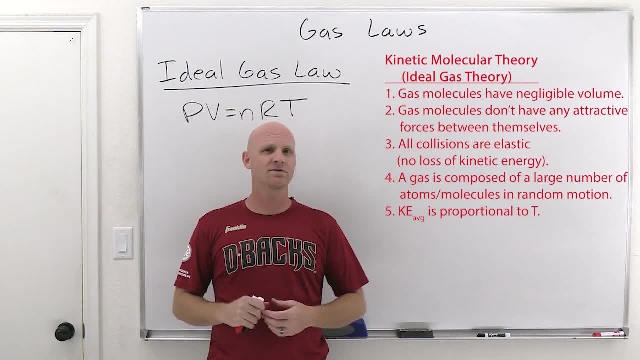 of what turns out low pressure. That'll kind of be what governs it here. So in a gaseous phase the molecules and atoms again are separated by a fair amount of empty space, so much so that the percentage of the volume 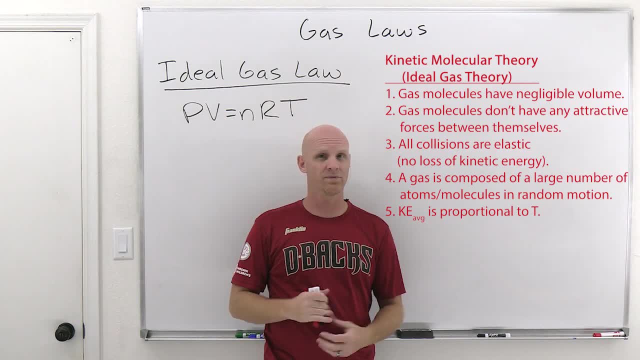 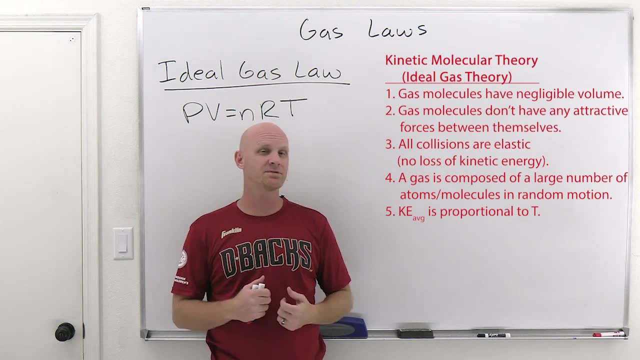 of an entire gas taken up by the little molecules that are spread out themselves is going to be so small- a fraction of the total volume that's actually again taken up by the molecules, instead of empty space that we're just going to round it down to zero. 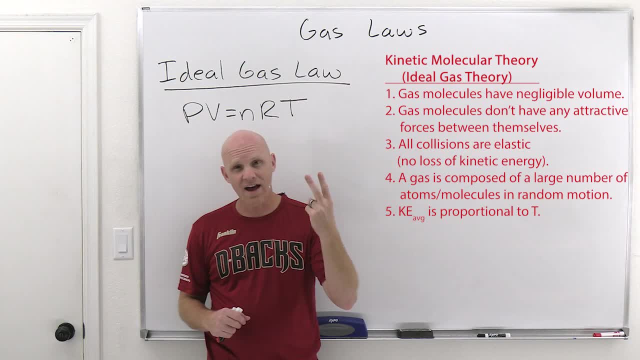 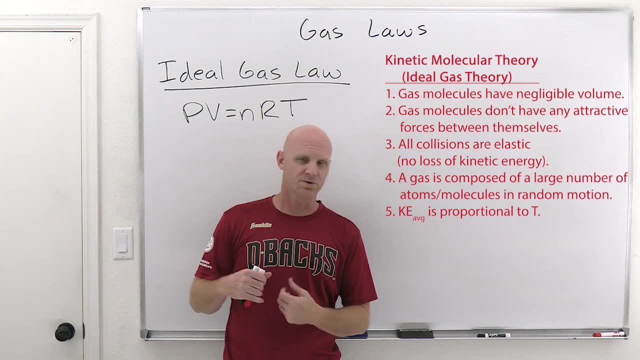 and say that the gas molecules have negligible volume. That's tenet number one. Now the second thing we're going to say is that the gas molecules have no attractive forces. So I mean technically you might say they have no repulsive forces either. 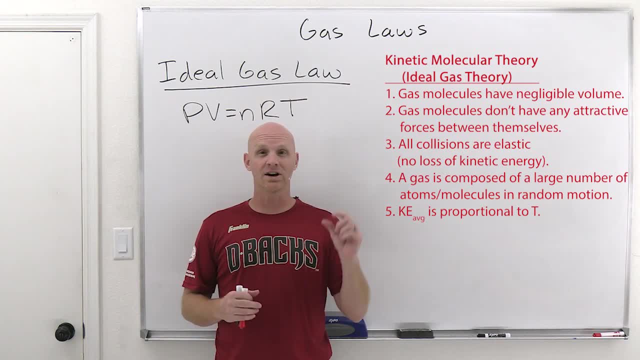 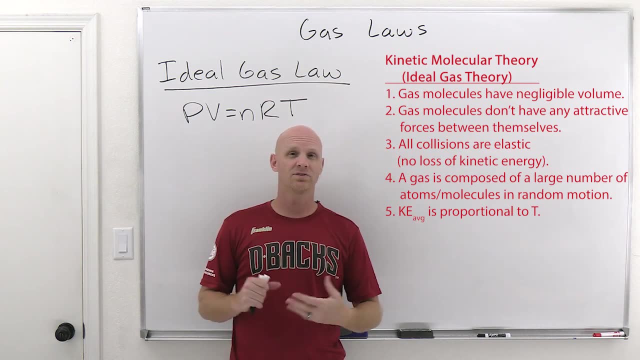 but it's the attractive forces we're worried about, because it turns out all molecules are at least a little bit sticky, And so zero attractive forces is not a 100% correct statement, but it is one of the tenets or postulates of kinetic molecular theory here. 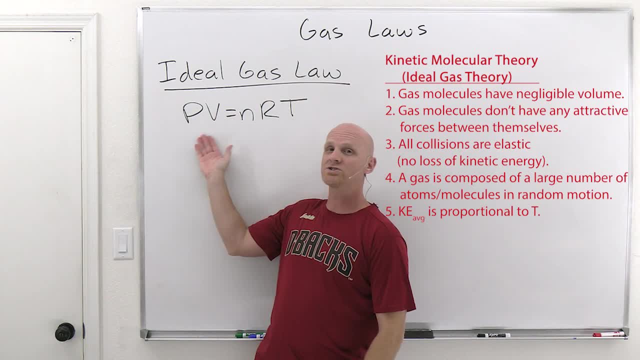 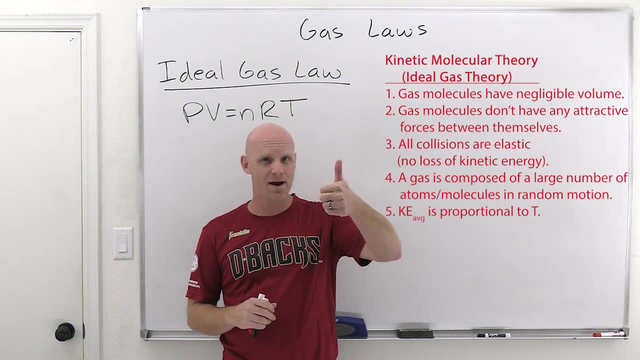 and it is one of the tenets that needs to hold true for this equation to describe the behavior of a gas, And so it turns out it is most accurate a statement, though at high temperatures, and the idea is that at high temperatures, molecules are moving. 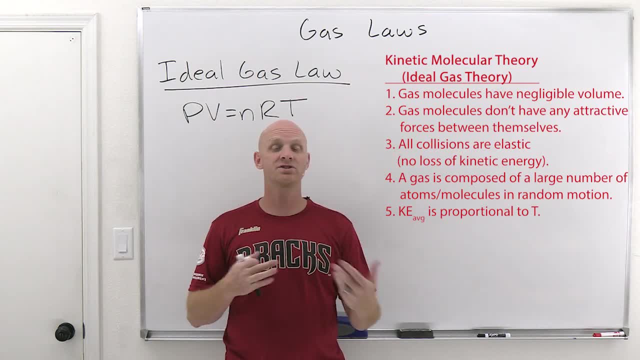 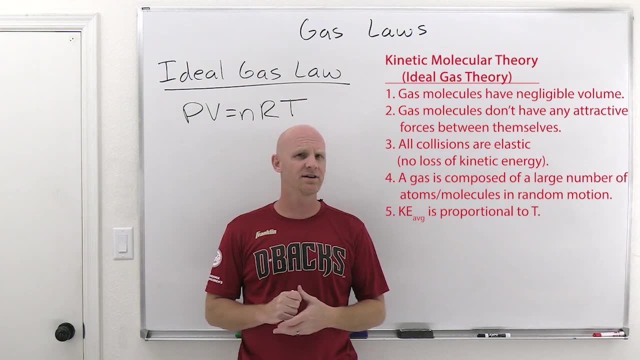 faster. It turns out, kinetic energy and temperature are directly related. As temperature goes up, kinetic energy goes up. molecules are, on average, moving faster, And we'll study this in a little more detail towards the end of this lesson, So, but the idea is that 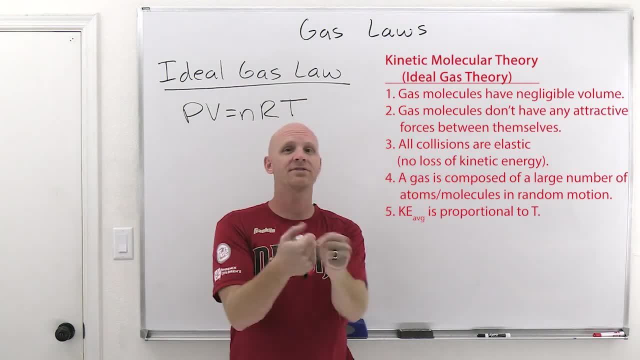 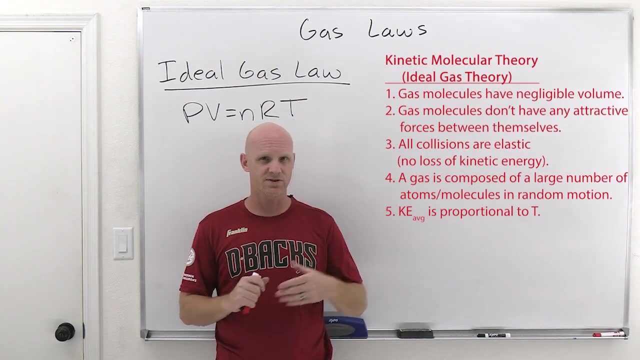 you know, when molecules are moving fast, then they're gonna collide faster too and have less of an opportunity, less time to experience any kind of attractive forces and stuff like this. So imagine having two magnets and I just bring these magnets ever so close together. 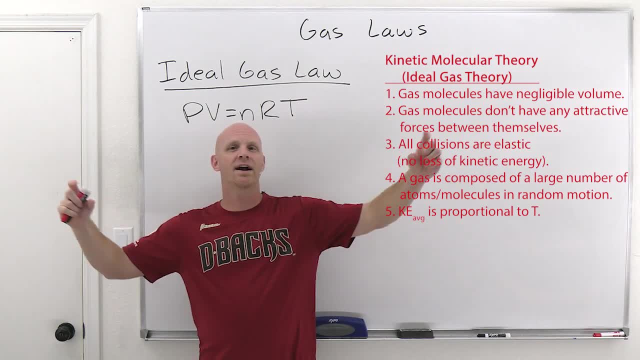 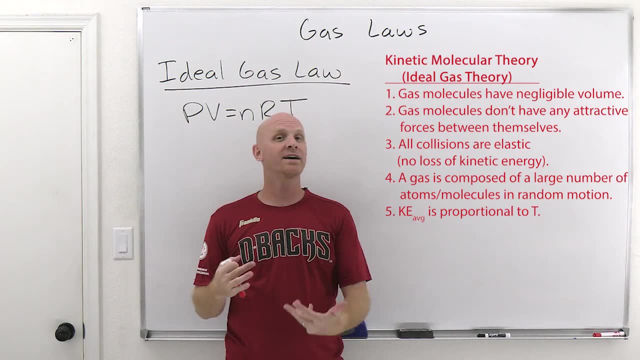 until they stick. Okay, Now imagine instead that I hurl these magnets at each other at 500 miles an hour, right off each other, and the idea is that they had enough kinetic energy to overcome any kind of stickiness they had. Well, the same thing is true. 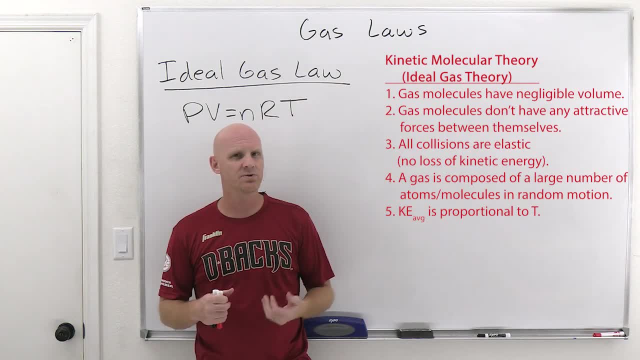 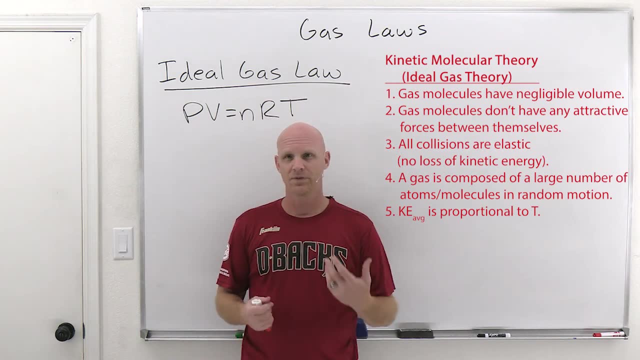 for gas molecules, As long as they're moving fast enough, they're not really gonna get much of an opportunity to feel their attractive forces, even though all molecules at least have a little bit of attractive forces, some more than others. And so the second tenet here. 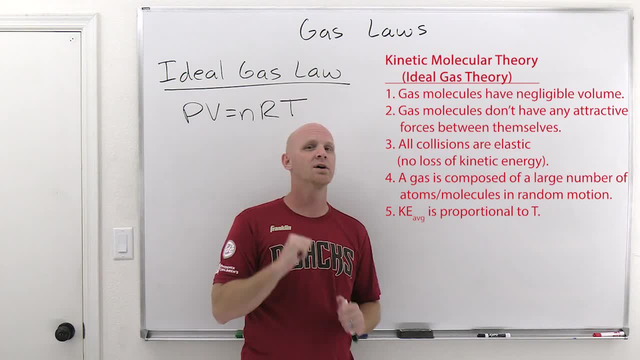 is that there are no attractive forces, and again, never 100% true, but it is most true at high temperatures. The first two postulates of kinetic molecular theory. we understand now why the ideal gas law is most accurate at conditions of low pressure and high temperature. 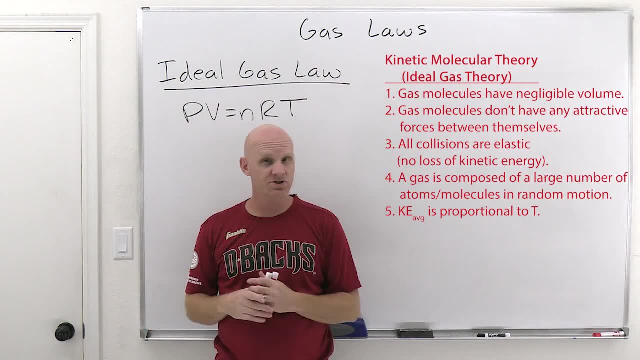 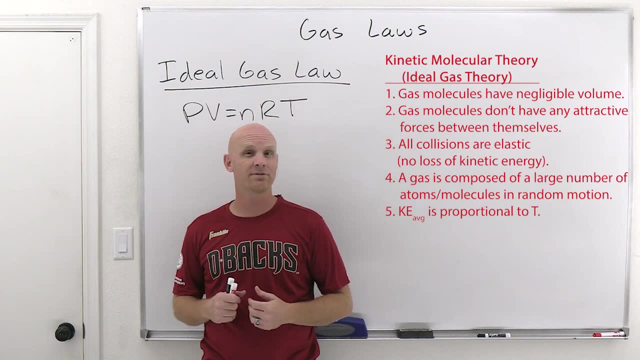 Postulate number one is most accurate a statement at low pressures, when the molecules are really spread out. and then postulate number two here is most accurate: at high temperatures, when the molecules are, on average, moving very fast. All right. Number three postulate, or tenet: 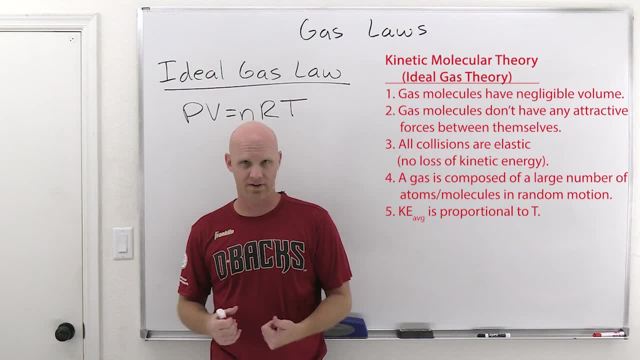 for kinetic molecular theory is that all collisions are elastic. So what that means is that no kinetic energy is lost during collisions. So you know, when the molecules collide with each other or with the walls of the container and stuff like this, we just say: 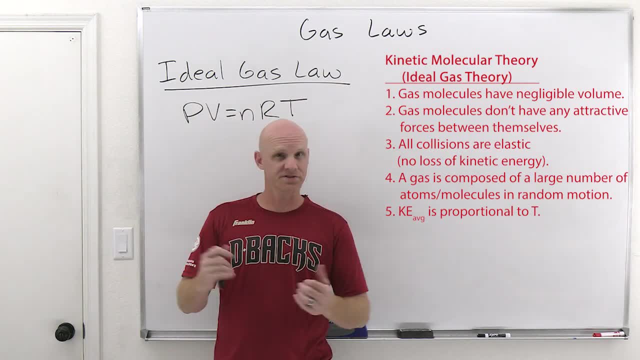 that there is no loss in kinetic energy. So, and that is what actually an elastic collision is- If you have had physics, when you talk about collisions, that is the definition of an elastic collision: one in which no kinetic energy is lost. And the idea is though: 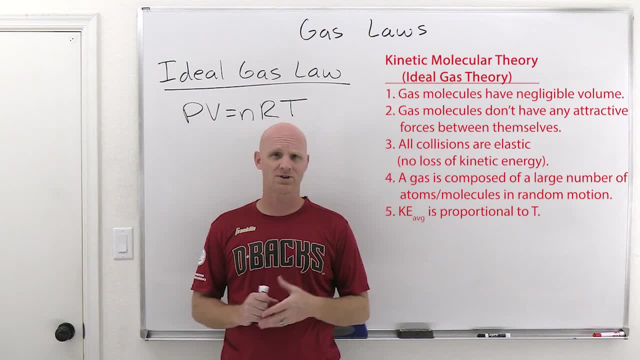 you know, this is really kind of related to the previous postulate in the theory. So an inelastic collision is one in which molecules lose kinetic energy and typically they are losing kinetic energy because they have these two objects that collide, in this case molecules. 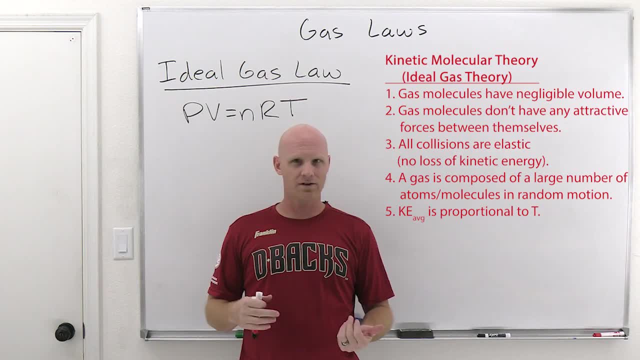 would have some propensity to stick to each other. Well, because we already said that they are not going to stick to each other, they have no attractive forces. that is actually what is kind of guaranteeing that the next postulate here is true, in that there is 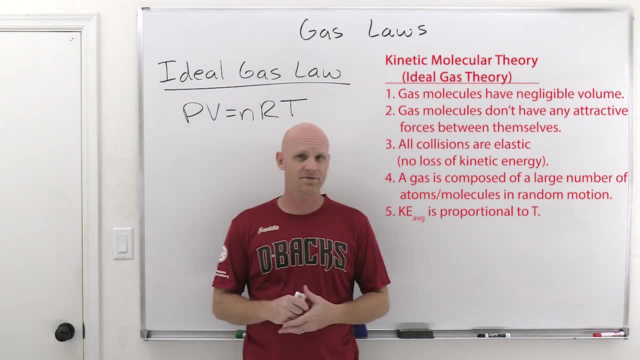 all collisions are elastic and there is no loss of kinetic energy. Finally, we say that, you know, a gas is composed of molecules that are in random motion. That is the last major postulate. We will talk about one minor one here, but postulate. 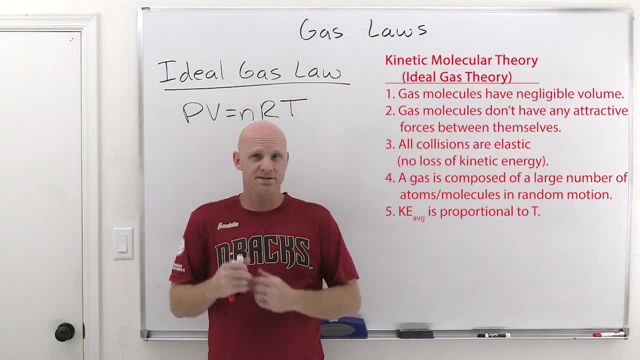 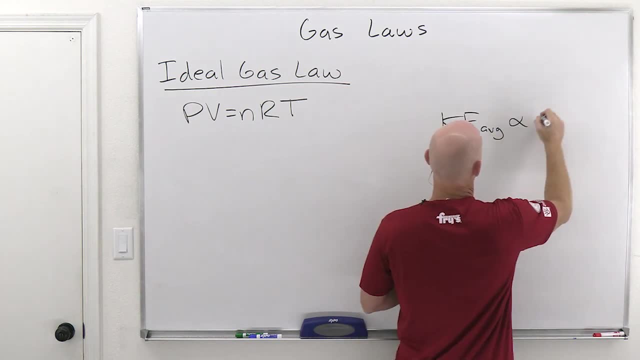 of kinetic molecular theory, and so the last one, though, really is- and this one is a little more minor and some of you guys might not even get this one, so- but it says that the kinetic energy, on average, is proportional to temperature. So it turns out. 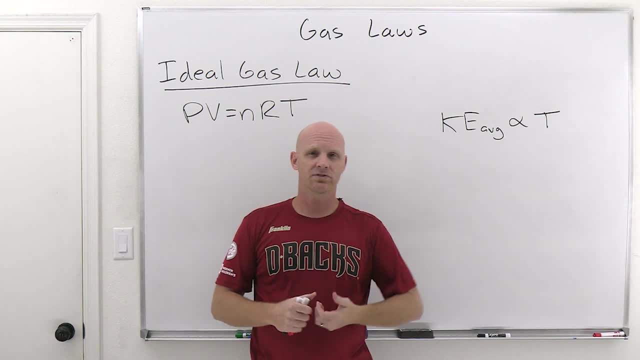 if you double the temperature of a gas, you will actually double its average kinetic energy, and we have to say average, though, because we're moving at the same speed. Some will be faster, some will be slower. What you can say, though, is that, if you double, 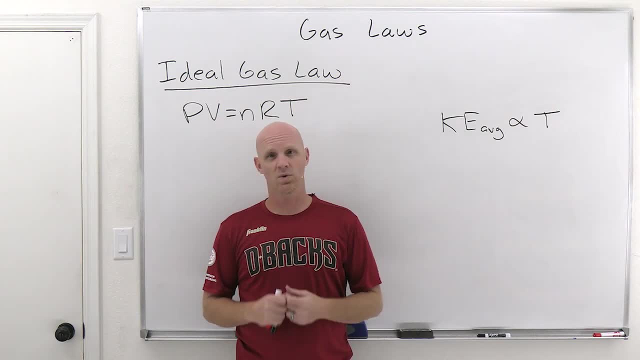 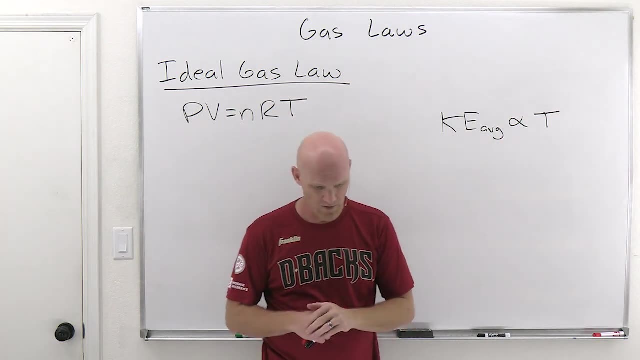 the temperature, then the average speed will double as well, and therefore- I shouldn't say the average speed- the average kinetic energy will double. We'll see what the speed actually does towards the end of this lesson. Okay, so now we know the conditions at which PV equals NRT. 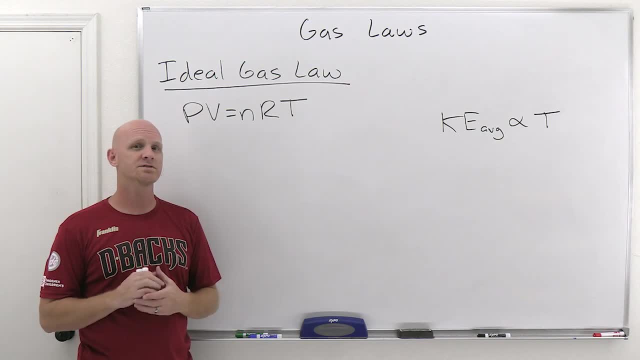 needs to be true. You should know those postulates, memorize them. for kinetic molecular theory The first two are the most important. So again that there are no attractive forces between the molecules, and again those are the ones we use to describe why this lovely. 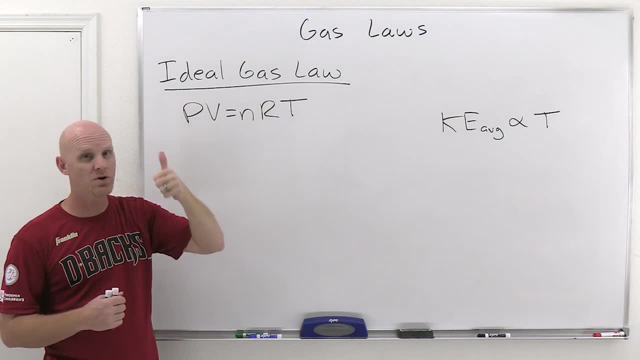 mathematical expression: PV equals NRT. the ideal gas law is most true, again, at low pressures and high temperatures, and you should know that as well. Okay, now actually using this- it's a plug and chug kind of equation here- and a couple things you should know. 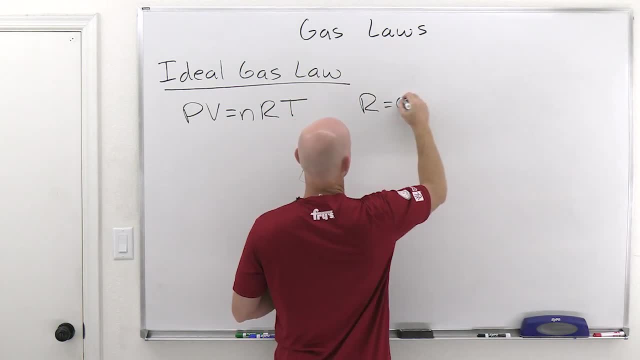 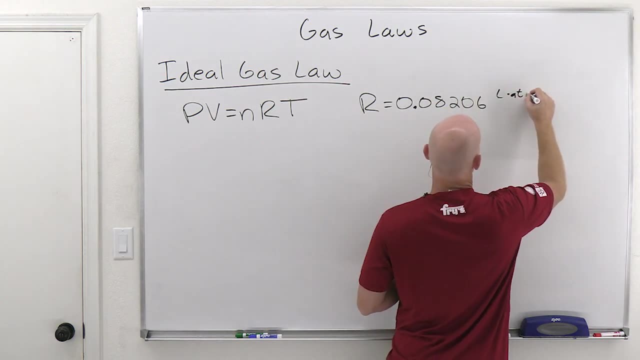 So R here is what we call the universal gas constant, and it has a whole host of values expressed in different units, and you're probably only likely to see it in one of two units, and this is the one we'll be using here. so if you take 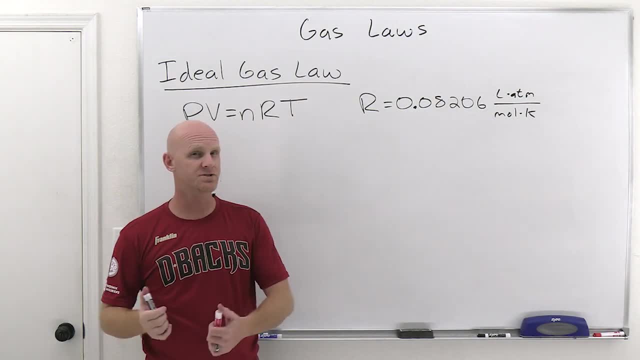 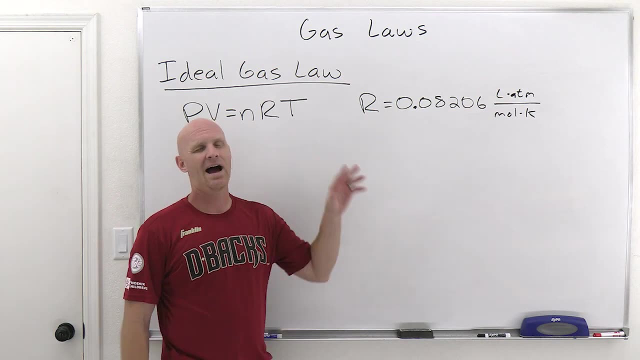 like a more advanced class, though sometimes you'll see it in a general chemistry majors class, but more commonly like a physical chemistry class. they might give you R expressed in like 10 or 12 different units. However, you're likely only going to see it. 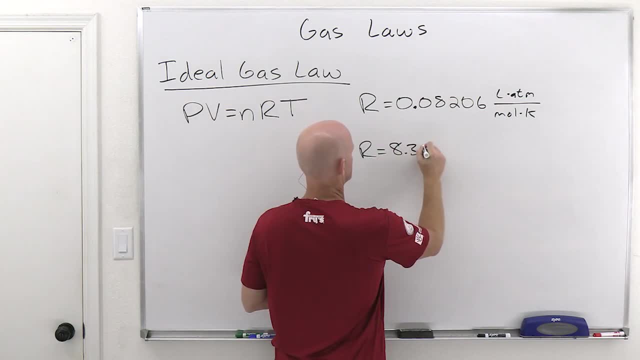 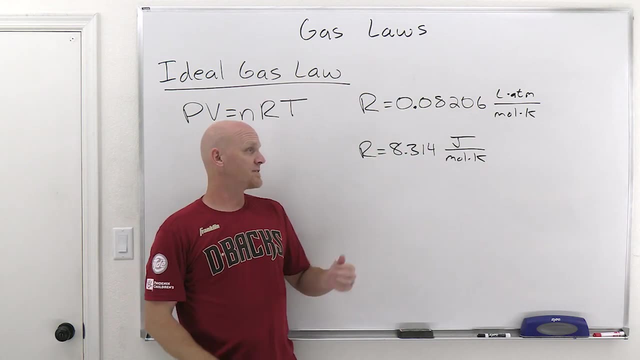 in two, and this is one of them and the other one is this guy. It turns out if you're doing any kind of calculations with pressure and atmospheres and volume and liters kind of stuff, you're probably using this value right here, but this one down here. 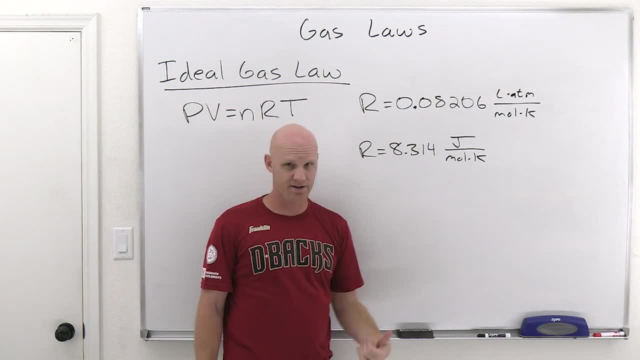 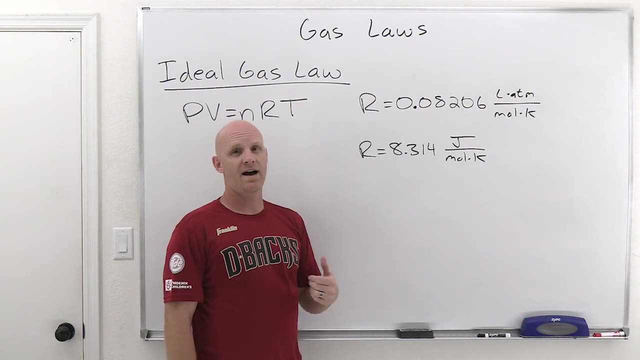 which is in joules per mole Kelvin instead. if you're doing anything in terms of energy, then you're probably using this value instead. Now it turns out, like I said, you might actually be provided in a more advanced class in 10 or 12 different units. 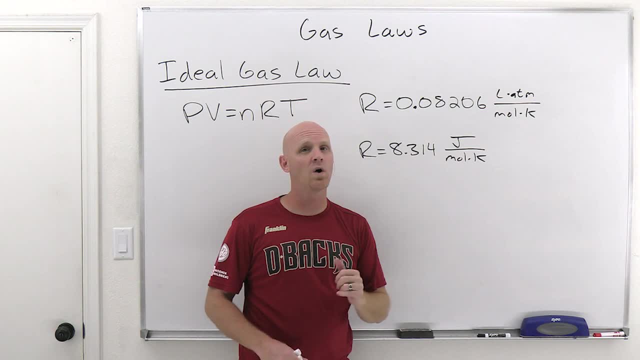 that way, you could, you know, have the pressure expressed in any units you want. You know, instead of atmospheres you can get a version where it's in pascals or kilopascals, or tor, you know, things of a sort and same thing. 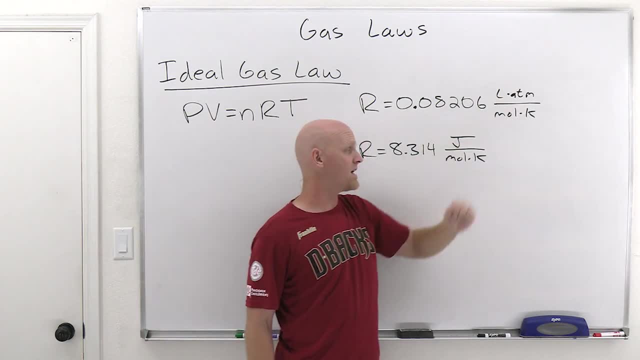 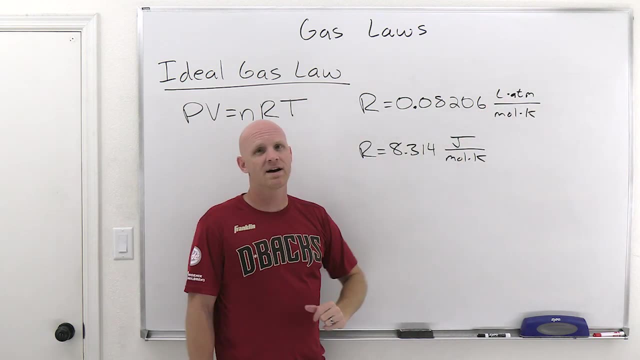 with the volume. instead of liters it might be meters, cubed and stuff. Well, it turns out that liter atmosphere is actually a unit of energy. that combination just like joules a unit of energy. notice the mole Kelvin. your pressure would have to use the SI unit. 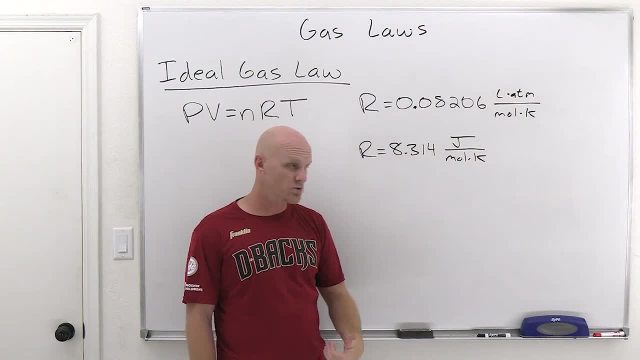 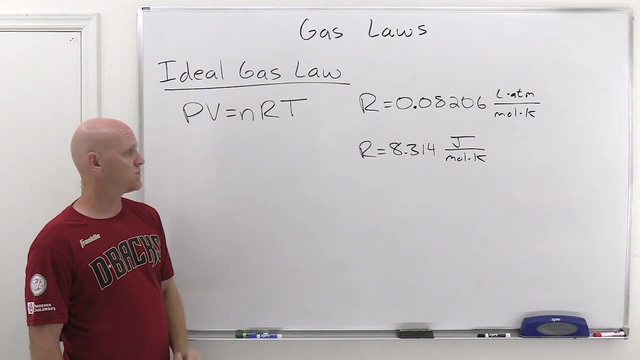 of pascals and your volume would have to use the SI unit of meters, cubed so to use this value, and so what you're going to find, though, is that if you're doing PV equals NRT calculations, students will never use this one here, otherwise. 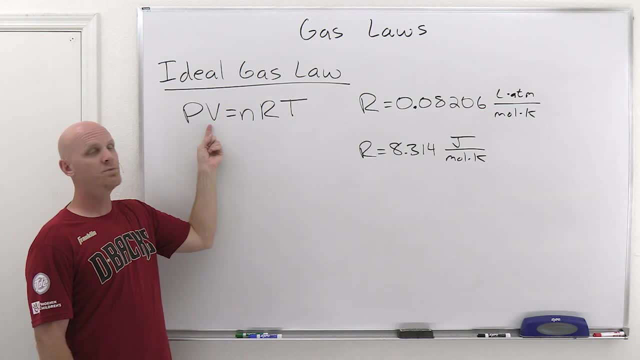 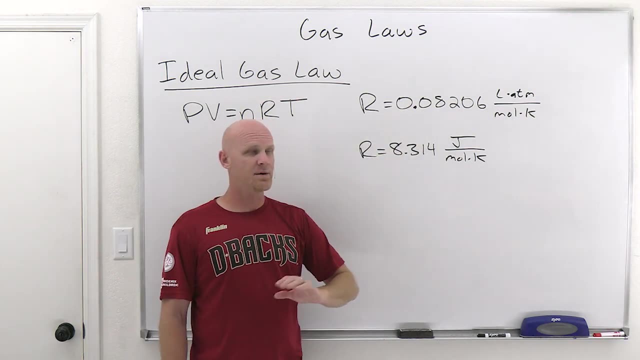 they'd have to remember how to convert, you know, their pressure into pascals and their volume into meters cubed, and they'd have to remember that that's what they even need for this to work, and so they almost never use that one, but this one here. 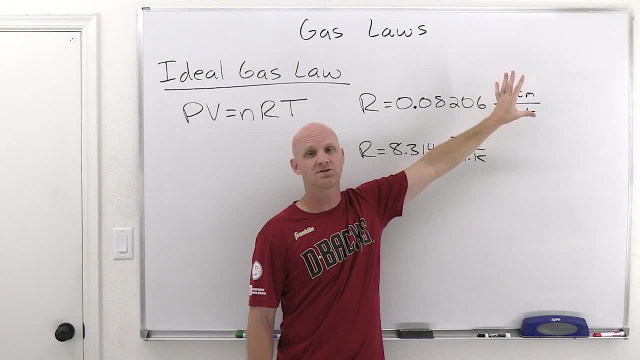 because they know how to get the volume in liters and the pressure in atmospheres. so, and life is good. but this also tells you, then, that if you use this value of the constant, which is most likely one you're going to use, it tells you all the units. 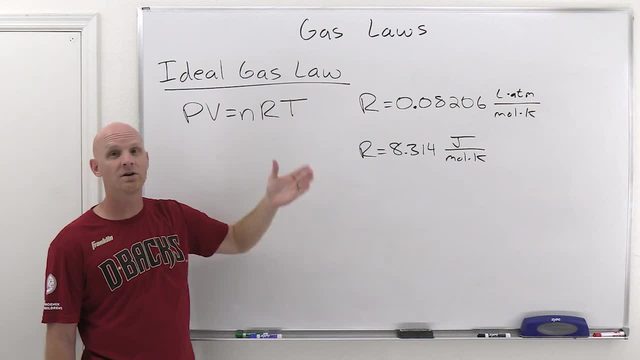 you need. your volumes got to be in liters, your pressures got to be in atmospheres, your temperature has to be in Kelvin. but again, we said temperatures always got to be in Kelvin in this chapter. and then obviously you got moles of gas here. all right, we will use this. 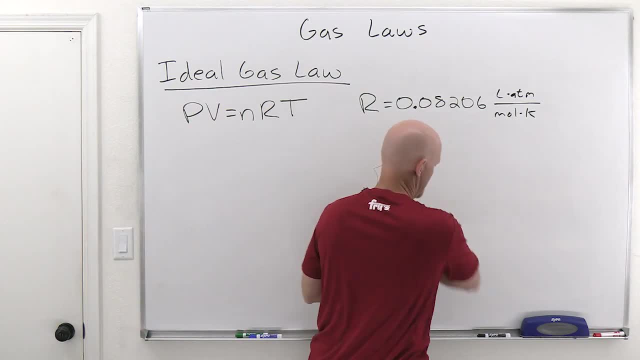 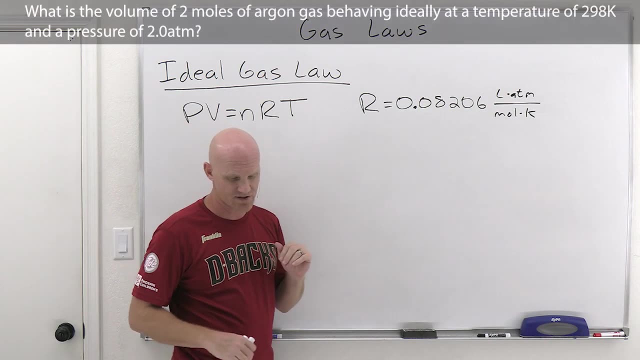 really briefly so, and now we'll just take a look at a couple of different calculations you might see using the ideal gas law here, and so question here on your on. the study guide says: what is the volume of two moles of argon gas behaving ideally? 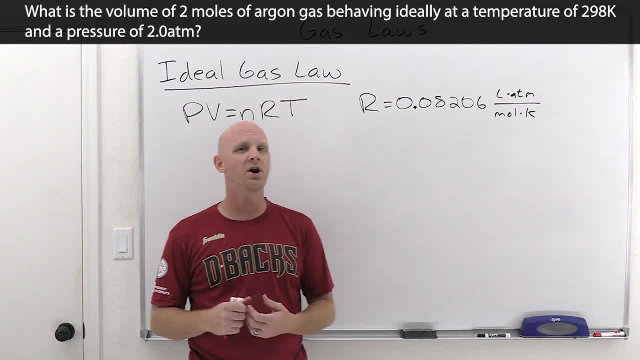 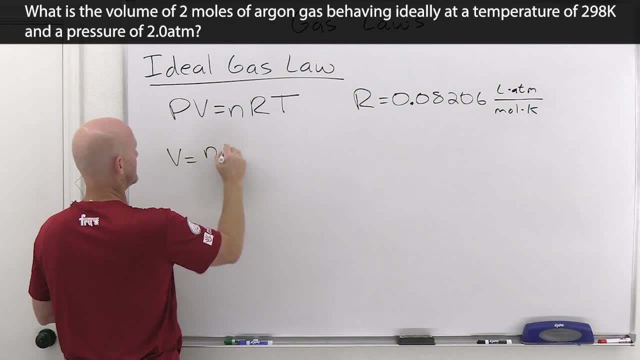 at a temperature of 298 Kelvin and a pressure of 2.0 atmospheres. so in this case we're solving for volume. so I'm just going to rearrange the expression here to solve for volume and we'll get. volume equals nRT over P. 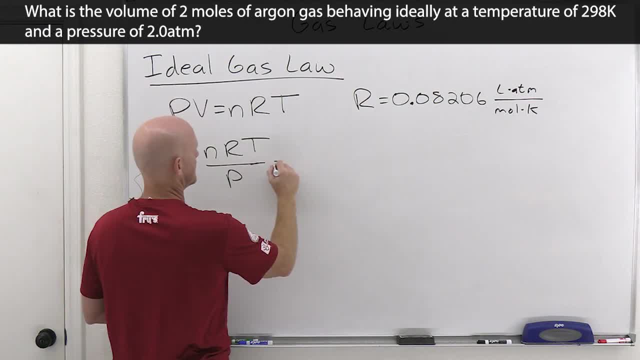 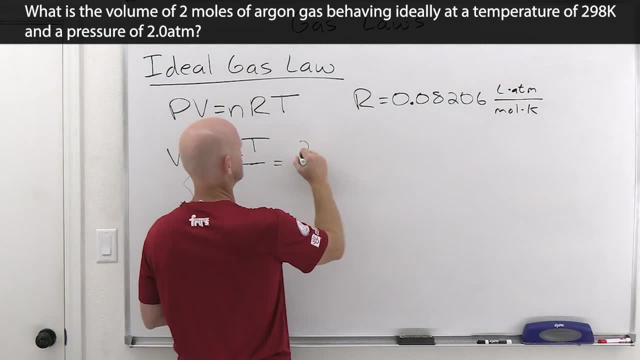 and just brought P over here and divided through. so in this case we were given everything we need in the units we need them. so we're told that it's two moles of argon gas and so in this case it didn't matter that it was argon at all. 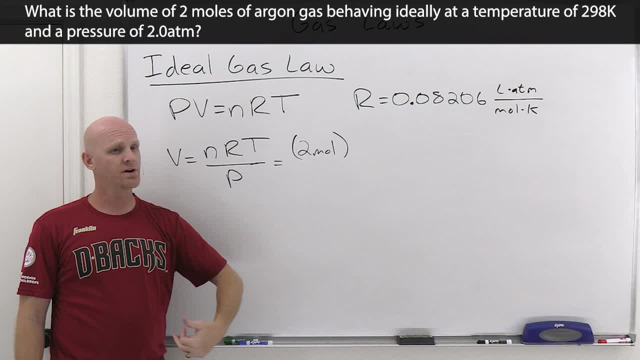 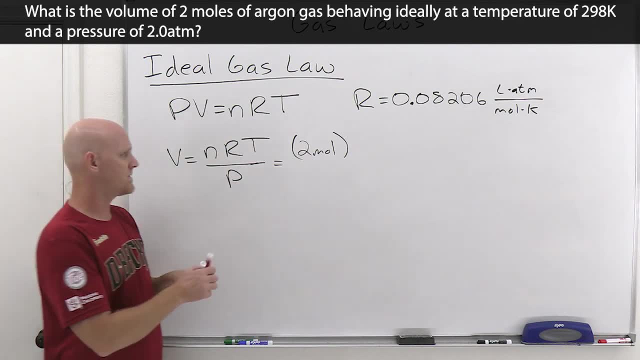 so the equation just calls for the number of moles of gas. whether it's argon or carbon dioxide or nitrogen or oxygen, it does not matter. it just needs whatever the number of moles of gas is. so then we'll plug in R here. sometimes you'll see, 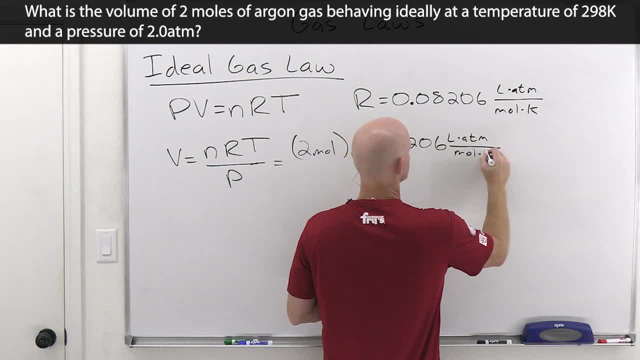 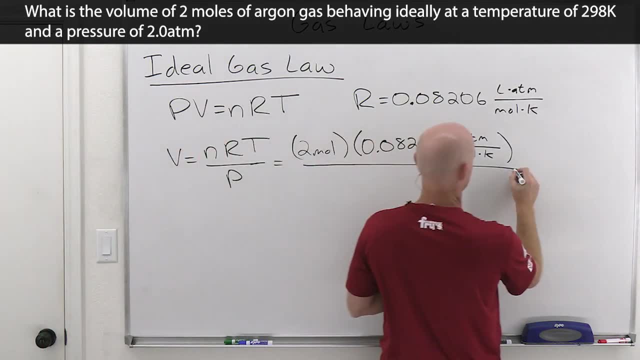 all the different ones because they're all the same, but I do want to make sure that you look at both so you can see that when you look at the difference in the temperature in the atmosphere, the temperature is at the same as the temperature in the atmosphere. 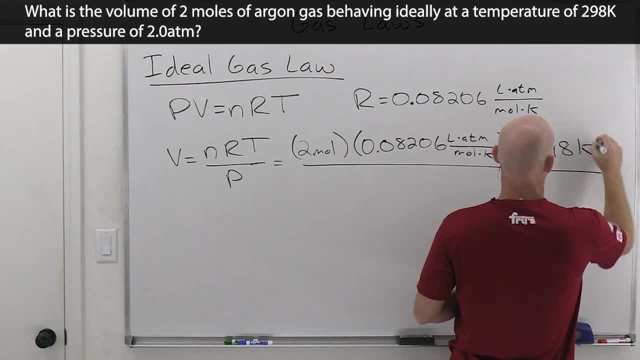 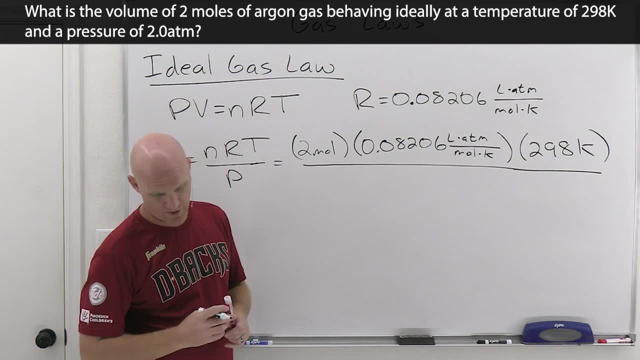 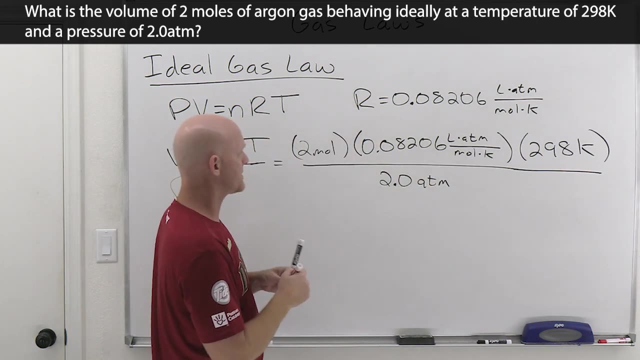 so in this case we're being told that it's at a temperature of 2.0 atmospheres. so we're thinking we could multiply that by a certain number of moles and that also gives us what the pressure is and we can see Cool, and you can see all your units are going to work out here. 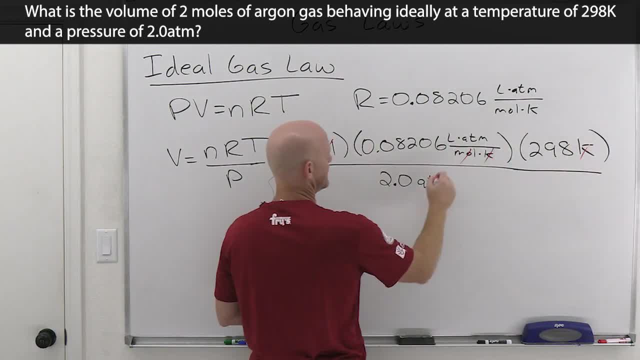 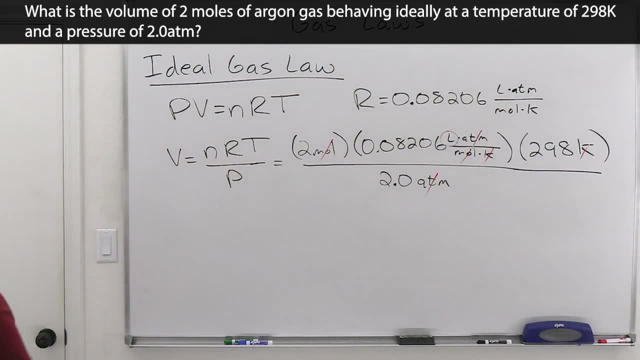 The moles here is going to cancel, the Kelvin here is going to cancel, the atmospheres here is going to cancel, and our volume is going to come out in liters. and let me grab my calculator, All right. so let's do some plugging and chugging here. 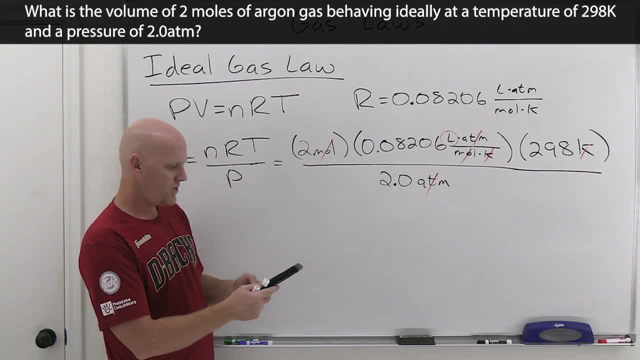 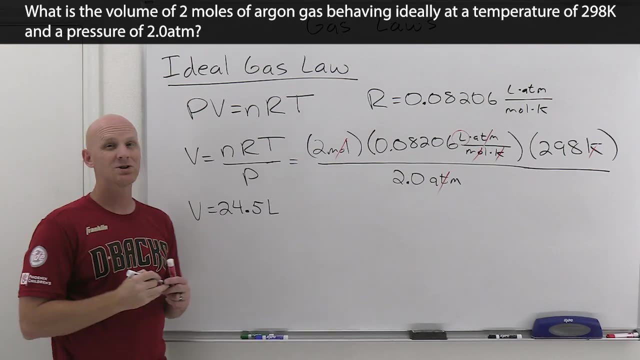 In fact the twos will cancel. so really we just got to do 0.08206 times 298, and we're going to get 24.5 liters. That is not in proper scientific notation and I don't care. 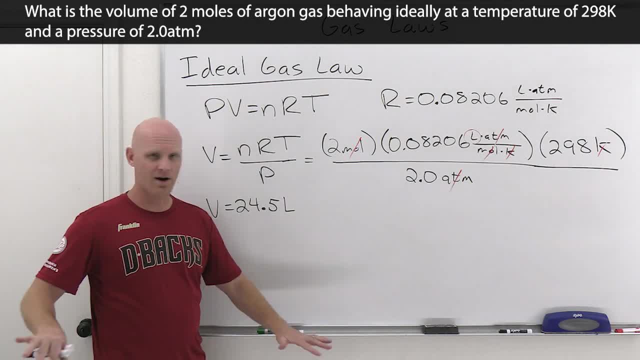 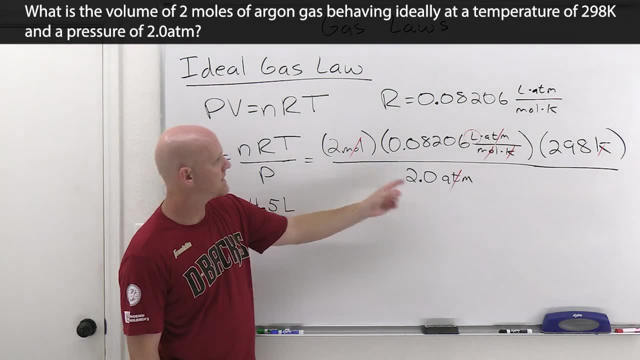 Not worried about scientific notation. it's not in proper sig figs and I don't care- Not worried about sig figs in this particular lesson. so I really should have rounded this probably down to 24, because it was really 24.45, and I really got. Actually, I maybe. 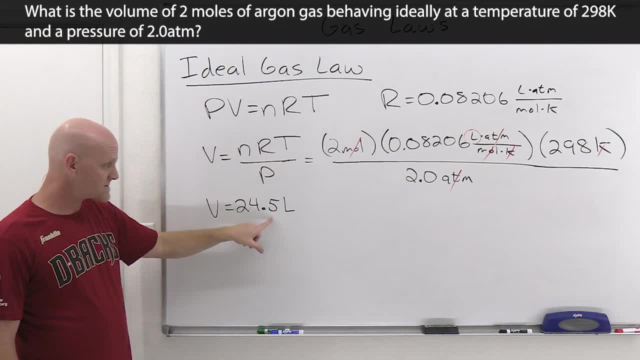 have to get down to one sig fig, and I don't really want to do that. so I'm just going to keep a decimal place and not worry about sig figs, All right, So that's the answer to this question. It was fairly straightforward. 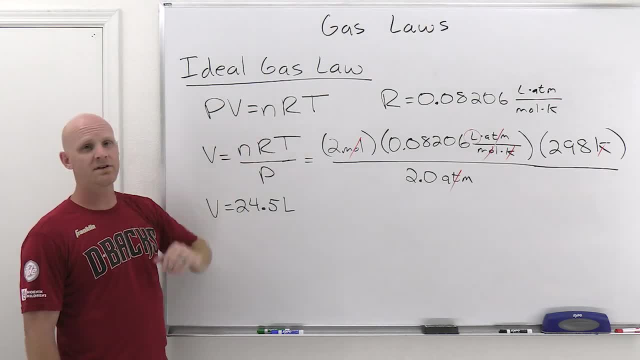 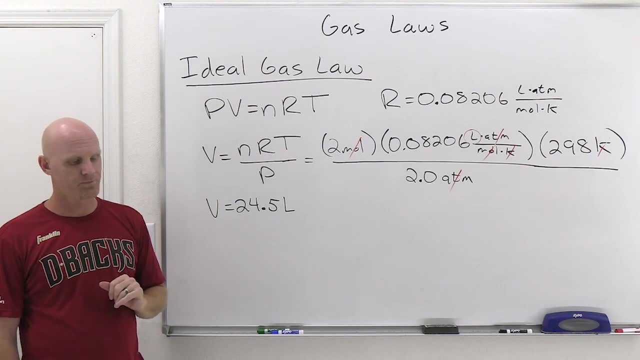 There are four variables in this equation and one constant, and out of those four variables, I gave you three, You plug them in, you solve for the one you don't know. Life is good. However, we can make this harder, and that's what I do in the next question. 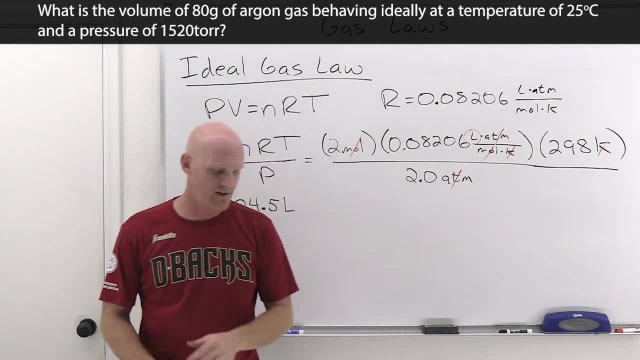 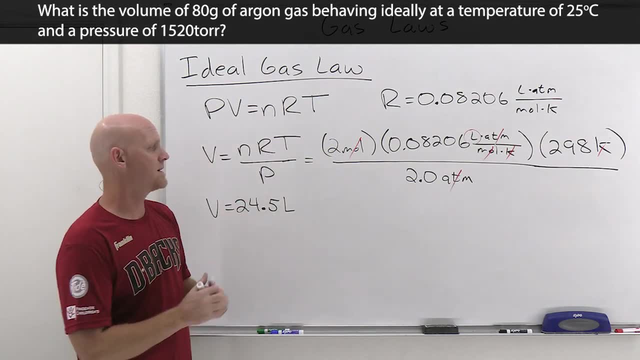 The question says: what is the volume of 80 grams of argon gas, behaving ideally at a temperature of 25 degrees Celsius and a pressure of 1,520 Torr? What makes this more difficult is that you're told that it's 80 grams. 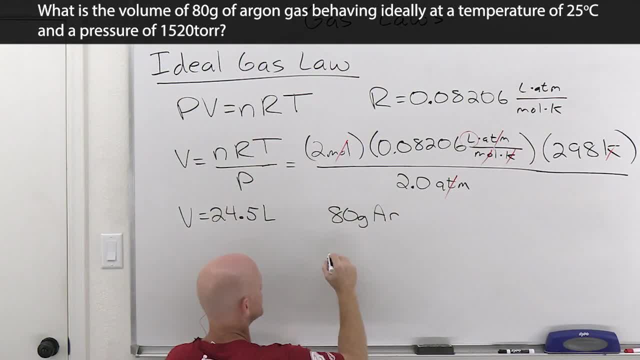 80 grams of argon gas, You're told that it's a temperature of 25 degrees Celsius and you're told that it's a pressure of 1,520 Torr, and the problem is, none of these are actually expressed in a way in which it will get plugged into that equation. 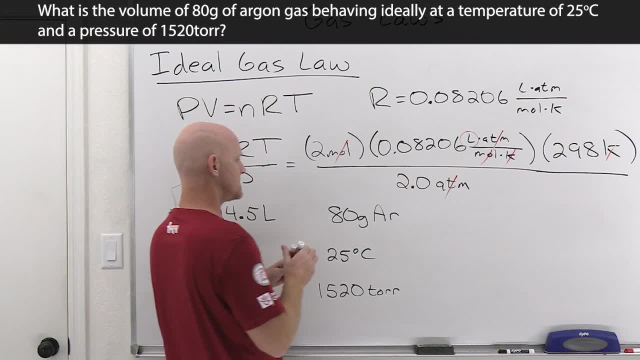 I don't need the mass of a gas, I need the moles of gas, and so you'd have to do a conversion here, right? So 80 grams of argon gas. you look it up on the periodic table and it turns out that 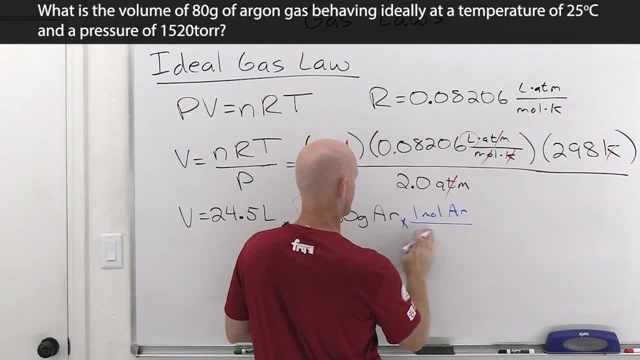 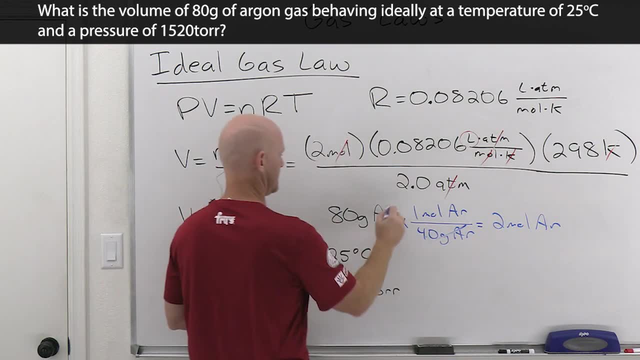 one mole of argon weighs- Not that It weighs 40 grams, and we'd find out that we've got two moles of argon. Great, Just like a minute ago, we're provided that we had two moles of argon. 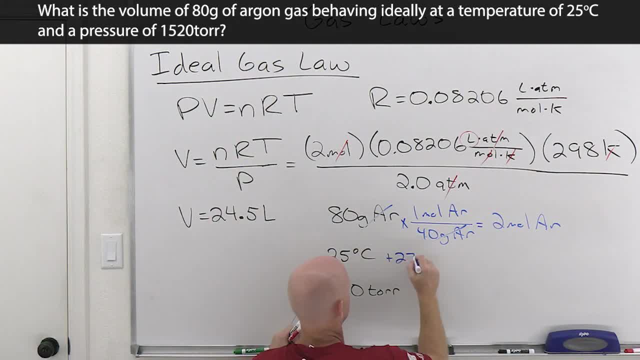 So 25 degrees Celsius. we just need to simply add 273 to find out that we're at 298 Kelvin, just like we had 298 Kelvin in the calculation above. Finally, 1,520 Torr. we want to convert that to atmospheres to plug it in again, all based. 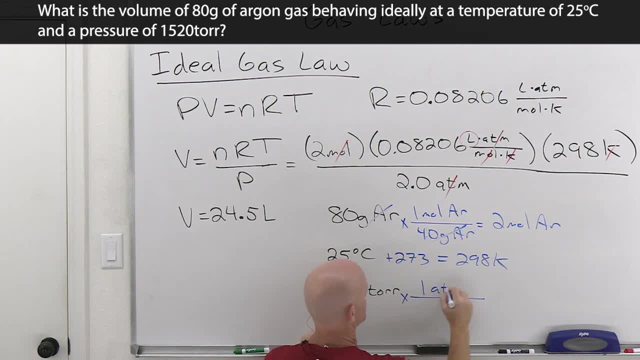 on the units of R, and one atmosphere equals 760 Torr, and we'll find out that we're at a pressure of two atmospheres In this case. we had to do a conversion for all three of these before we got them into. 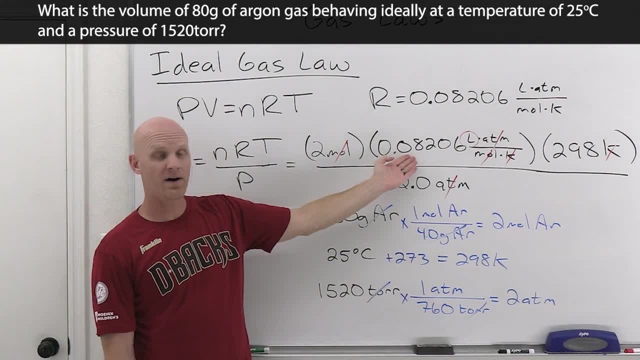 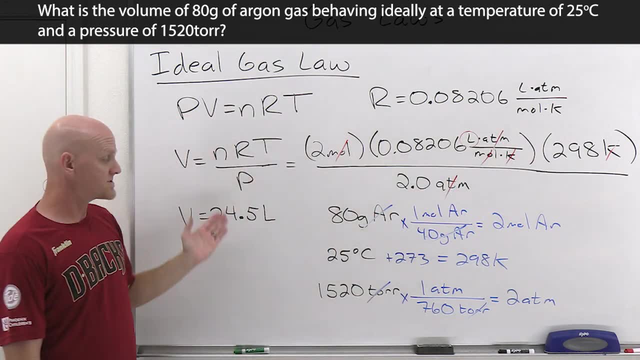 the units required for plugging them in here, based on the value of that universal gas constant we're using. But notice, all these came out to the same values we had just a second ago, and so if you solve for volume, you're still going to get this 24.5 L. 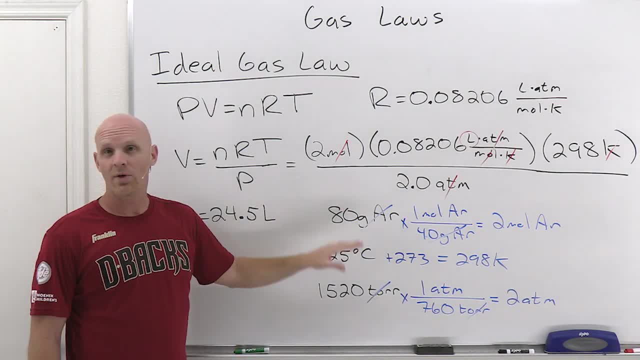 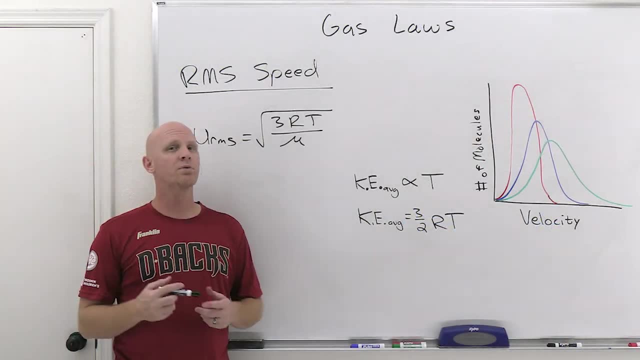 All right, So be prepared for it to be a little more challenging and have to do some conversions more than likely on a typical exam question. All right, So now we're going to really briefly talk about RMS speed, That's root, mean square speed. 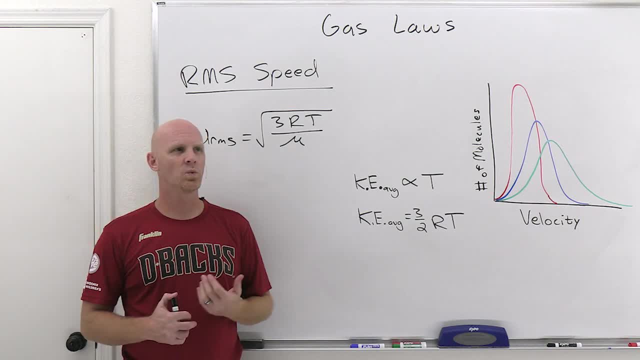 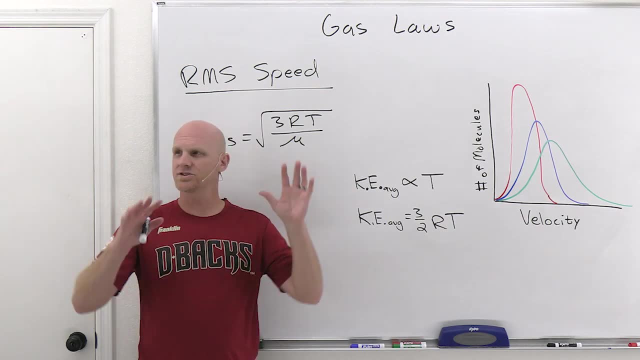 So you typically talk about something that's a root mean square, when there's actually no overall value for that particular quantity because it's going in all directions. So in this case, like in this room right now, the gas molecules in the air they have just 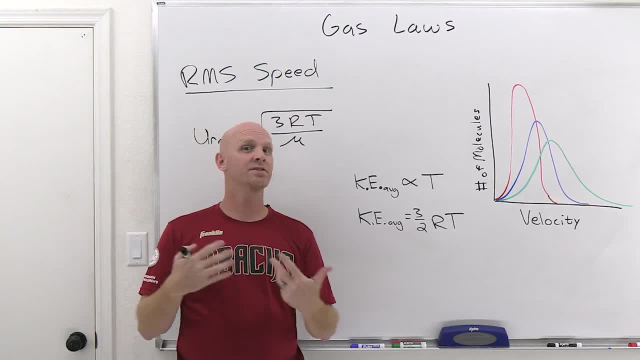 as high a likelihood of moving in any position. They're moving in any particular direction and there's no net movement, you know, flow of air in this room And so, as a result, the average velocity, if we actually, you know, calculated it and 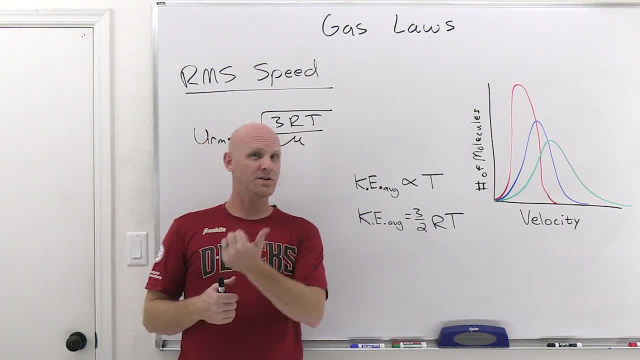 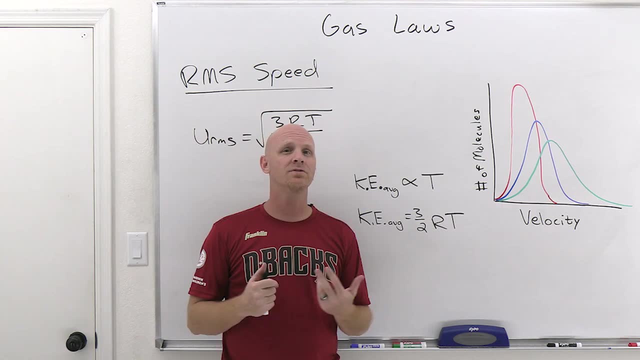 tabulated it, for all the molecules would be zero, because you know anything moving to the left would cancel out. you know things moving to the right if they're at equal magnitude and stuff. And so you find out, lo and behold, that the average velocity is zero. but that's not a. 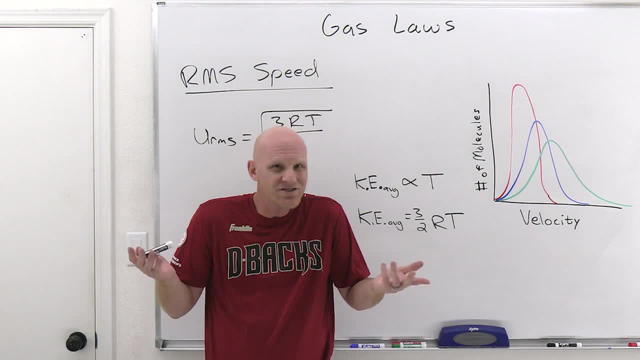 very informative number because I want to know, like, what speed, like how fast are the molecules in this room actually traveling around? I mean they're bouncing into each other and stuff, and I realize I'm bouncing off the walls and stuff. 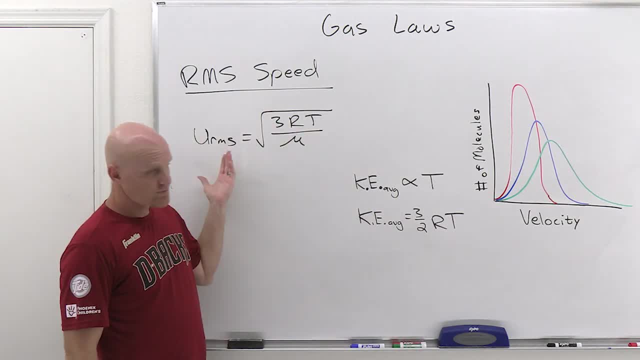 How are they really moving? So, and that's what root mean square speed will allow us to do in this case. So it's kind of like an average. It's not the same thing by any stretch, but it's kind of like an average when you don't. 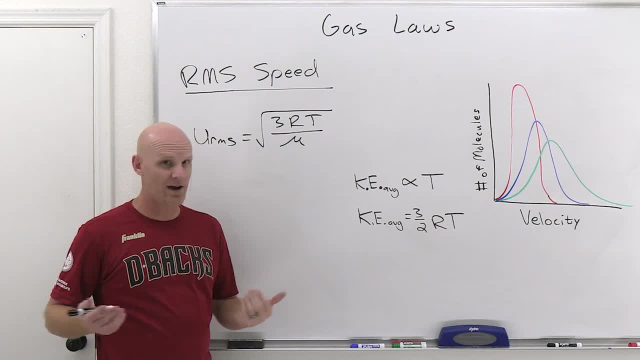 want direction to kind of make you know, to result in all of them canceling out and giving you a value of zero for something like this. So in this case, it turns out we have a lovely formula for this and we'll derive that real. 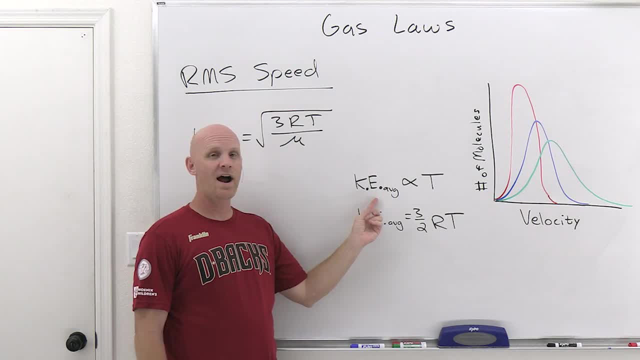 quick. We said with kinetic molecular theory that the kinetic energy on average was proportional to temperature. So If you look back up on your study guide, I actually gave you this expression right here. So it turns out for a monatomic ideal gas here. 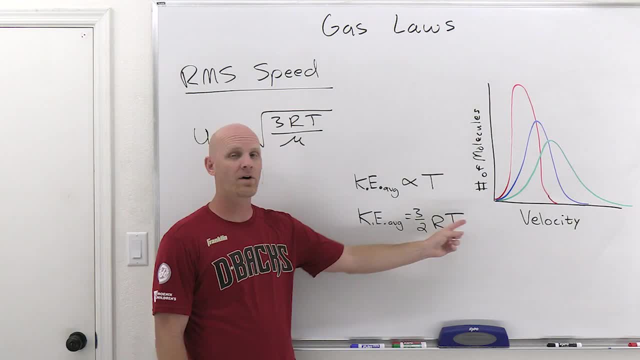 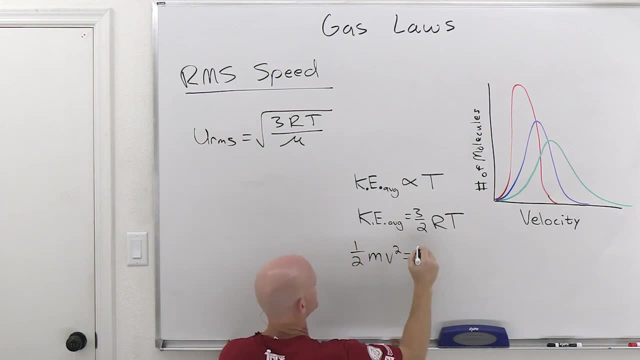 So your kinetic energy, your average kinetic energy, actually equals three halves RT. And if you've taken a physics class, you know that kinetic energy is one half mass times velocity squared. So in this case that's going to equal three halves RT. 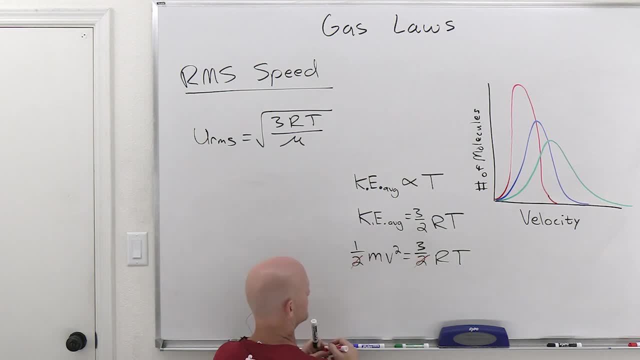 And so we can get rid of a couple of things here. Here's the halves part we'll get rid of, And so we'd get V squared. We solve for V squared: Move the M over. It's going to equal three RT over M, And then we just take the square root of both. 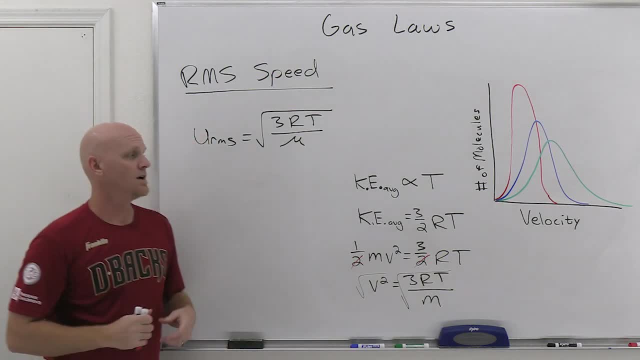 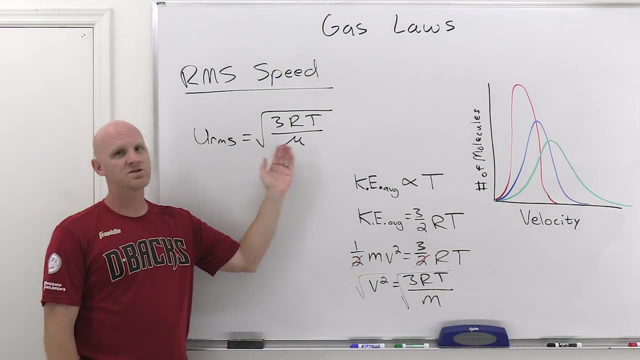 sides, and you find your velocity would equal the square root of three RT over M. Well, instead of velocity, here again we're actually using root mean, square speed. U here is going to stand for speed, but you can kind of see where this equation comes. 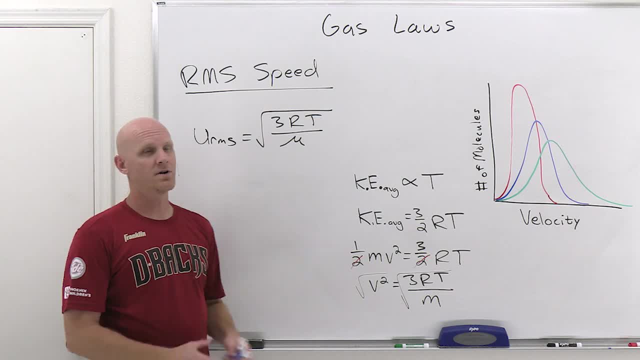 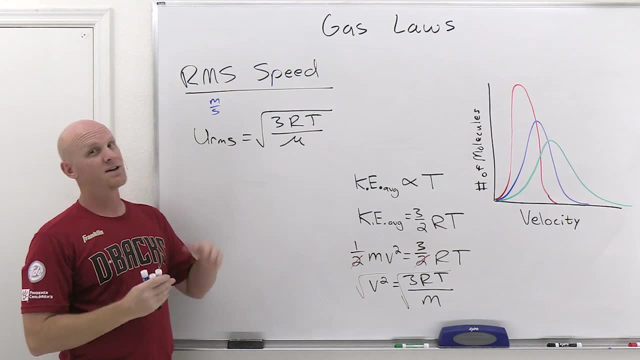 from A couple of things. we really got to be careful here, though, is that if we're trying to get root mean square speed, well, the SI unit for speed is the meter per second, And if we're trying to get this to come out in SI units, 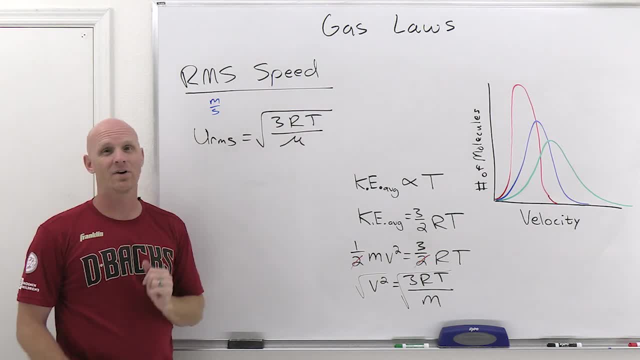 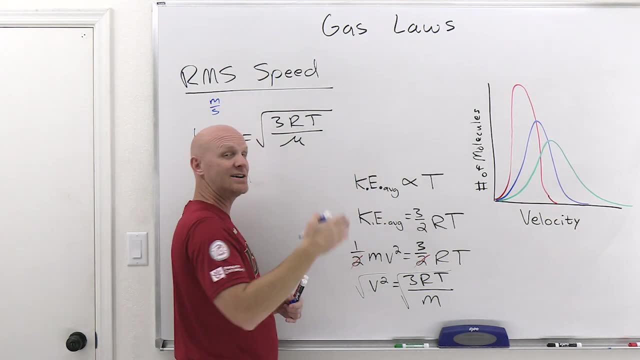 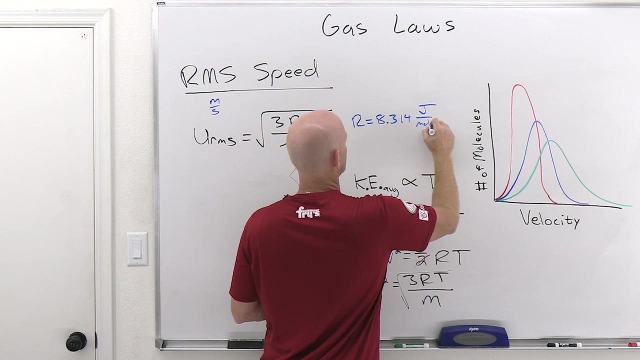 Well then, we better make sure we're using SI units for the entire calculation, And that sucks. This is the one place in this chapter where, instead of the 0.08206 liter atmospheres per mole kelvin value of R, you're going to preferentially use the 8.314 joules per mole kelvin, because, 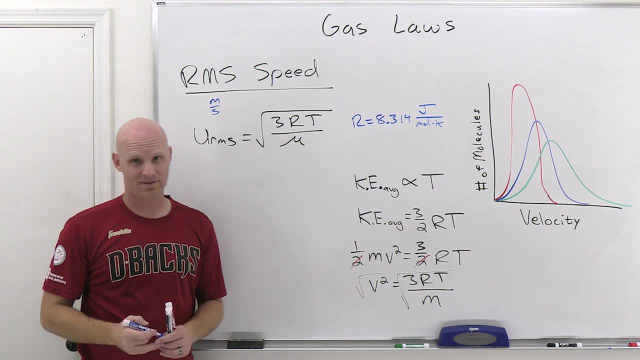 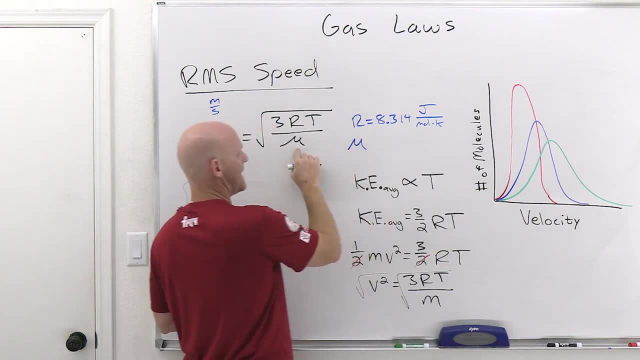 the joule is the SI, is R expressed in SI units, whereas the liter atmosphere is definitely not SI. So one more thing here is that your molar mass, Molar mass here is what mu stands for, and that molar mass has to be in SI units as well. 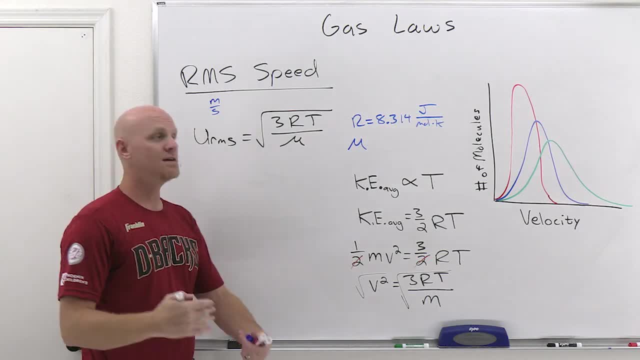 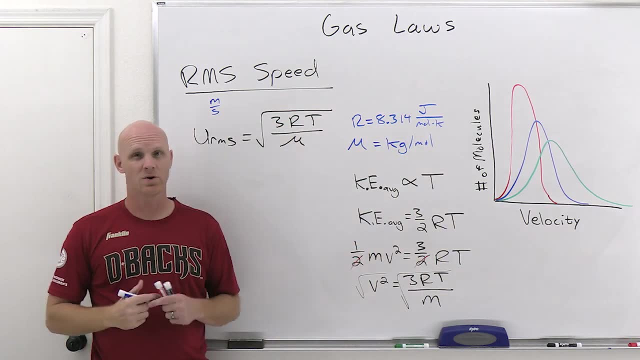 And the SI unit for mass is not the gram, It's the kilogram, And so you're going to want to express that not in grams per mole, but kilograms per mole instead. So got to remember both of those things. You got to use the proper value of R and get your molar mass in kilograms per mole rather. 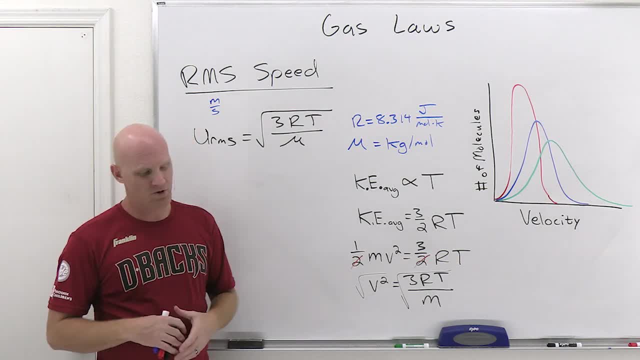 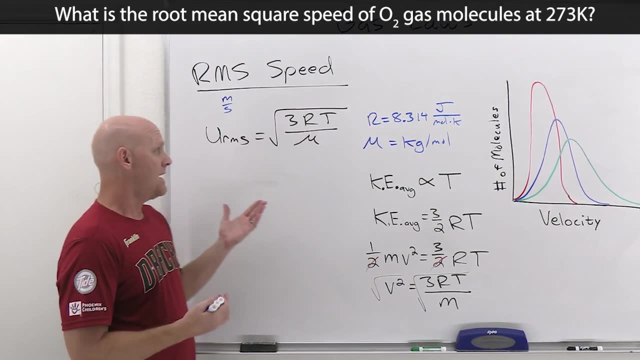 than grams per mole. After that, though, you'll be good to go, So the question we're going to take a look at here is: what is the root mean square speed of O2 gas molecules at 273 kelvin, And in this case, it's just going to be a plug and chug kind of situation here. 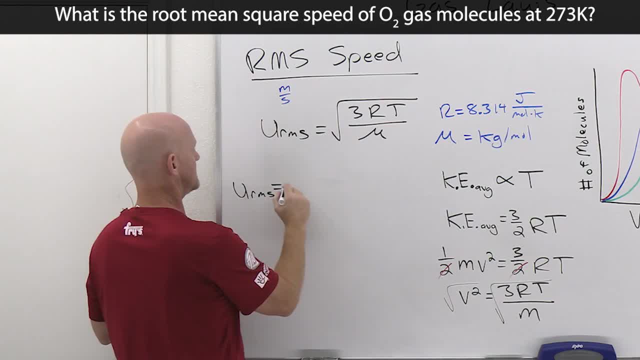 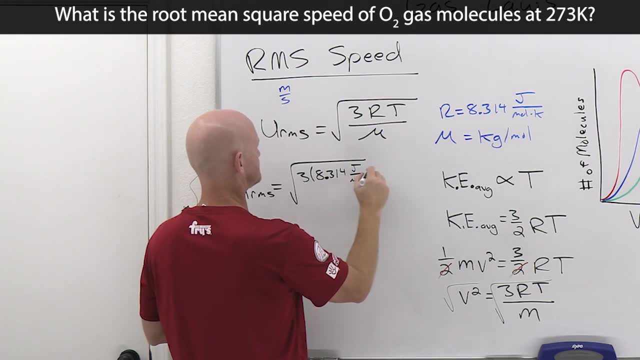 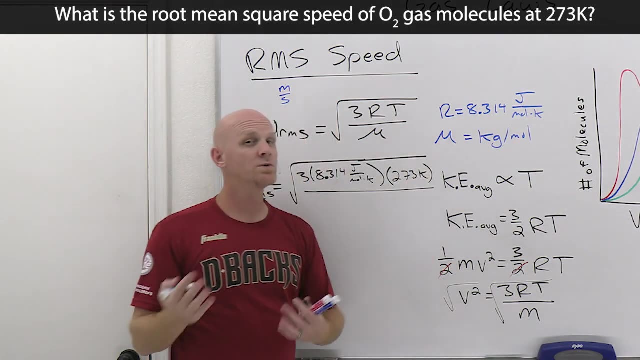 And so we're going to get our RMS speed. It's going to equal square root of 3 times 8.314 joules per mole, kelvin times temperature of 273 kelvin all over the molar mass. Well, again for O2, for oxygen, the molar mass, just O, is 16 grams per mole. 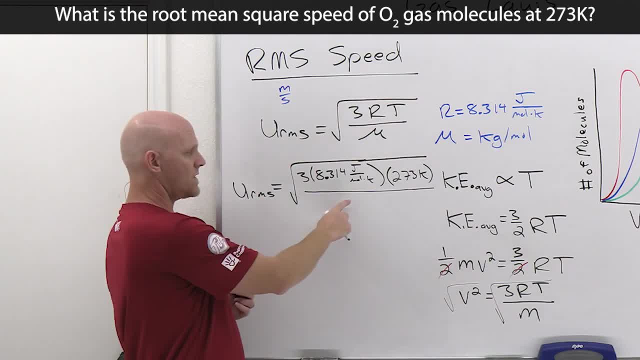 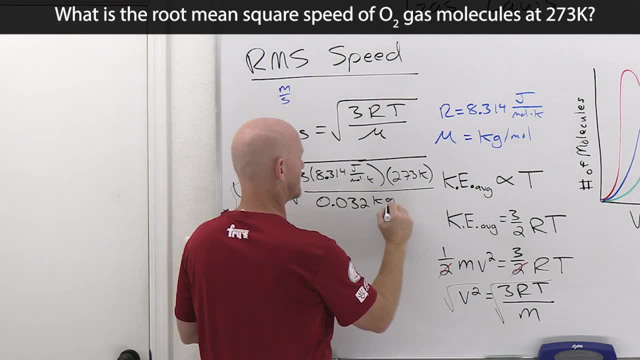 But for O2, it's going to be 32 grams per mole. But I don't want grams per mole, I want kilograms. So instead of 32 grams per mole, it's going to be 0.032 divided by 1,000 kilograms per. 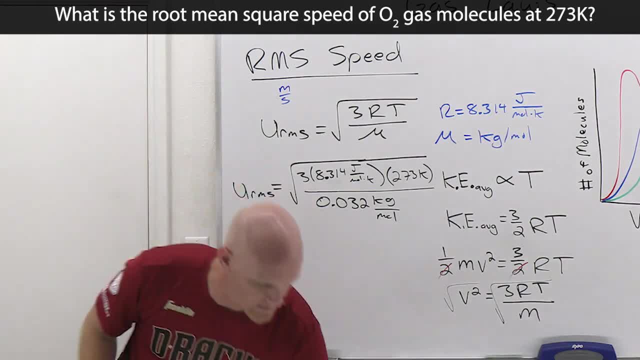 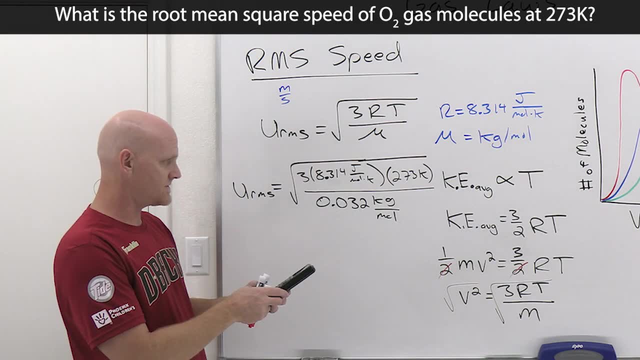 mole, And from here then it's just plug and chug. So we're going to take 3 times 8.314 times 273, divided by 0.032.. And then I'm going to take the square roots of that answer and get 461 meters per second. 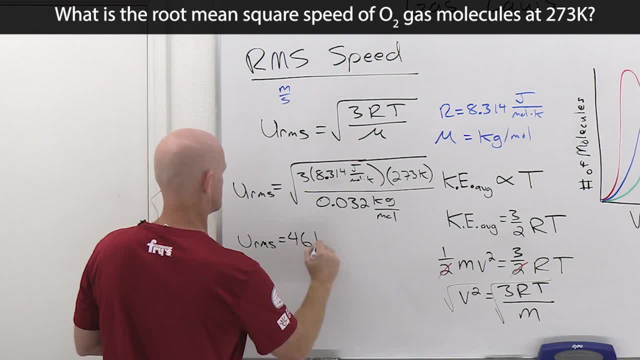 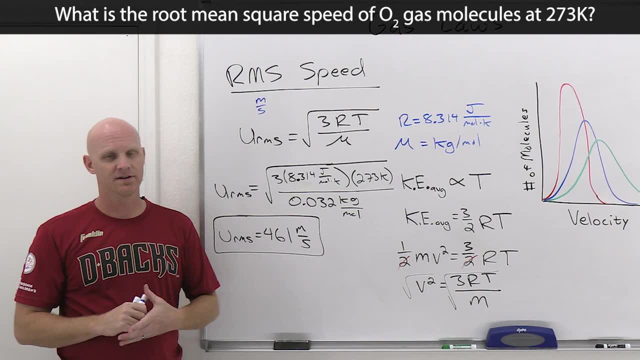 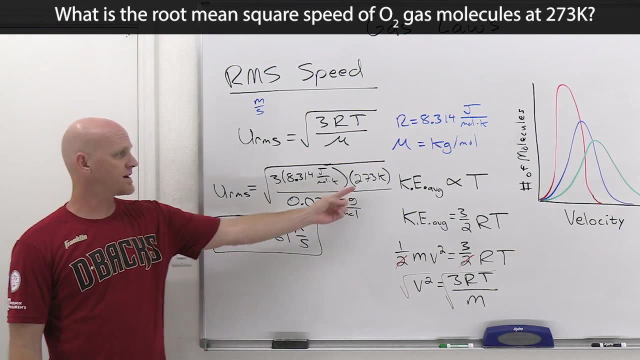 So that's rather fast, The average speed, if you will, and again it's not really an average. The root mean square speed of one of the O2 molecules in this room would be a little faster than this, because we're not at 273 kelvin. 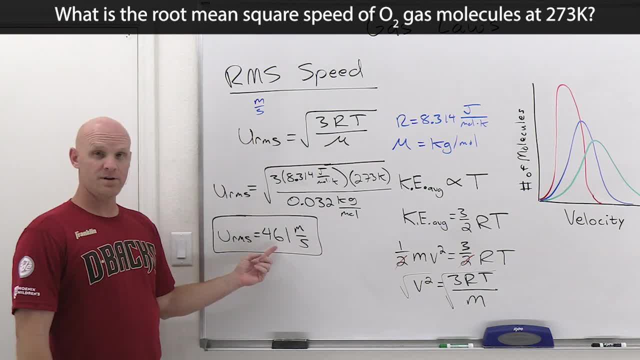 We're at 298 kelvin-ish in this room And so, but it's going to be on the order of this, though just a little bit faster than this. That's actually rather fast if you think about it, Cool. 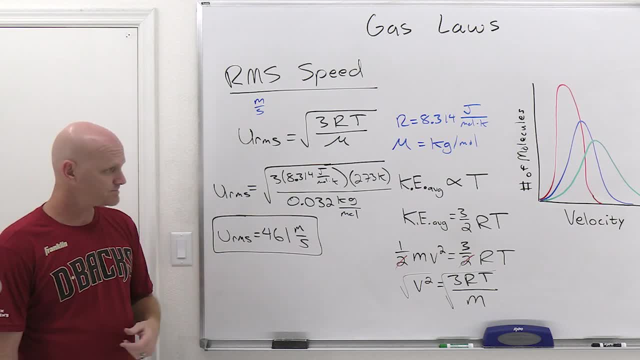 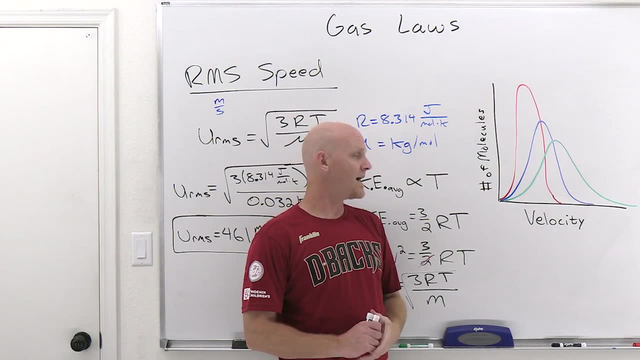 And that's root mean square speed. So yeah, You know faster than you'd think. Now one last thing I want to talk about here, with root mean square speed. here is this lovely diagram here which gives you the Maxwell distribution of speeds. 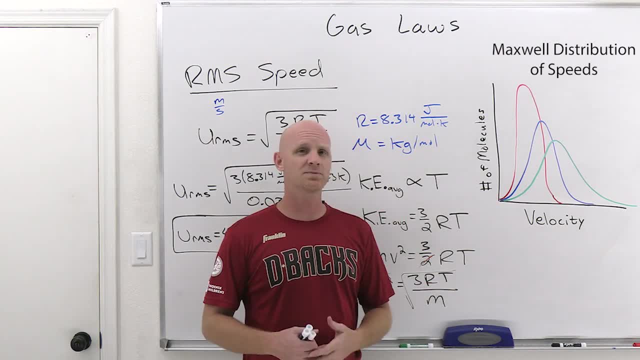 And we've said we have to talk about, you know, average kinetic energy and stuff like this, because not all molecules are moving at the same speed or velocity. Well, in this case, this gives you a graph of kind of what it looks like. 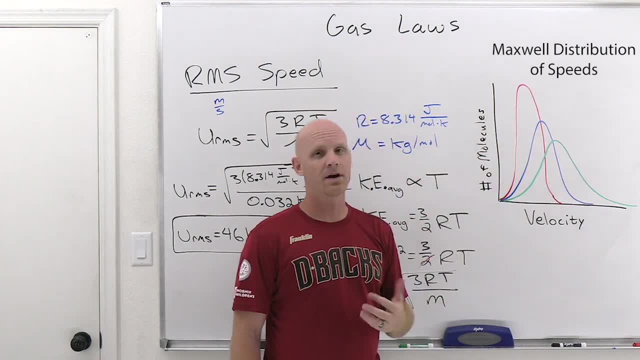 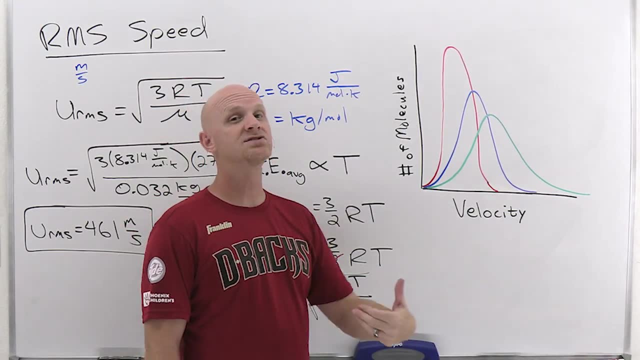 And so here I've got- actually, you know, three different graphs on here. I'm going to focus on one of them for a second, And so let's just focus on the red, And that's going to be the Maxwell distribution of speeds for a gas at a particular, you know, particular gas. 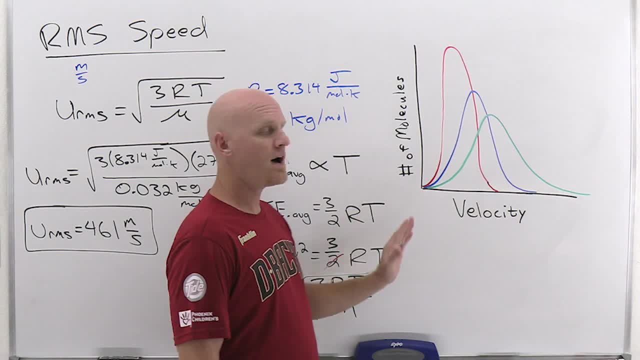 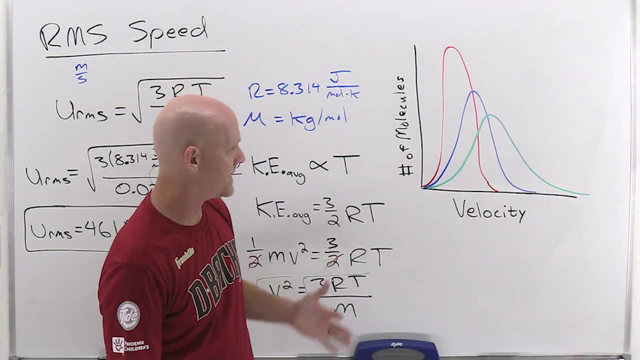 at a particular temperature And what you'll find is that you know they're not all moving at the same velocity. but there is this nice, lovely, looks like fairly Gaussian distribution. It turns out it's not perfectly Gaussian, but looks that way. 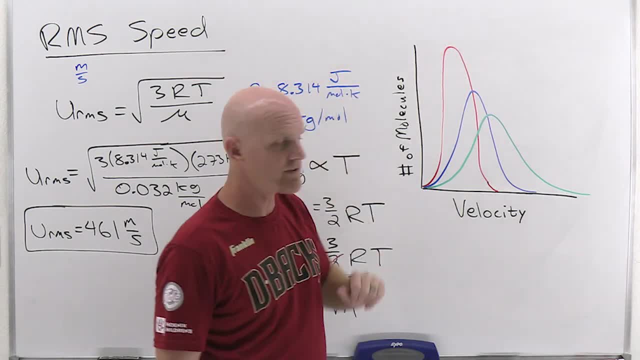 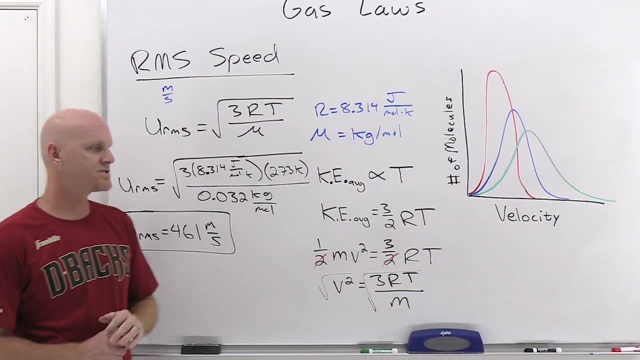 And obviously your average would be, you know, right, somewhere up towards the top here, and stuff like that. Life is good. So well then, what are these other two graphs? Well, they're one of two things. You can look at this Maxwell distribution of speeds, either as a function of speed or